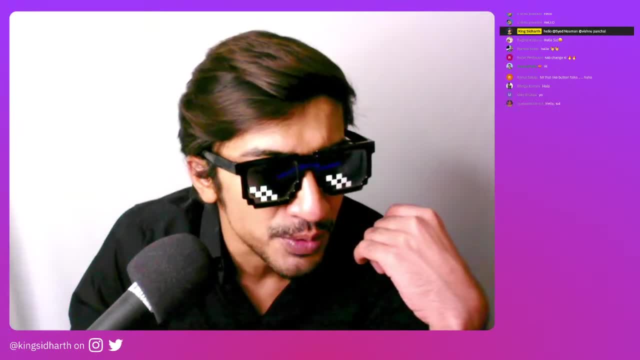 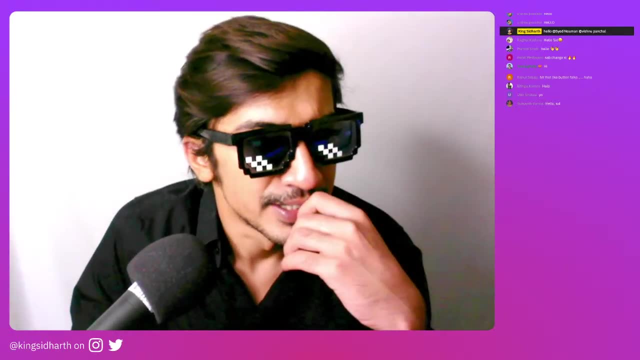 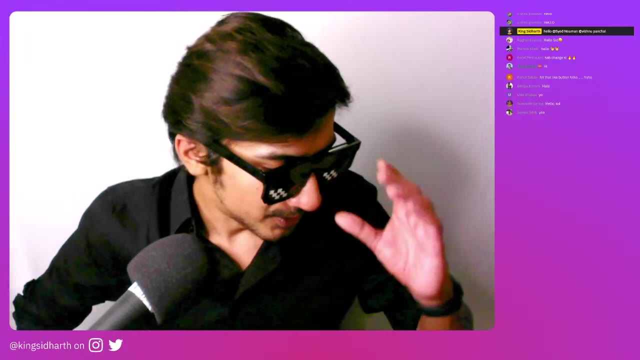 What do I even have? Let me adjust my screen a little so I look a tiny bit better for all of you. Looking better has never hurt. anyone Has it now. Don't mind the darkness behind. I fried my LED, So here we are. 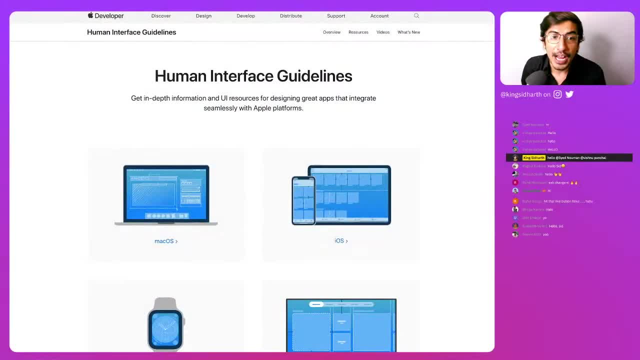 With fried LEDs, and we're looking at Apple's human interface guidelines. If you don't know where to find this web page, just look Google for human interface guidelines and click the first link. It's that simple And let's get started. So, those of you who've been following the series, 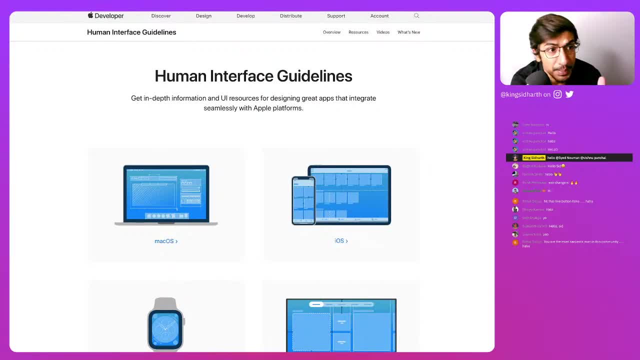 you would know that we spoke about design system basics. You know what a design system is beyond a component library, how it evolved historically speaking. Then we looked at Google's material design guidelines And we saw what kind of documentation they had. I also see Birgu joining in. 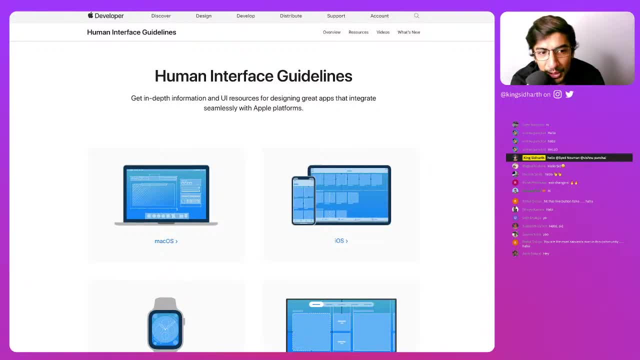 Udachakya is here. Hello, Samant is here, Savik is here And Amit is also here. Good to see you. You are the most sarcastic man in the community. Oh, you have no idea the levels my sarcasm goes to. 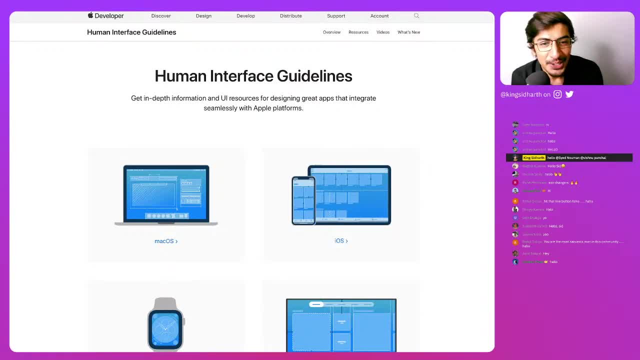 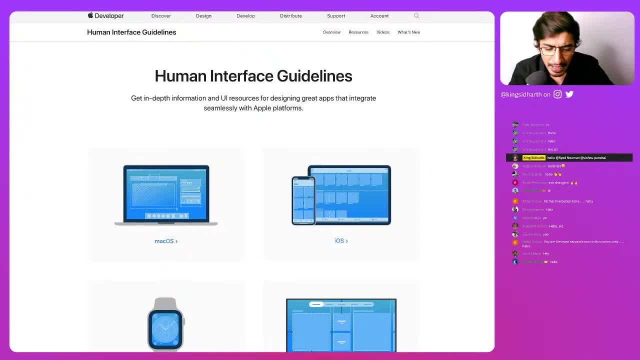 Okay, This topic? Yeah, So Apple has had design sensibilities since beyond. Google woke up to design. To those who are born recently and not in the 90s, that might come as a shocker, Like what Google was not as great at design always. 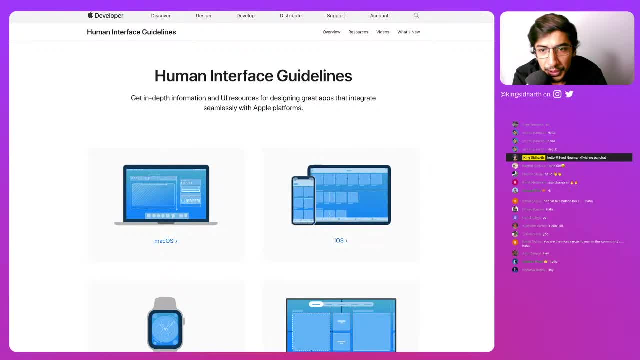 No, they weren't, And Apple's tradition of human interface guidelines and keeping them simple and legible goes long back. In fact, when we go through these guidelines, you will see they are also, you know, written for human beings. However, we'll not find what we found in material design. 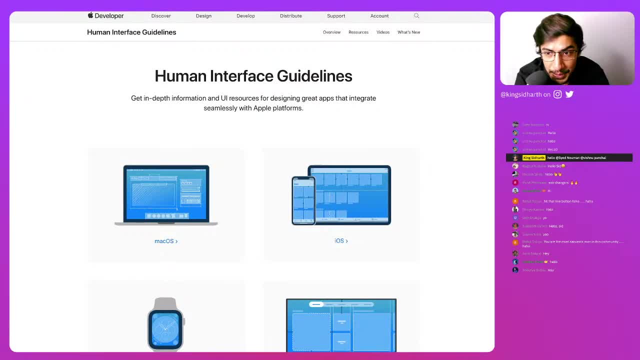 which was a huge component library. right Along with the systematic pieces Here we will find some OS level, some systemic pieces like tab bar, OS bar, this kind of thing, navigation et cetera. that are standard. But Apple's way of leading the design in their community is with example. 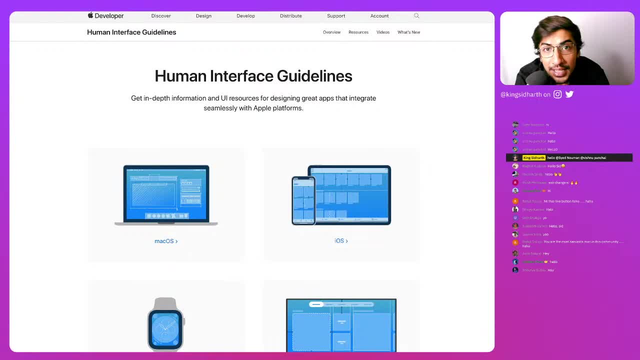 In fact, with every iOS release, the redesigns often they end up doing to the OS and to their native apps, And their native apps often defines you know what kind of guidelines will come into picture, And then designers interpret that into their work. 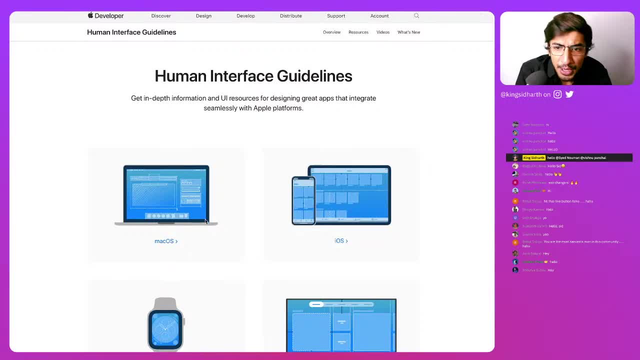 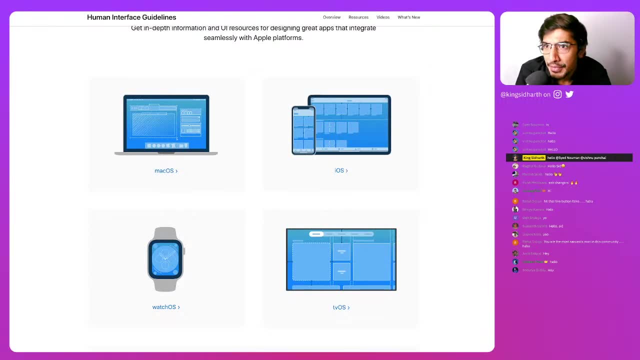 So the guidelines, as we expect, exist for macOS. Recently we saw Big Sur with those new kind of things coming on. I can show you some, because I have Big Sur right here If I go to the control center. this is what that looks like, right? 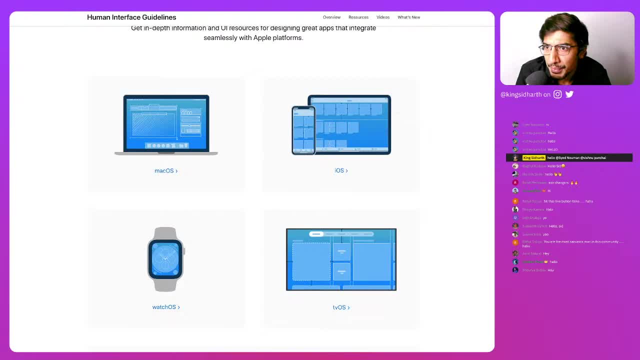 You can see in this top corner like this, all of that kind of stuff happens, And there's iOS, There's watchOS, There's tvOS And in future there might be more. Today we'll look at largely iOS, maybe a little bit of watchOS and macOS as well. 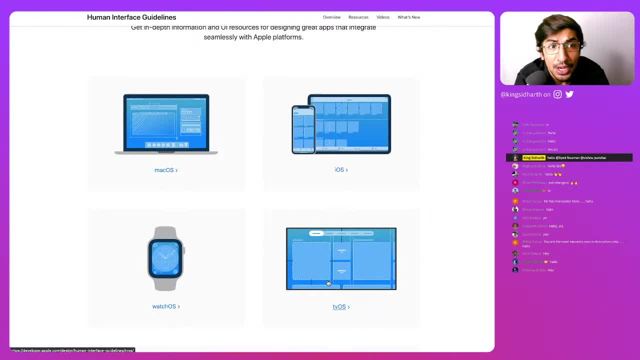 if we get time, And that is what we're going to talk about that. how does Apple talk about? how does Apple look at these systems And remember these guidelines were written back in the day and they've been. the underlying system was written back in the day when design system as an idea did not exist. 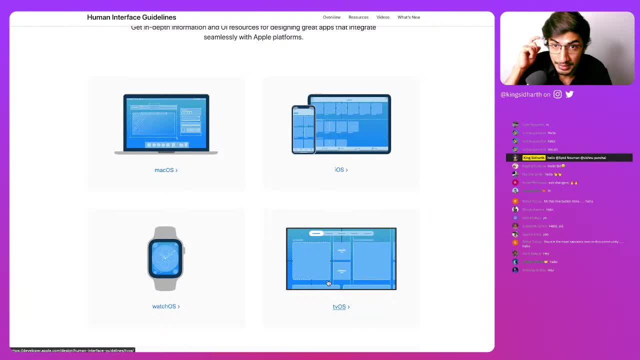 So many things here are what we will recognize as design system today, But these predate that And therefore Apple continues that tradition the way it culturally and with community and with example tries to lead. you know the design language, which is surprising you. 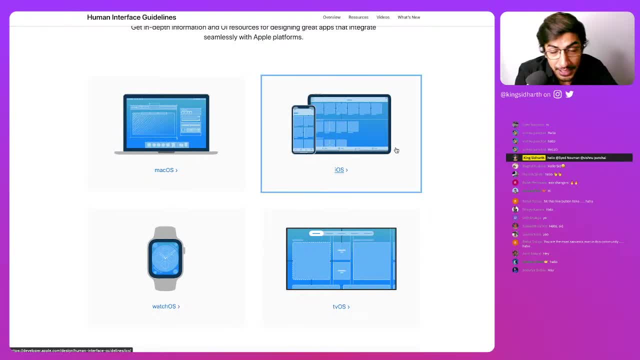 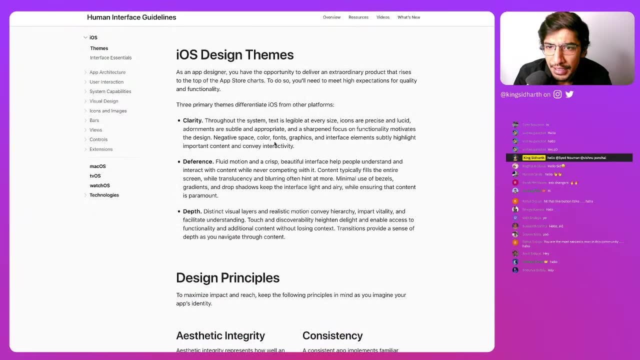 know like one would think that Apple would have even stricter things, But let's take a look. So we click on iOS and we are greeted by this page and we say iOS design themes And they talk about the philosophy behind. This is very important. 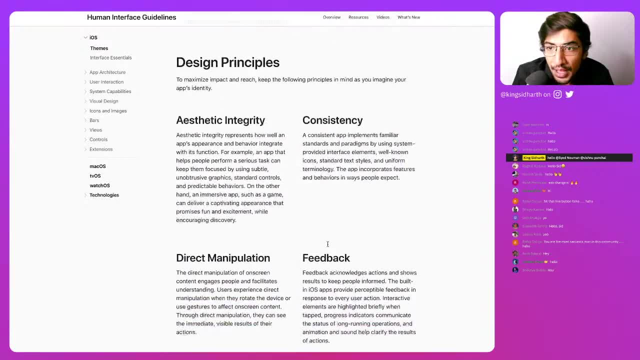 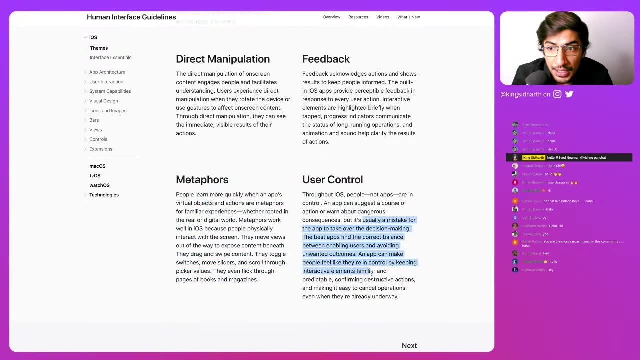 Of course, like we see that philosophy is the basis of all systems. And then they talk about some other things that are important to them: how to use metaphors which a lot of people recognize from the skeuomorphic era, how to think about user control. 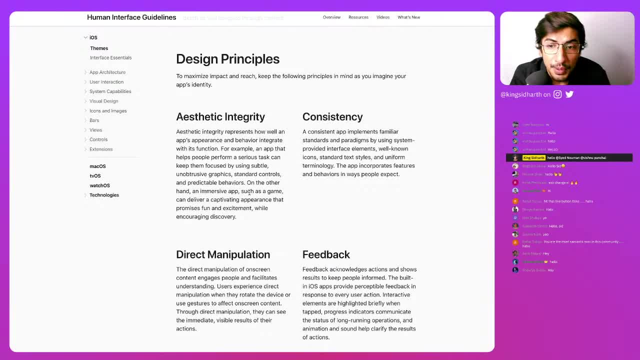 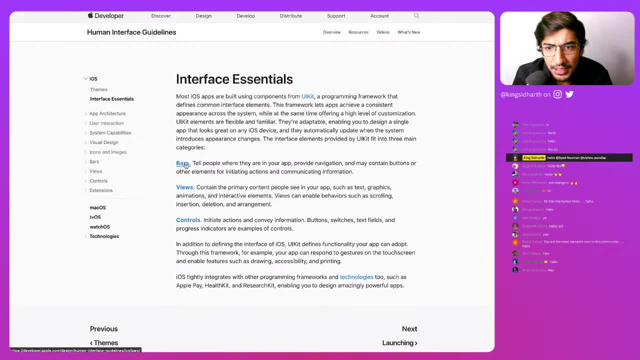 feedback, direct manipulation, which is a big part of, you know, UI, touch interface that they talk about. So let's go to interface as an essential They talk about. there are three kind of interface essentials they talk about. They are bars that create iOS. 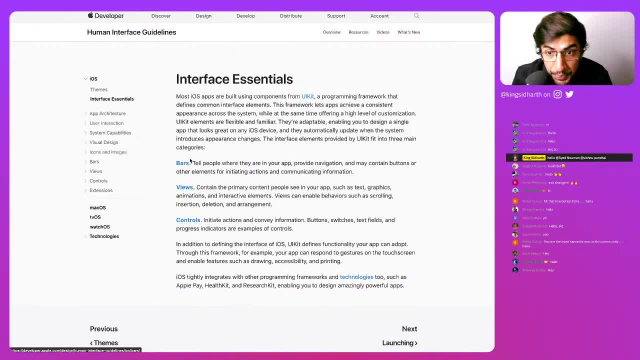 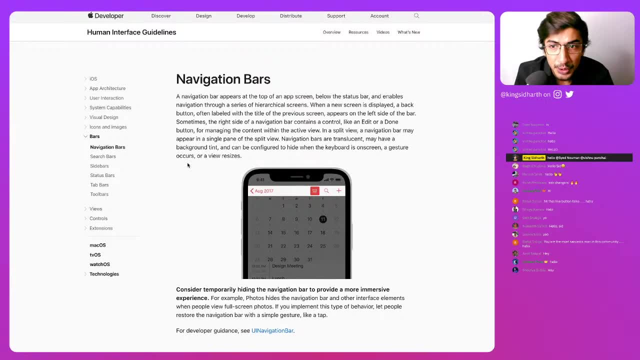 They have views that you know make iOS apps and their controls. Let's look at bars Bars. This is one of the most fascinating ones. The obvious one is a navigation bar which is manipulated heavily throughout. one is the navigation space. 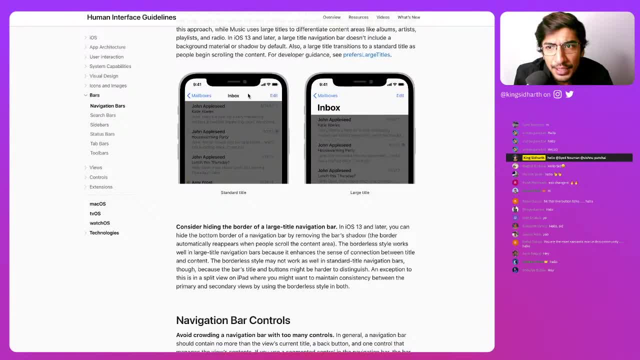 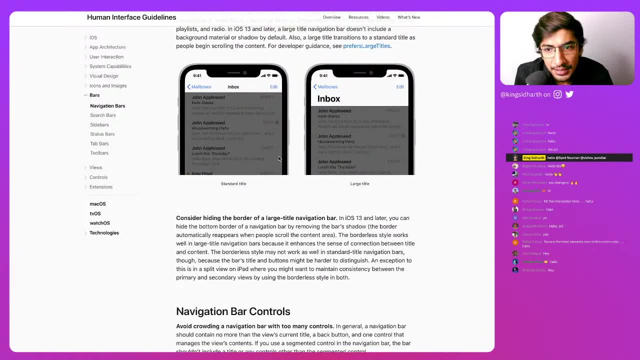 And you can see how it takes you inward forward. You can have like: uh, this we see, uh, you know, larger small title. We see the same example with material design guidelines as well, but here it's done slightly. 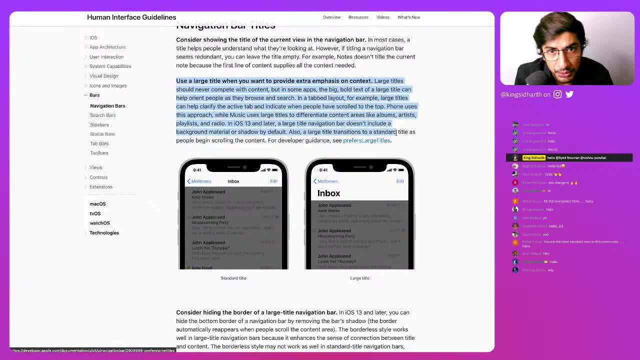 differently And they also talk about you know when to use it, while material design may not talk about as much. So this is one of the key, important differences between how Apple treats guidelines And how Google treats guidelines. Google will give you an option, maybe some hints, but 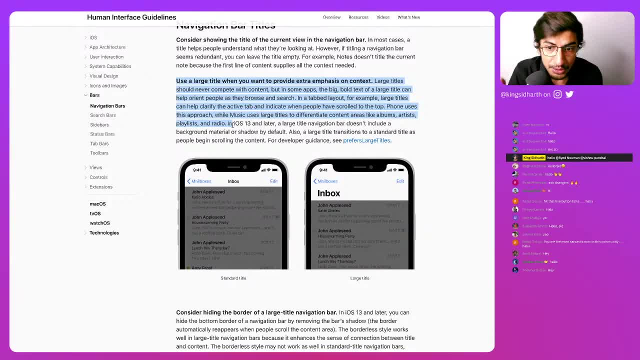 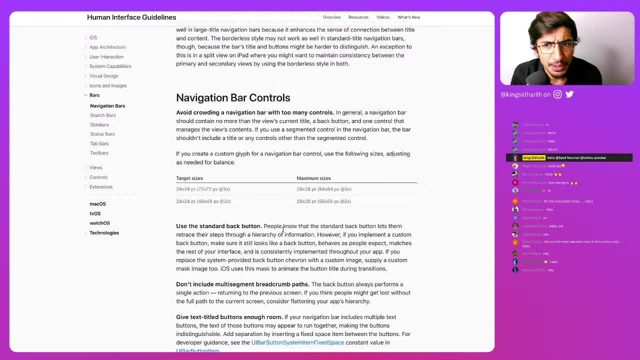 apple will start with the point, the problem, the kind of things you're trying to do for us, and then talk about what are the, what are the options. So consider hiding, border, et cetera, and they will go to that kind of nuances. 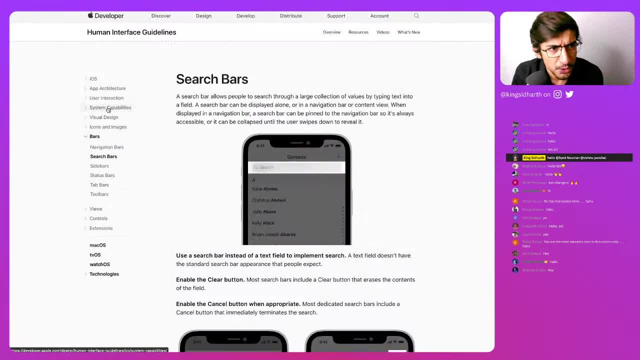 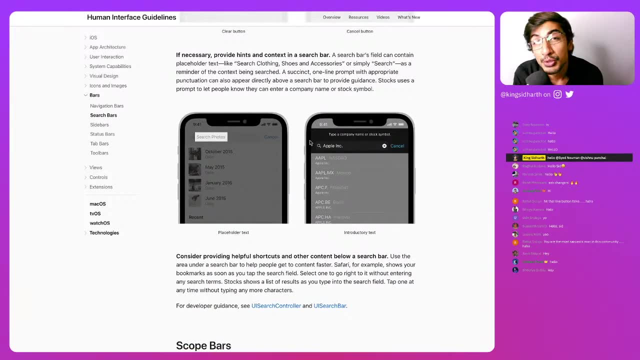 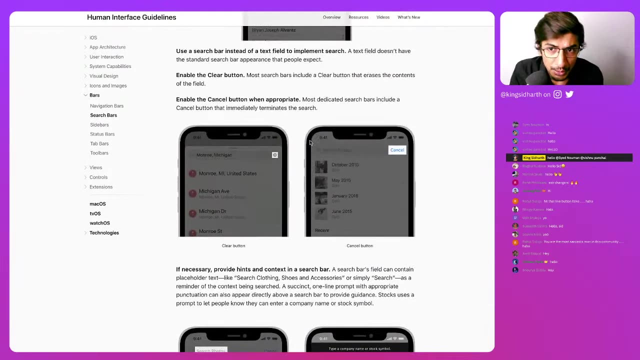 Uh, then they talk about controllers. Then what if the bar turned into search, which is a very special treatment in iOS? Those of you using iOS will recognize this as a standard search bar which is used across iOS. Like websites, whether I mean on web, there can be different implementation, whether on a browser. 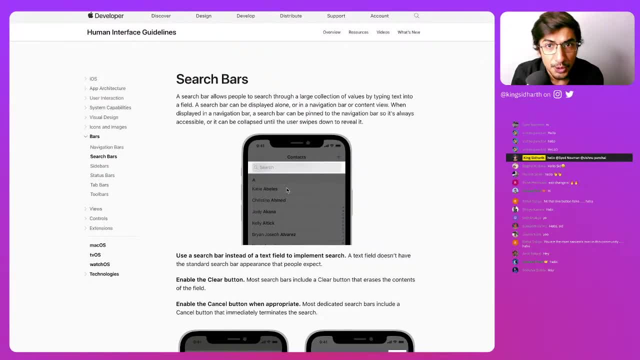 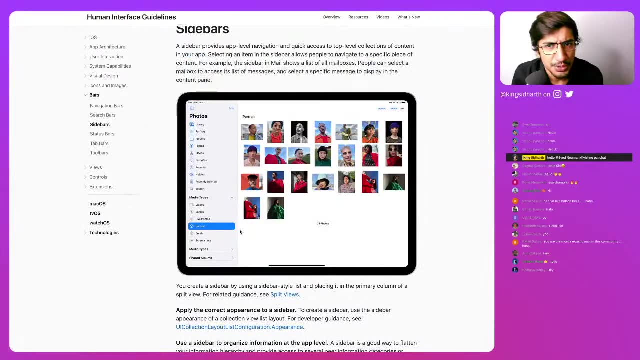 using the browser main navigation bar or any other app, the search works the same across the apps. Then we come to sidebars. when you open in sidebar what the you know, which is weird, but if you think about it, what they're thinking in their terms, I find this slightly weird. 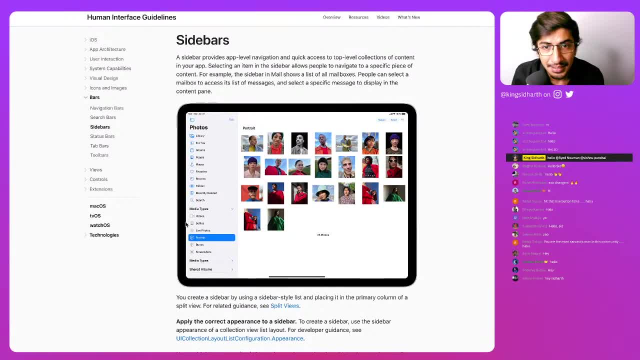 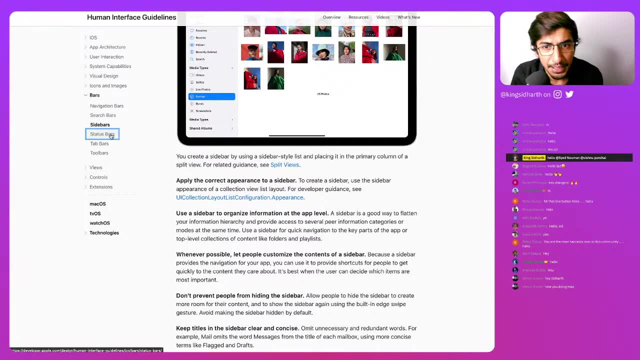 I think sidebar could have been completely different thing, But they look at it as a stacked, you know as stacked bars. And this is the header right, the highlighted header that we saw earlier. And the same thing goes for status bar. that status bar is on the top. 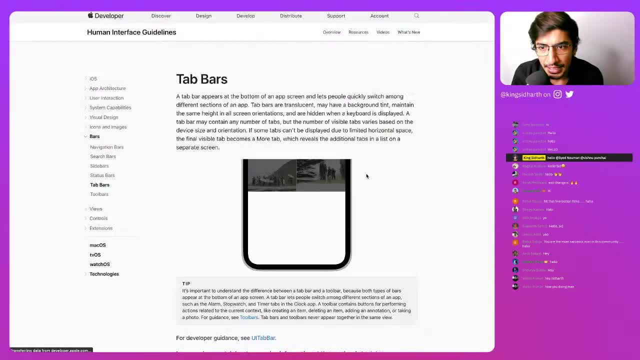 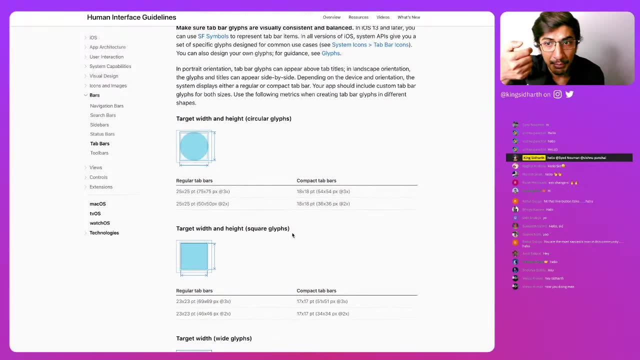 And this is a standard pattern in iOS. then we have tab bars, and tab bars appear at the bottom, like we see on, you know, material as well, And they talk about, like, what should be the target tap with when you have circular things, square or rectangles, etc. And the last but not least, 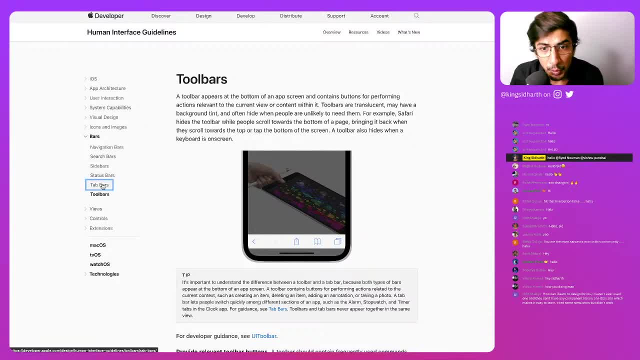 is the toolbar. Now, what is the difference between tab bar and toolbar? Now, tab bar can be is the usually the primary navigation in an application. For example, this is for photos And a toolbar appears in specific context. So toolbar on this page may be different from. 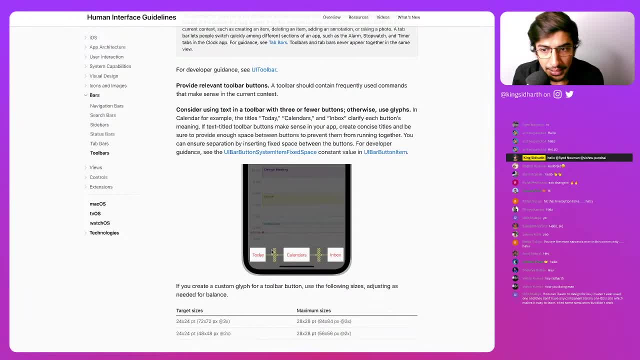 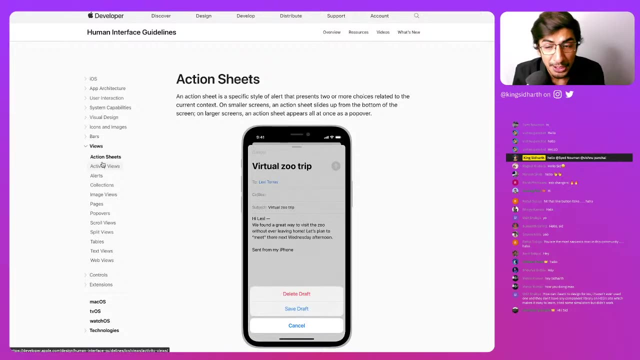 toolbar on another page. It's specific to the tool on that area, So you can see how toolbar changes for calendar. Alright, so now we have spoken about bars. The next thing they talk about is views. Views is the massive thing that covers everything. Some of the special views they talk about is an. 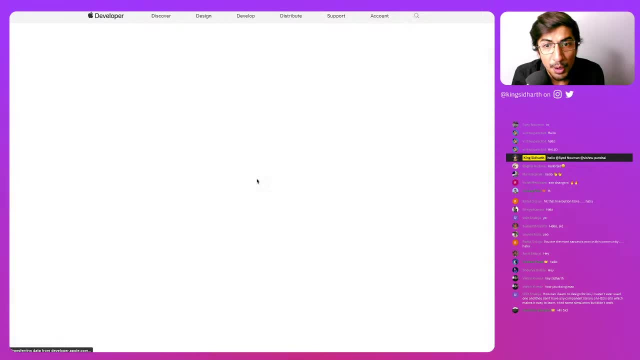 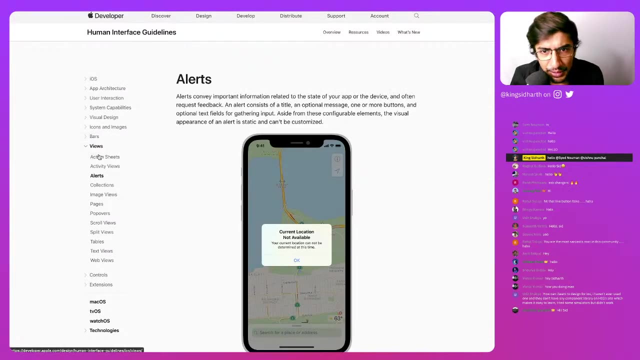 action sheet, which opens specific kind of actions. Then they talk about activity views, which are the share sheet right. Then they talk about alerts, which is nothing but you know a pop up like you have a functional pop up. then they talk about collection, which can be grid or list, And 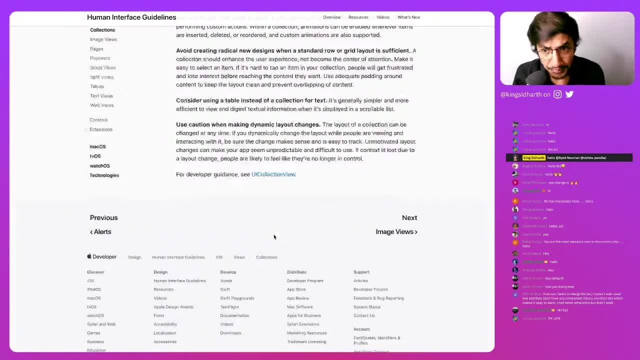 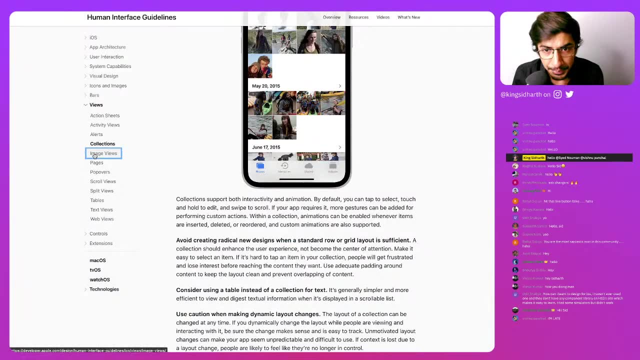 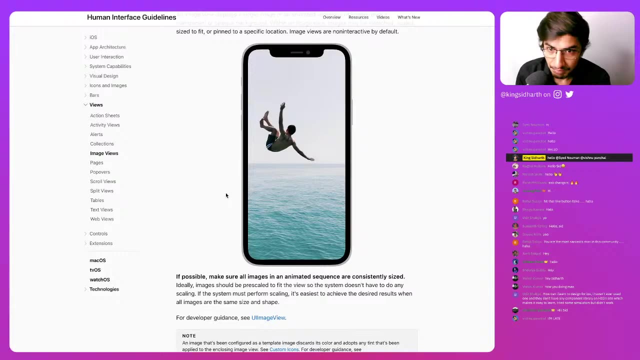 then talk- actually let's talk- about collections. This is, again this, highly linked to the developer options that are provided. So that is, you can see how tightly knit Apple's user interface guidelines are to the development tools, Full image views, which are, you know. 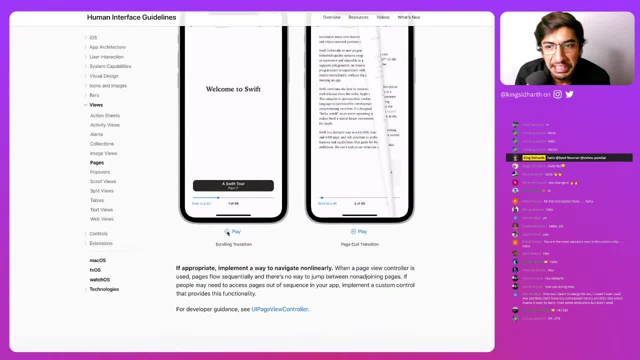 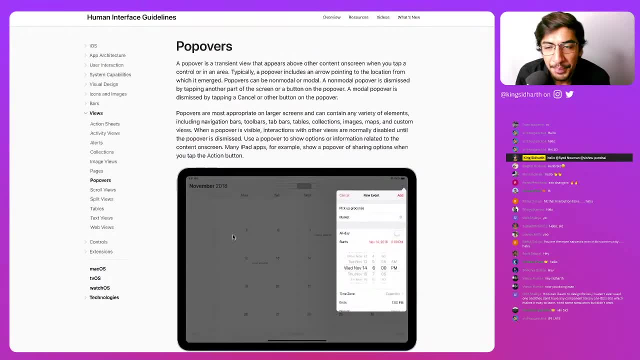 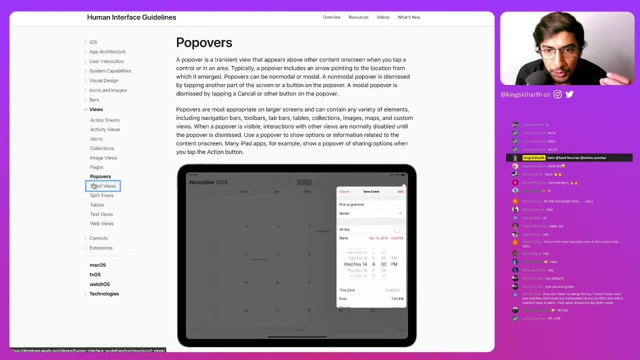 I don't know if it warrants something like that And pages which essentially can cover anything and everything you want. Then popovers, which are usually- you know, they are- available on iOS- sorry, smaller devices as well, like iPhones as well, but usually, more often used on tablets. 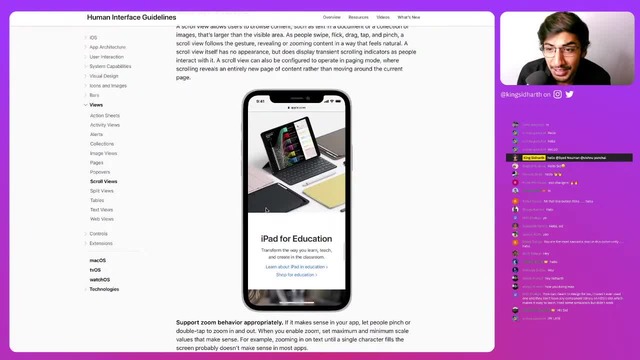 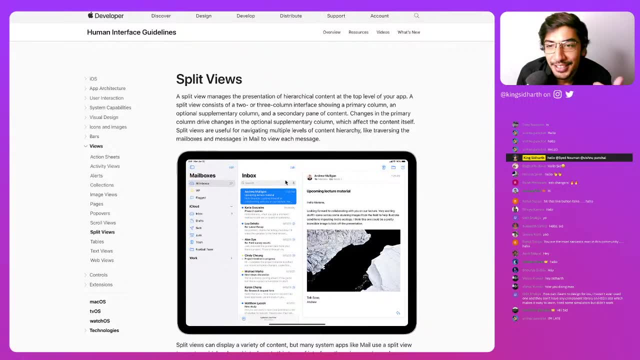 Scroll view again contains every and everything Like scroll view. you can imagine like everything is scroll view, right? That is where it becomes. it starts to give you more liberty, right? That is why you saw more innovation from designers in these areas as well. 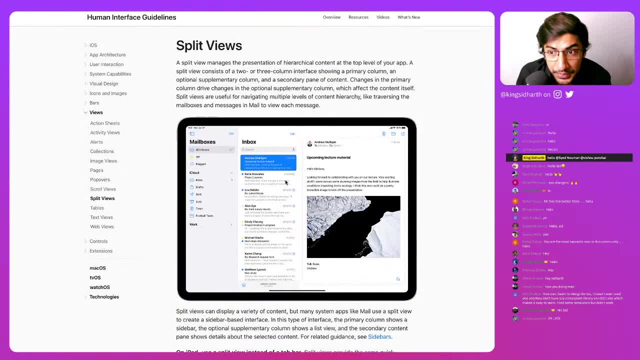 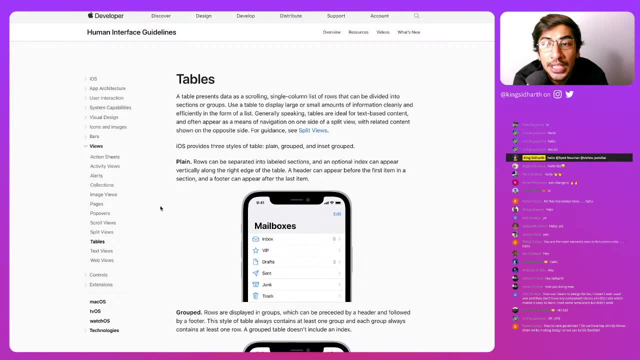 Then split views which are more popular on again on the tablets, the iPads, And then we see tables. Tables are critical. Now I want to stop on tables, because tables is perhaps the most simplest and the most complex one, which has done the most heavy lifting since time immemorial. 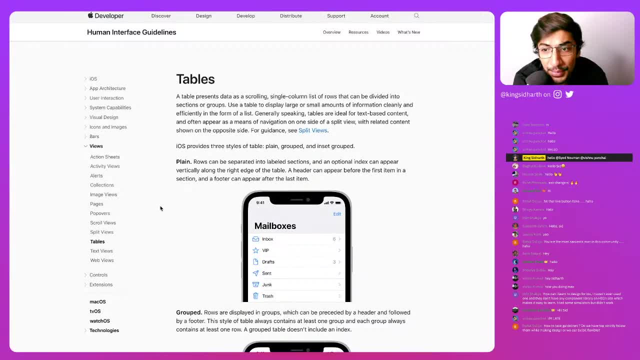 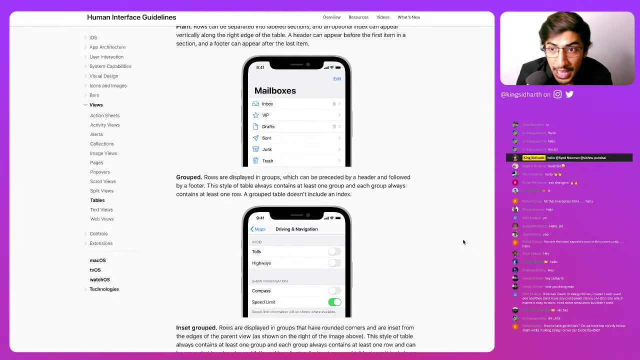 Now, many of us would just recognize this as a pattern we use in setting this ECRA, but this used to be the primary way. most applications worked early on, So you have nothing but a list which can have you know, a list of all the things that you need to do in order to be able to use it. 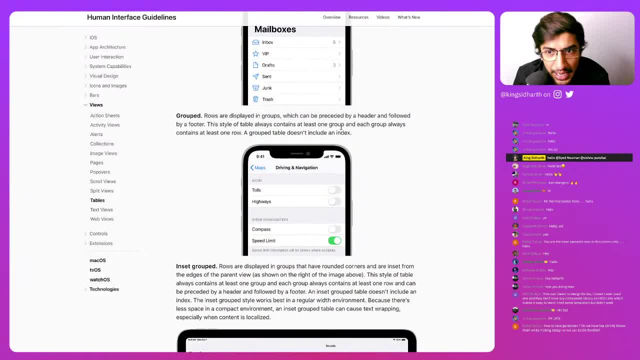 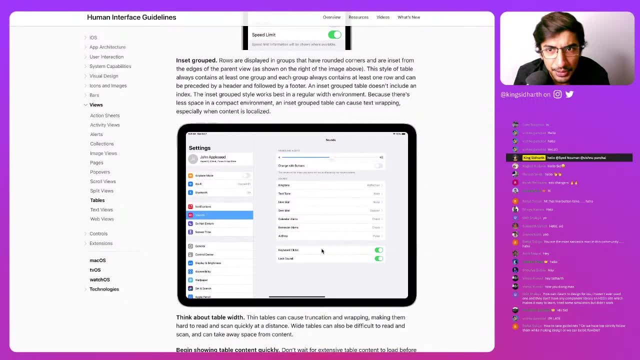 You can have you know icons on the side and some kind of like you know numbers on the side which you can again turn to actions and this turns into that sort of list. You can create groups. Then these groups can become nested. sorry, these groups can be within other sort. 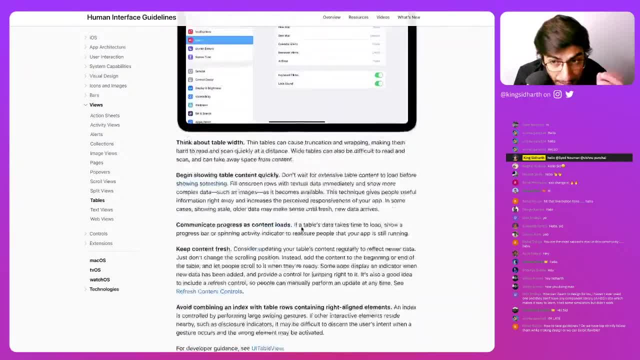 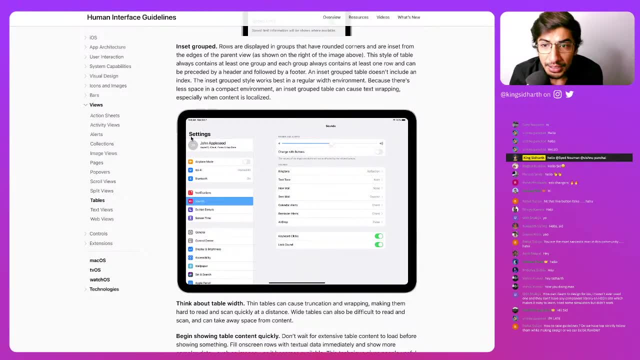 of groups. So you have complex UI states happening, like the settings thing on the- what do you call that iPad? Now, the same thing. if I was to show you, let me actually show you. let me quickly pull up QuickTime and I'll show you the same thing. 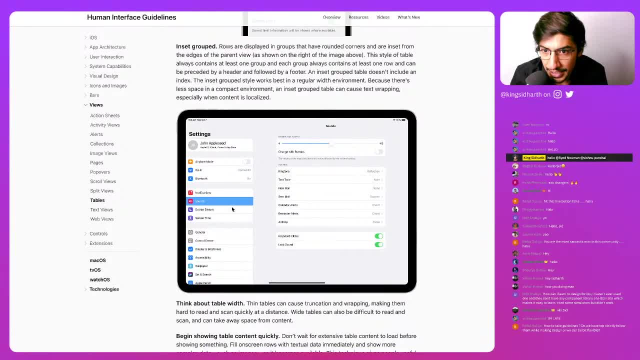 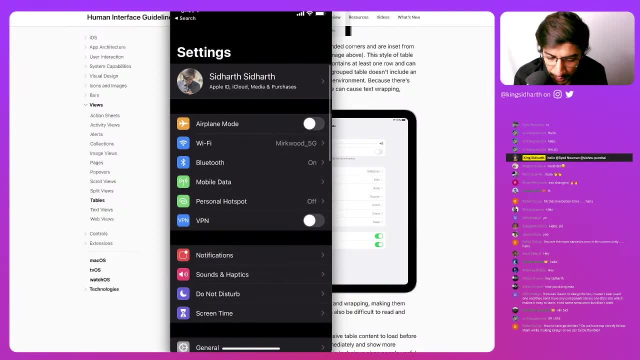 on iOS, right On this thing, it happens like this: right, You can access it side by side, but on iOS, the same pattern is extended with this sort of thing where I go inside and I go back right. So the same interface. now, if you look at, these are two tables. right, This is a table view. 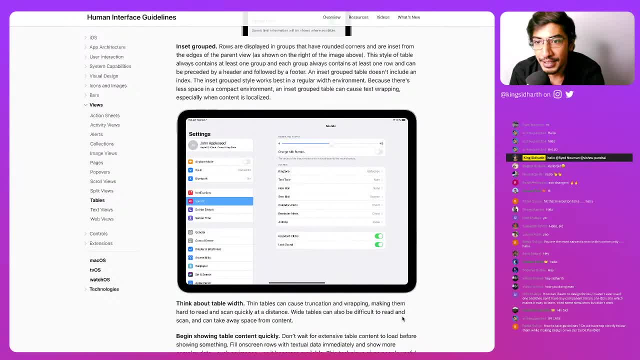 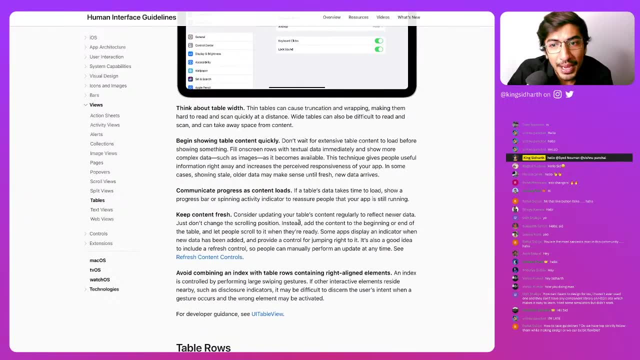 and this is a table view, and these two table view are then combined here to create a different view, which you can also call this a split table view. So this is how they combine very basic elements like legit. these combinations- split view of two tables- is how they start creating. 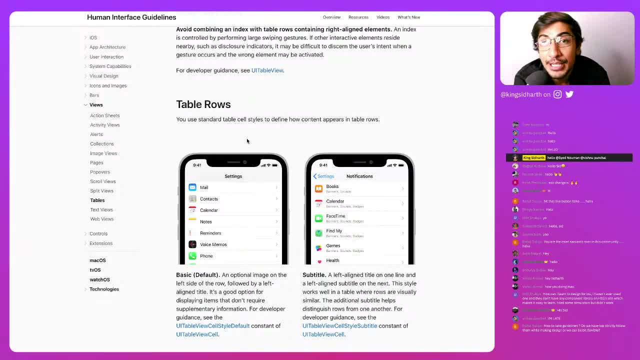 complex UI. So Apple interface guidelines are really simple because they really focus on the core aspects, the core components which deliver over and over and over again. And this is why I think this is crazy, because these are also examples of table rows and table views. So if we 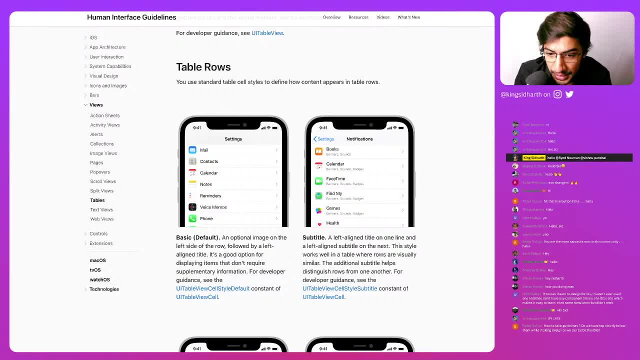 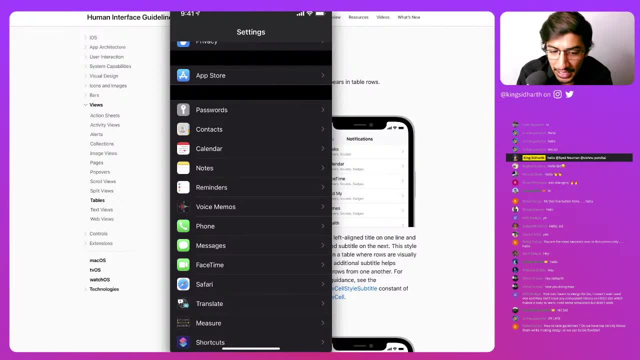 again going back to settings. if I was to go to settings, where is my iOS? and if I go to settings and if I scroll down, you will see some apps here Which, again, like, is another table view. And if you go into one of these things, let's say calendar. 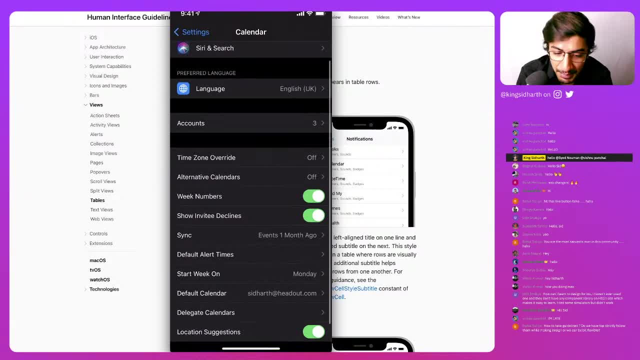 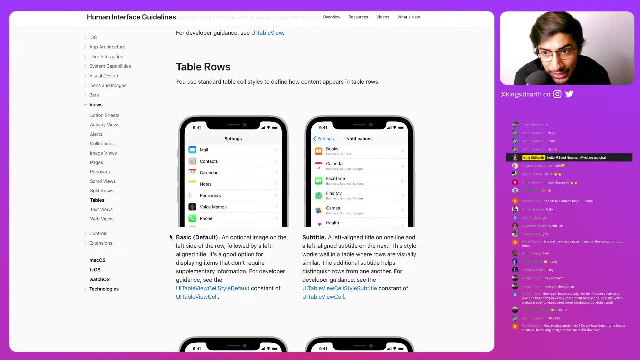 you can see permissions, which is another table view, And table views inside table views, inside table views. the thing continues And you can actually cover a vast number of contexts just like this, And this was one of the revolutionary things that were fascinating about you know. 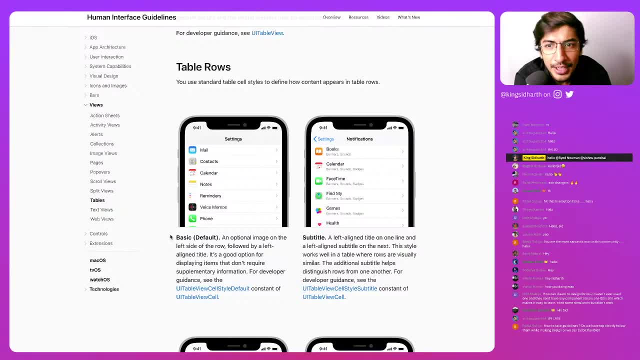 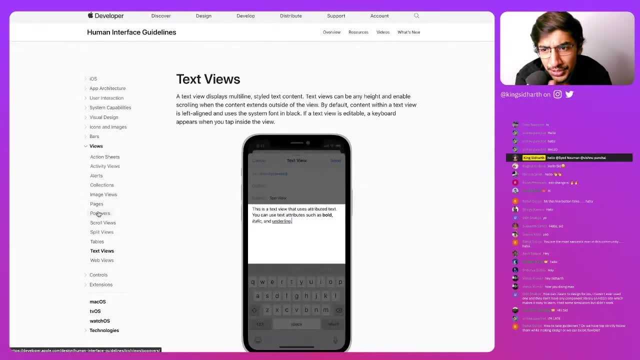 Apple's user interface Now to all of us. it's obvious, but this was the simplicity of UI when it came back in the day. Now we're going to cover text view. Text view is simple, but when you're inputting text and web views are specifically for iOS apps. 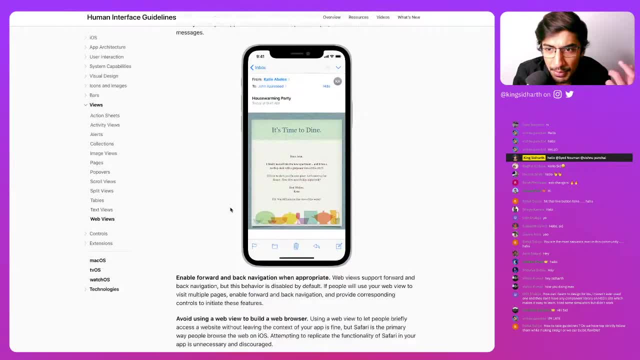 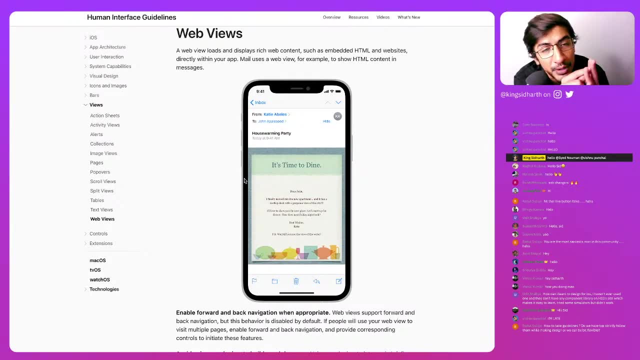 where you actually pull up, you know a website or. this is not a great example of how people use web view, But often when you click on an Instagram, if you go to my Instagram profile and you click on the YouTube link, it'll open a sheet. that's also a web view, a Safari web view. So that covers. 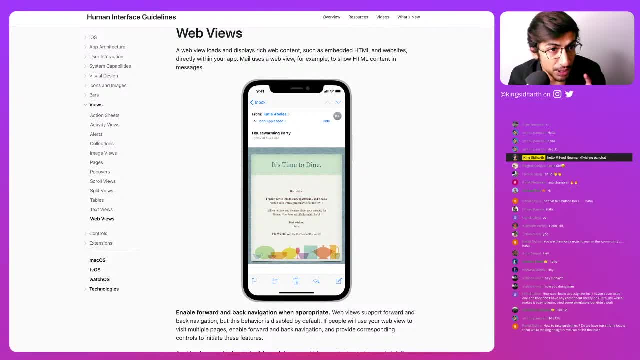 views as we can. as you can imagine, it covers everything. We're going to come to controls in a second, But first we're going to look at chat. All right, what is chat saying? Amit is here, Oh. 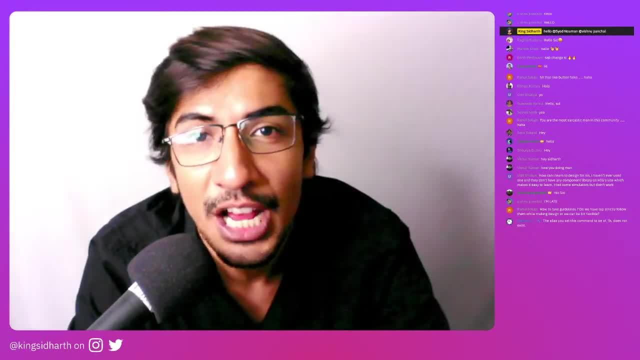 all right, Shoray is here. Good to see you. I'm doing good, Vishal, How are you doing What it says? how can I learn to design for iOS? I haven't ever used one and they don't have any. 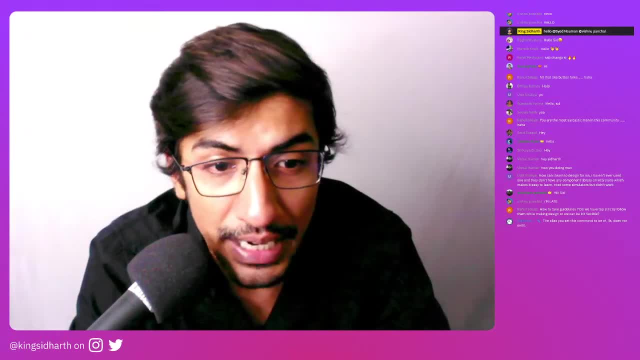 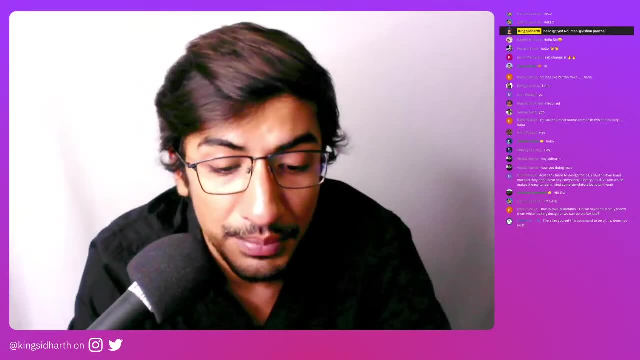 good component library on HIG site which makes it easy to learn. tried some simulators but it didn't work. Simulator is not a great way because the touch is very important part of iOS. You can- I think they still- produce that iPod touch which is the cheapest iOS device still- I think 10,000. 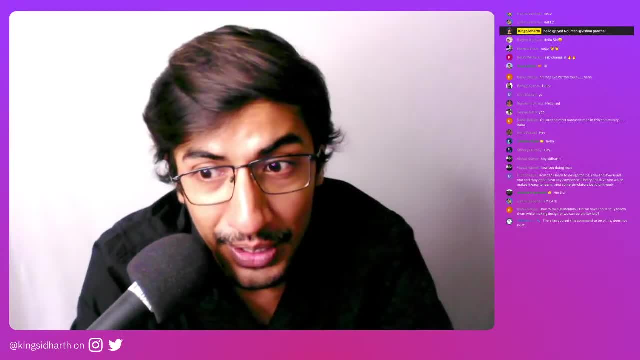 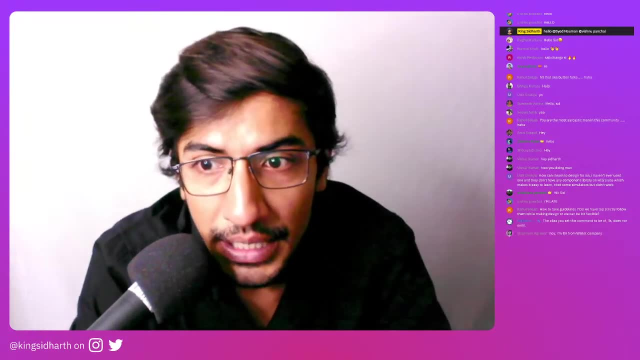 rupees or something you can get that. I don't know if they support the latest iOS or not. you've got to buy that before you buy that, Or you can always get a secondhand Apple device with it. But that touch part is important. An Apple device is just not about the software. you've got to also 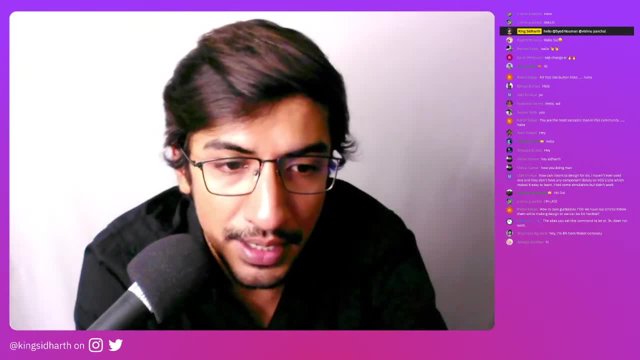 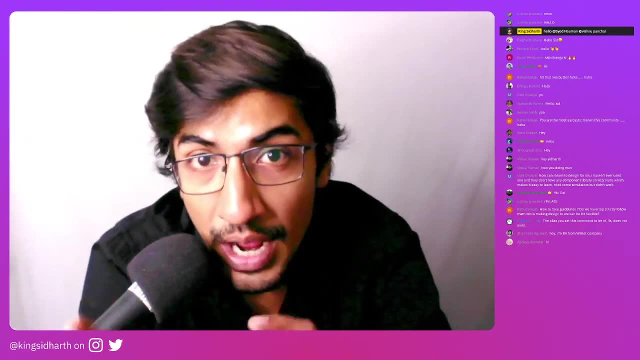 got to know the hardware to be able to design for it. So I would highly recommend getting your hands on an iOS device checking out some app, and we're going to look at some examples. That is exactly what I covered. This is not how they think about design. They don't think. giving you 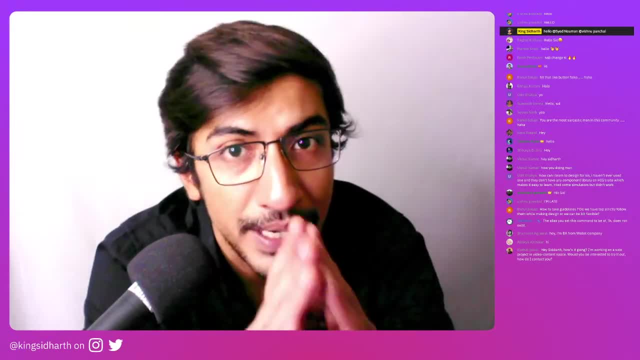 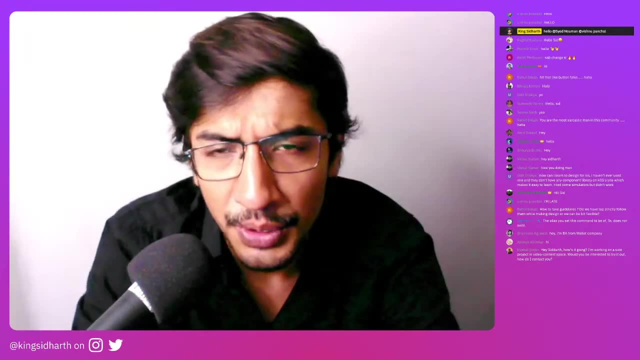 a massive list of components is going to work. They talk about what are the basic elements available to you and how they think about it, And then you can think the same way about your applications, And we'll take a look at Apple's best example of their own implementation. 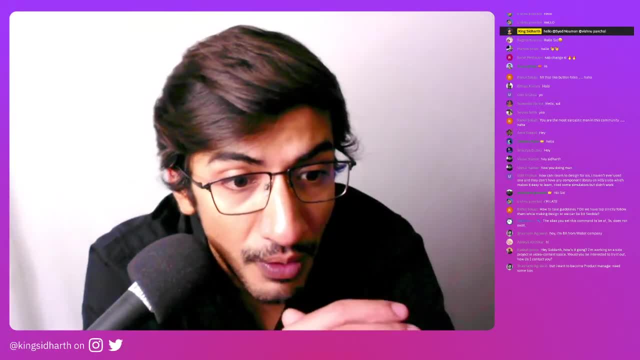 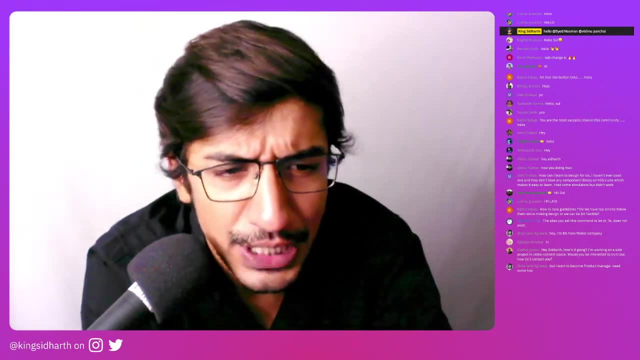 of their own Apple interface guidelines and what it can create. All right, Then we see I'm late, Vishnu, no problem. Shubham says: Hello Sid, Hello Shubham, Good to see you here. Shashank says: Hey, I'm BA from wallet company. All right, Shashank, I'm not sure what I'm to. 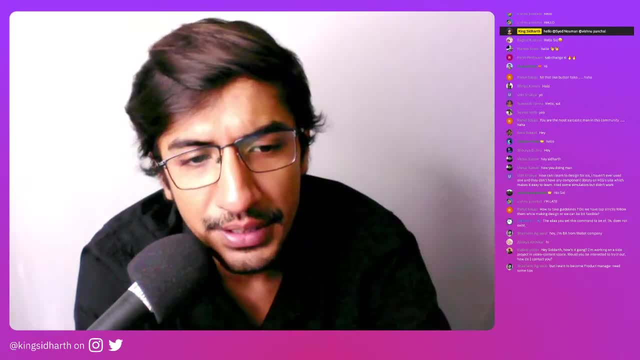 make of that? Ajinkya says Hello, Hello, Ajinkya. Kushal Yadav says: Hey, Siddharth, how's it going? I'm doing a project in video content space. Would you be interested to try it out? How do I contact? 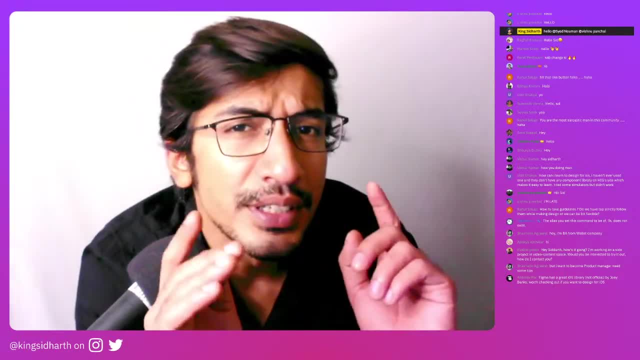 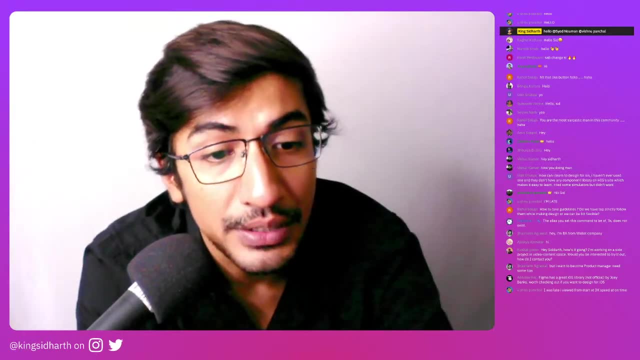 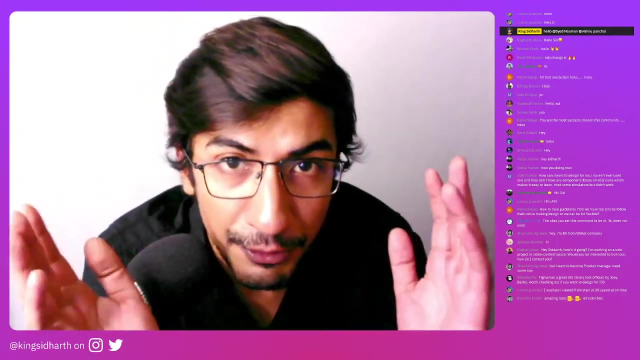 you, Kushal, you can DM me on Instagram or DM me on Twitter. Twitter DMs are less busy than Instagram, So just a growth hack, Quick one to reach out faster. Okay, So the Shashank continues, but I want to become product manager, need some tips? Shashank, check out. I have an entire free course. 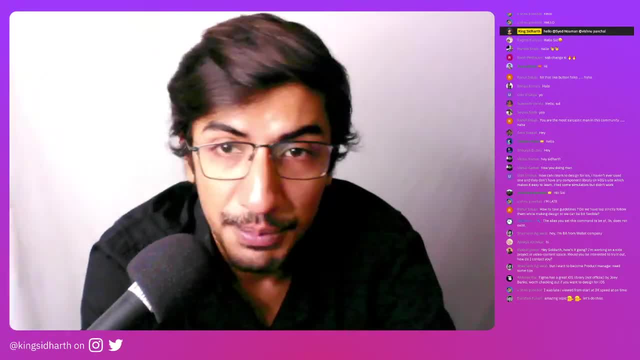 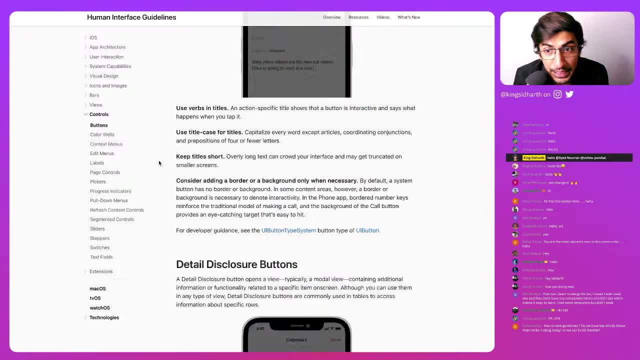 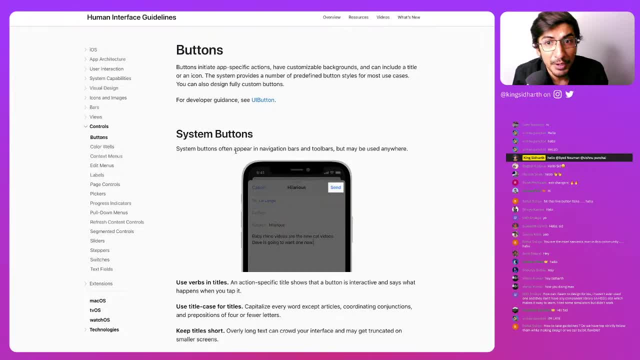 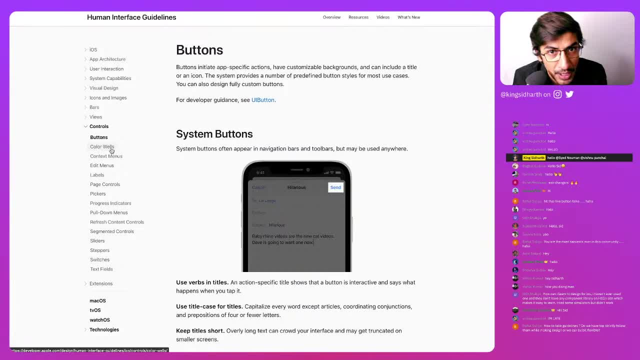 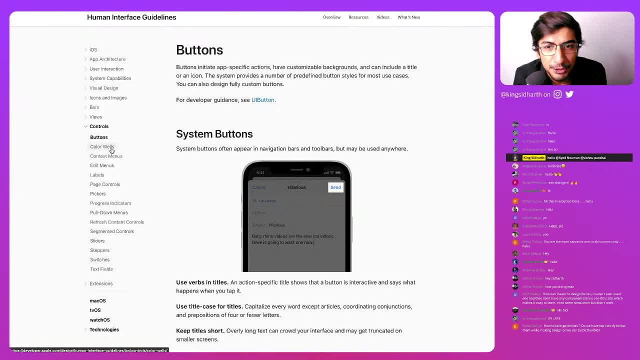 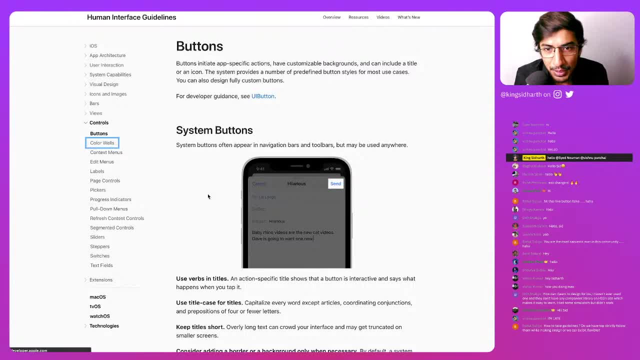 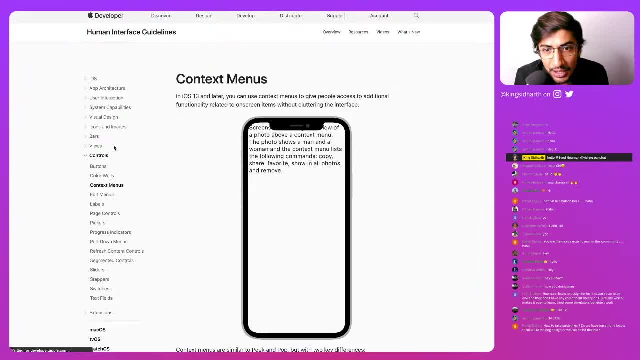 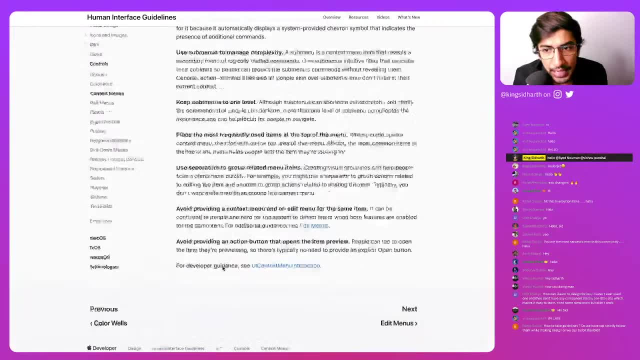 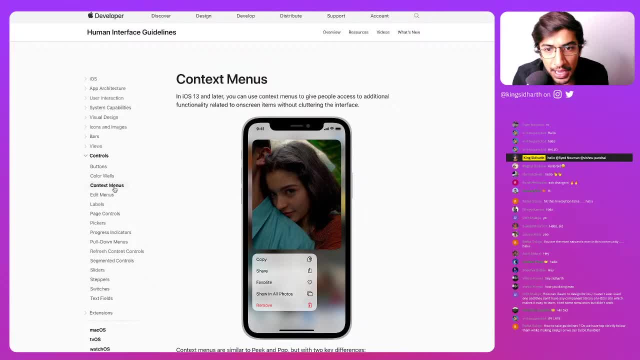 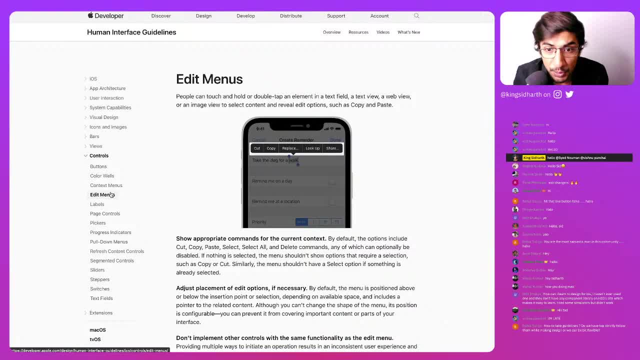 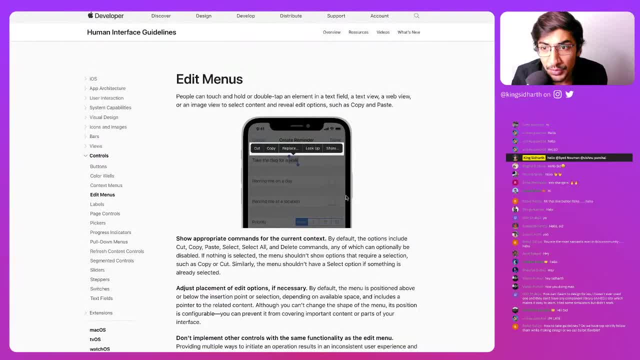 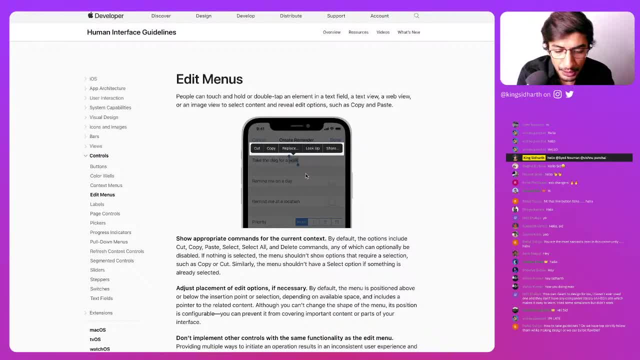 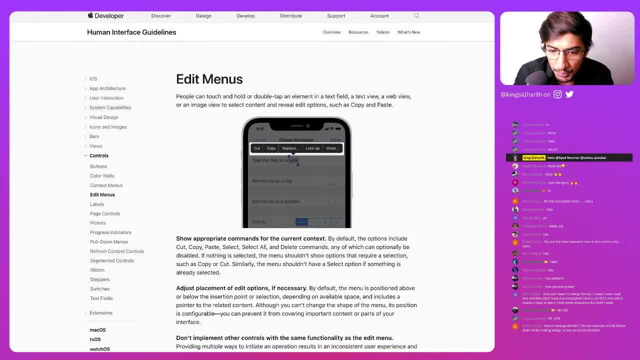 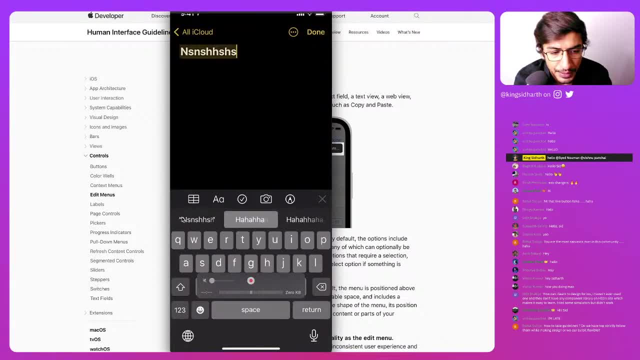 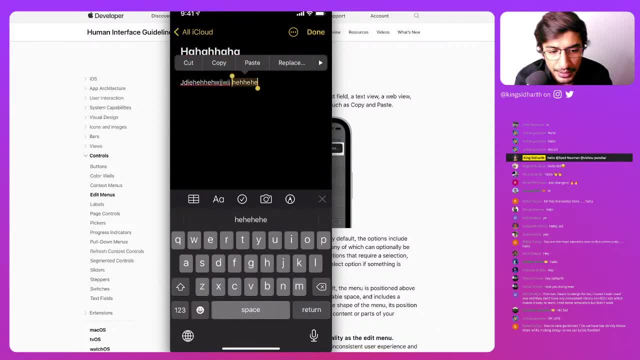 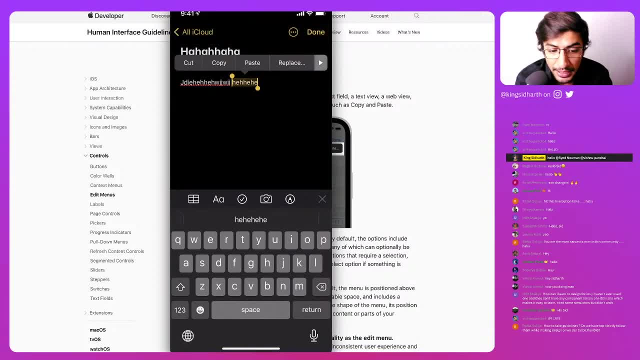 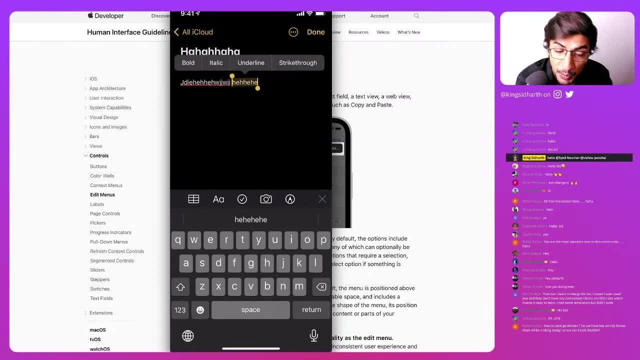 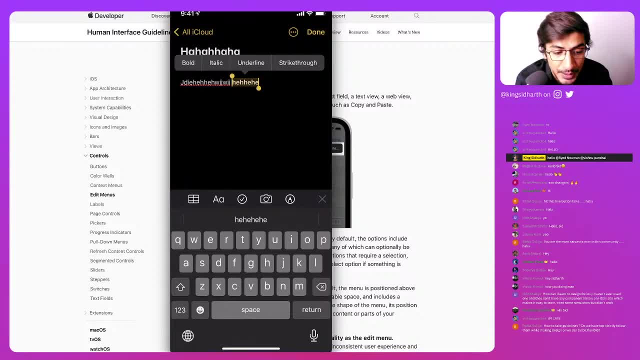 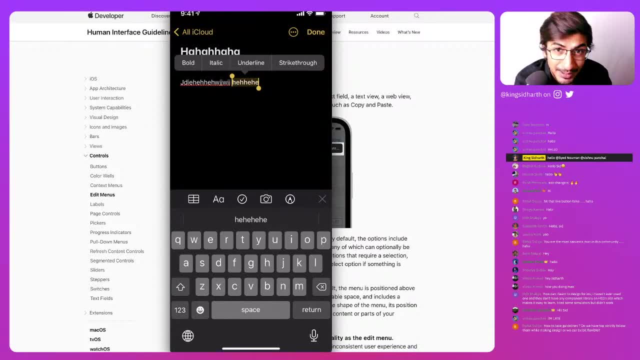 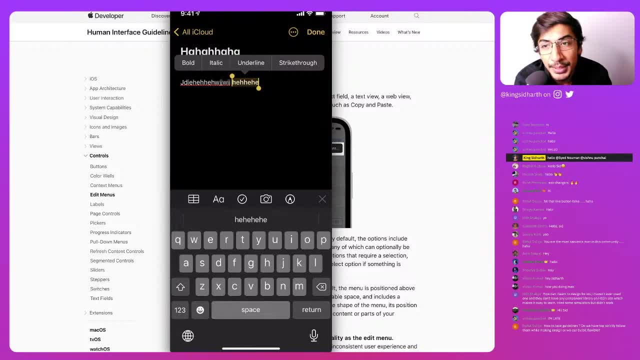 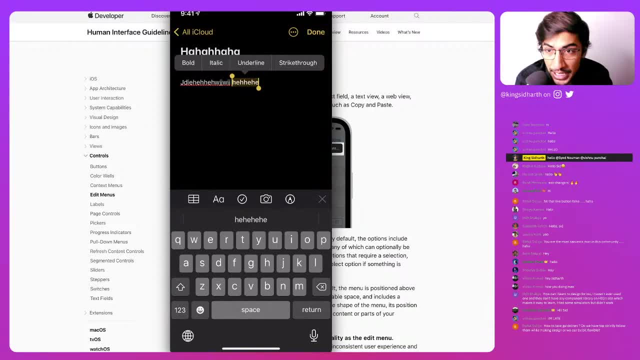 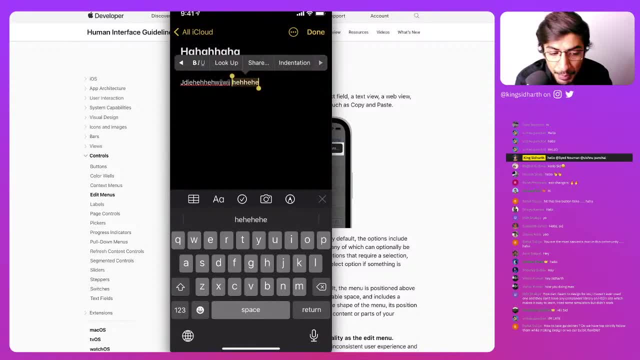 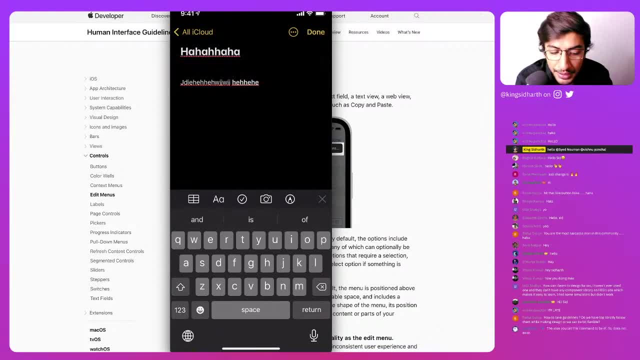 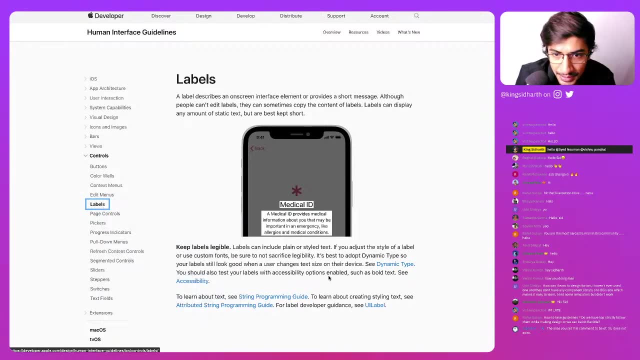 Hello Shubham, Hello Shubham, and you underline it And that's how you do that. So this is another example, right, And we go to labels and labels. I don't know why they're called labels, it's just. 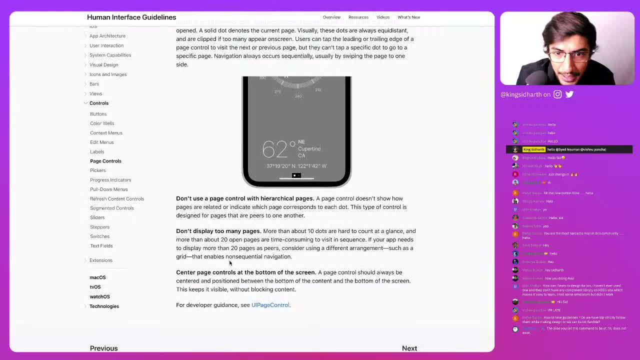 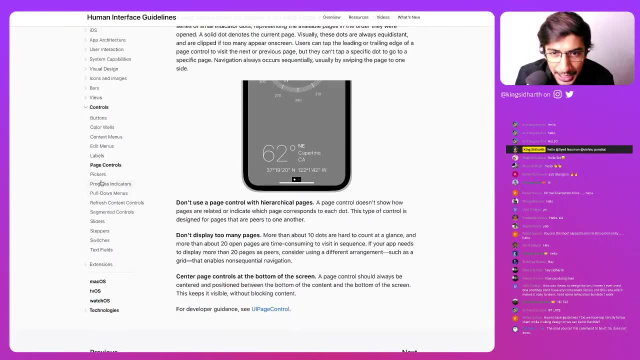 text, but that is how they are called in backend Page controls are these items, these you can go to next and forward this. a lot of weather applications use it and default. iOS also uses it to change swipe button screens because 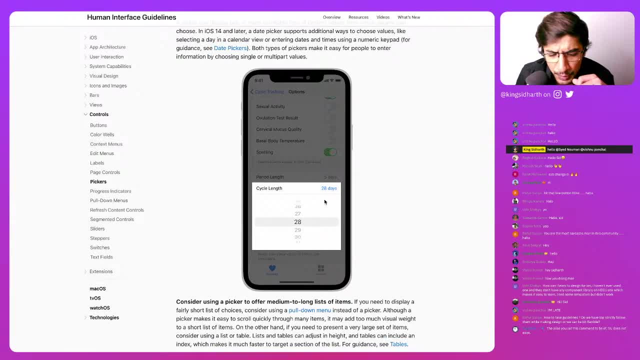 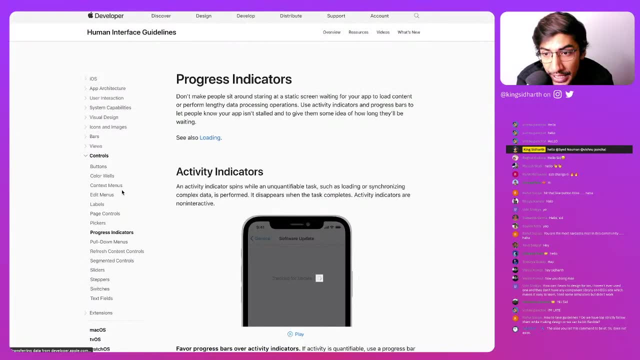 they're essentially select selection drop-downs which appear in this weird way- Alarm clocks, date selection etc. are places you're gonna see it a lot often. Progress indicators are very interesting. they are the basic thing that appear, especially when you swipe down and progress bar appear. Now, both are 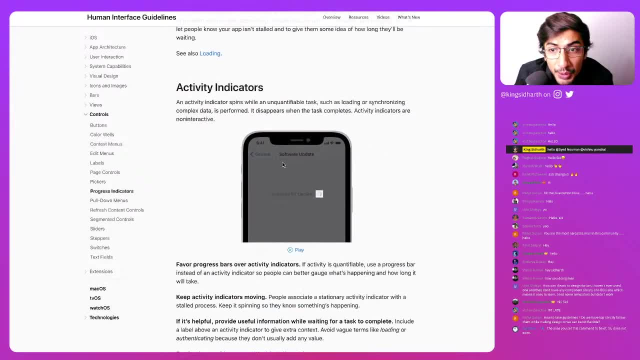 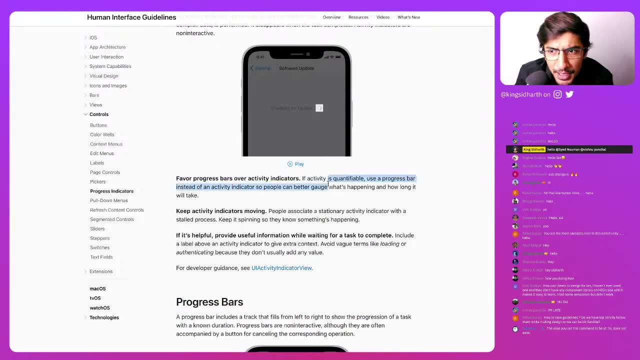 available Apple's recommendation on when to do one over the other? I have not been able to find. I mean, there you go, favor progress bar, let's go through it. let me try to find that answer with you folks again. Favor progress bar over. 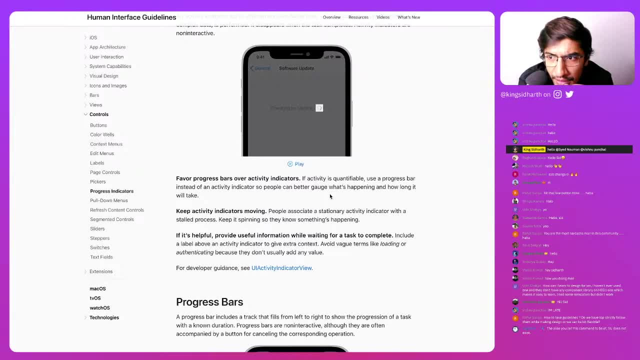 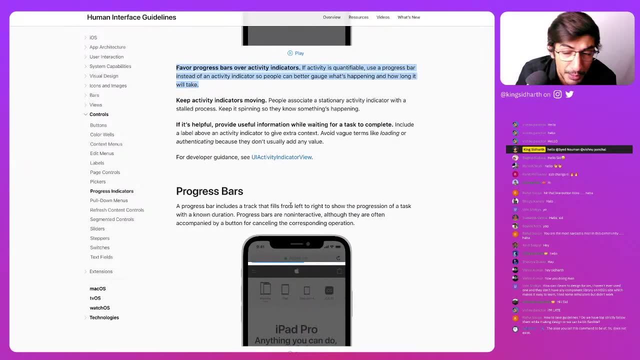 active indicators. okay, so this is what they say, that favor progress bar over activity indicators, but they put active progress bar below The reason they say it. I missed this out last time when I was doing research, but they say the reason they prefer. 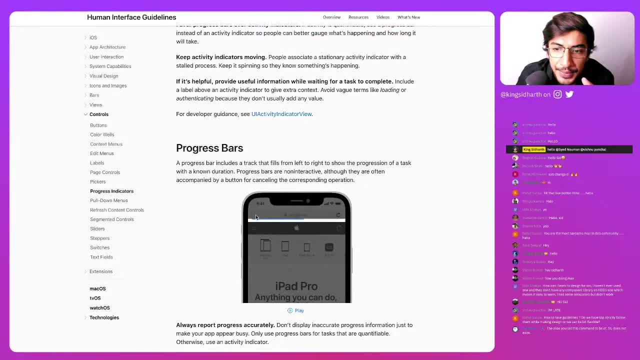 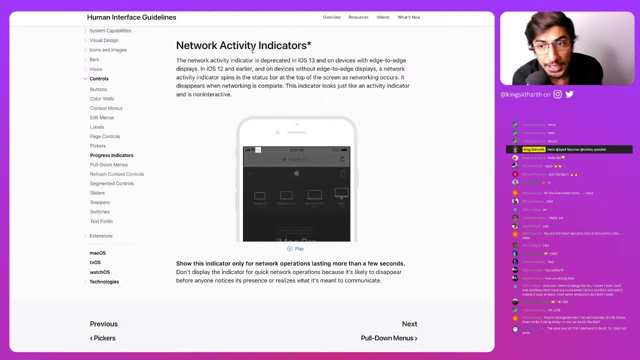 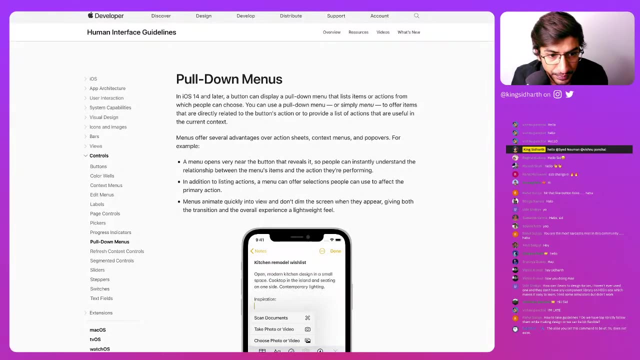 progress bar is because you know how much time is left right in the progress progression of something as well. Network activity indicator is special thing for iOS connectivity where, if the network is not available, you will see the special sign. people will recognize it as well. Alright, the last one we're looking at is: 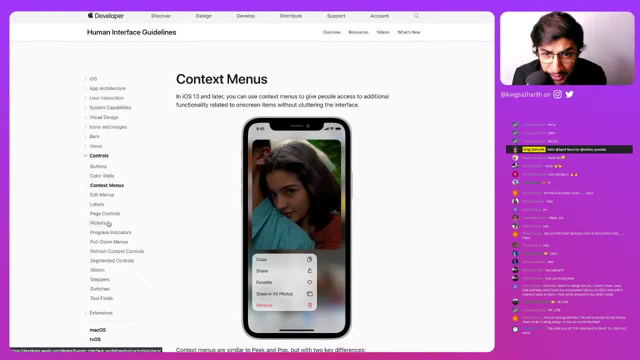 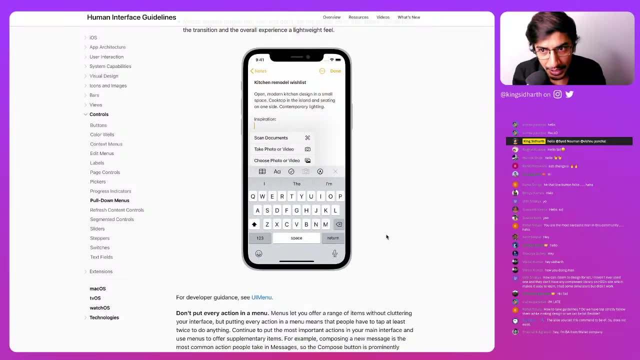 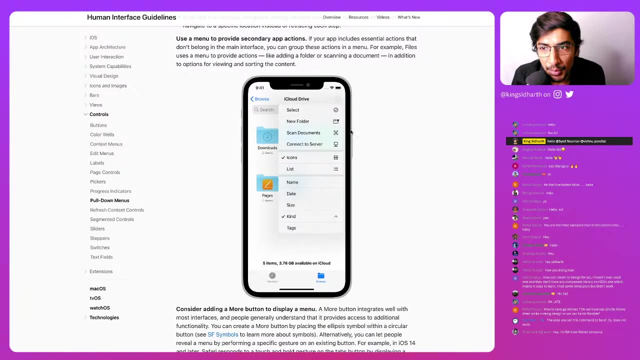 pull-down menu which again I don't understand. why is it different from context menus? but yeah, there we go. they are pull-down menus which have again give you options, which is part of their notes, application and other things as well. The biggest difference I've seen here is probably what they're. 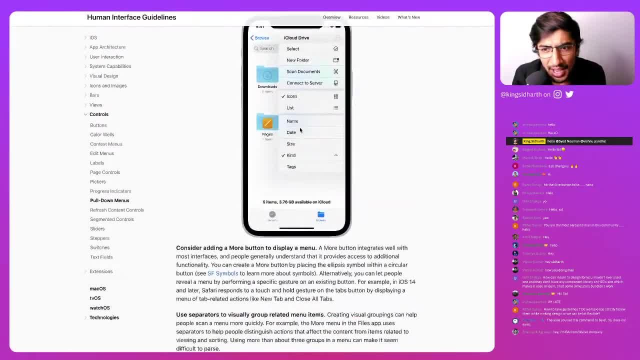 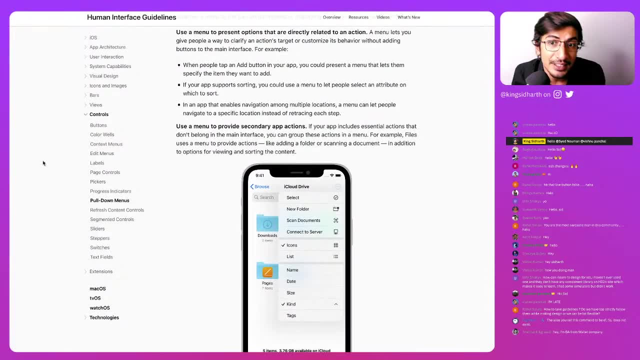 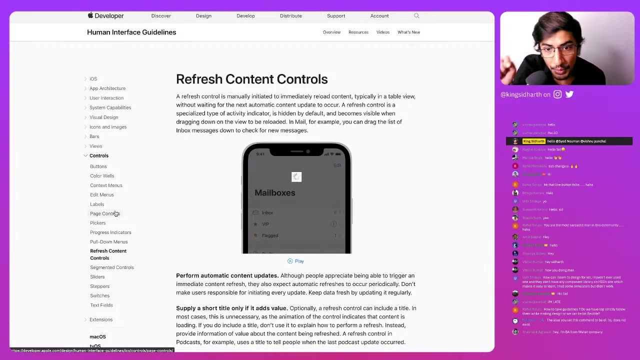 talking about is the inexplicable? no, there is not. I could not find. I think there's a better: just skip menus, edit menus and directly go to pull-out menus. and edit is a special case of that. Refresh content controls is specifically when you pull down long and then this reloads Again. I feel this is. 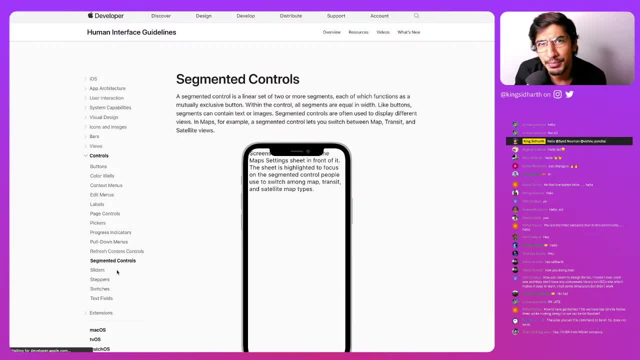 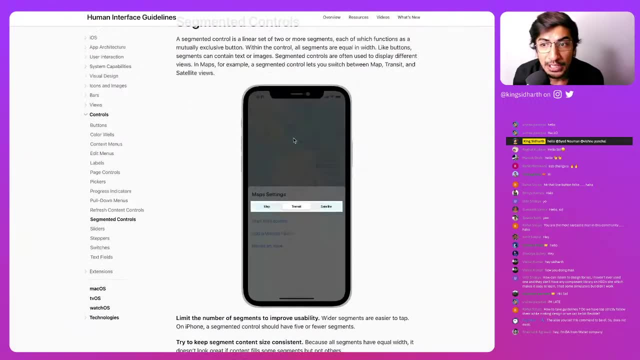 a much better thing to be combined with progress indicator. So information architecture of Apple's interface guideline is questionable. so no doubt people get confused, right? Segment controls, or, as we call them, tabs, Apple reinventing everything as usual. So segment controls are, as we call them, tabs, Apple reinventing everything as usual. 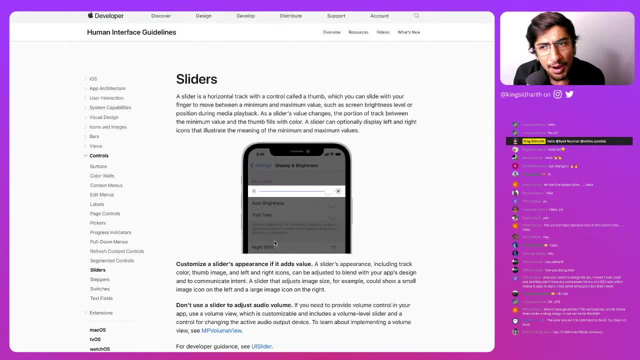 So segment controls are, as we call them, tabs- Apple reinventing everything as usual. So segment controls are, as we call them, tabs- Apple reinventing everything as usual. However, they don't talk about multiple, like double slider and all those examples which are kick-ass, especially used in e-commerce, especially a range. 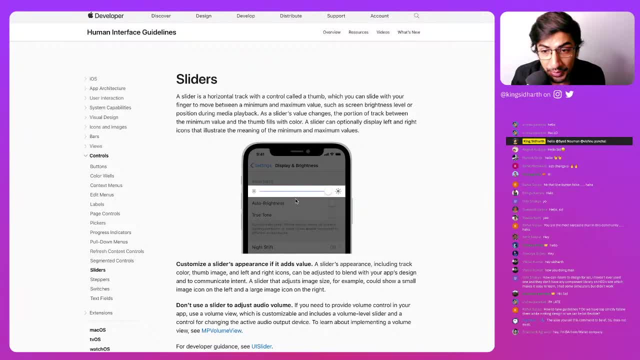 slider from this to this, so those are not covered. if you wanna see some implementation of that, you can check out Myntra app or some other standard applications. Myntra is my favorite one steppers are one up, one down The count. 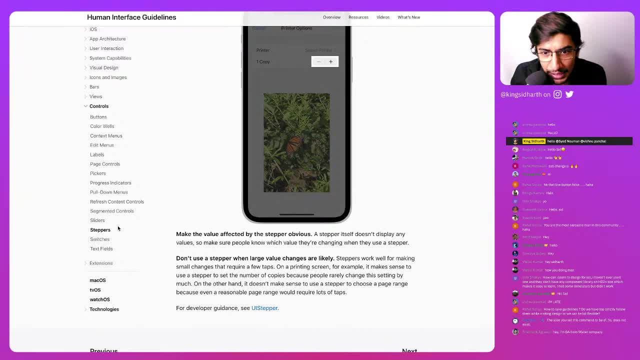 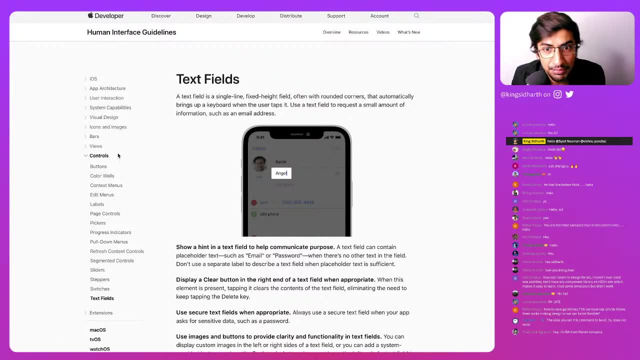 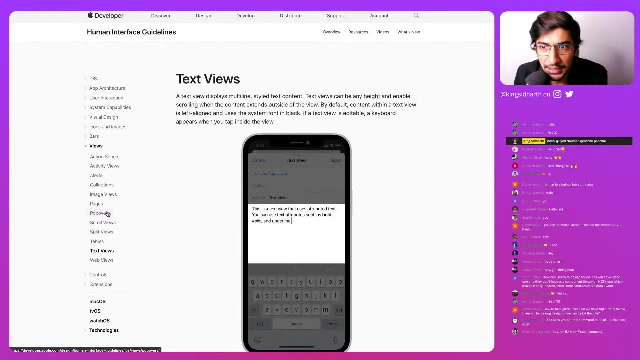 is shown here, which I don't know why they don't show an example of it here. God knows why. Switches are obviously like on off, on off things and text fields are what we said, text fields, which is, I don't know. why. is it different from you? know text views? why don't ask me like don't. 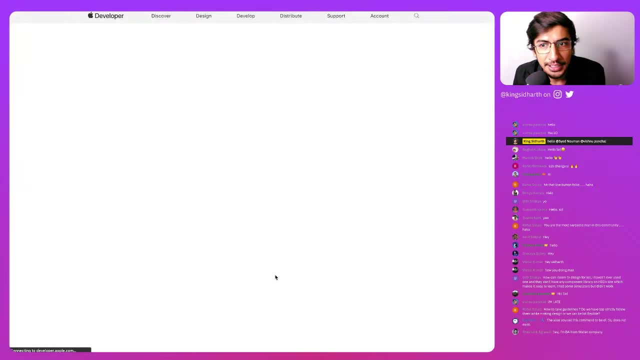 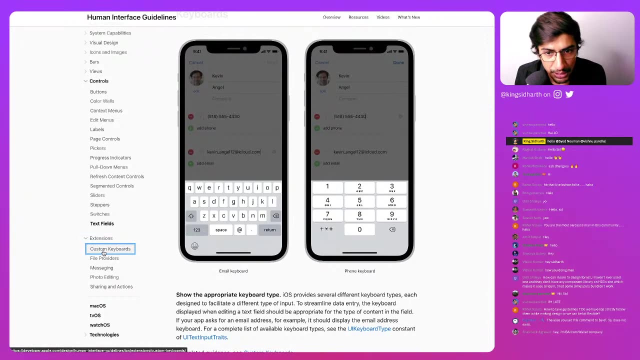 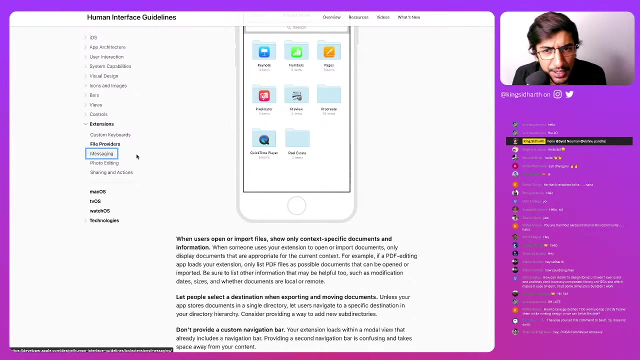 ask me text views and then we go to control and then we see text field like why. and then the last thing is extensions. Apple allies your custom keyboard, as many of you have seen it, or you can have file uploads right where you can pull a file, etc. messaging. I don't know what that is. I've not gone. 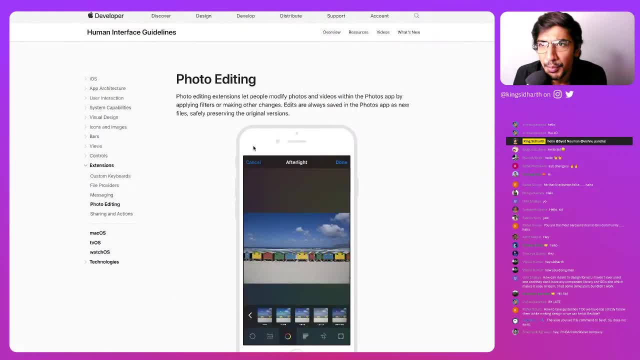 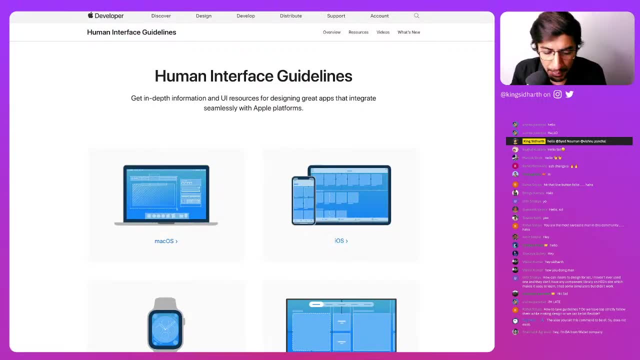 through that? oh, I don't know. I think these are just them promoting their apps, and there we cover human interface guidelines. but let's go to the actual example. like we looked at the note notes app, I want to show you the actual, real example, one of the best examples of Apple's own implementation of their own. 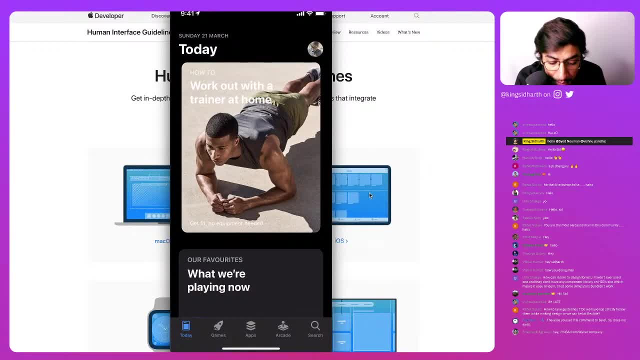 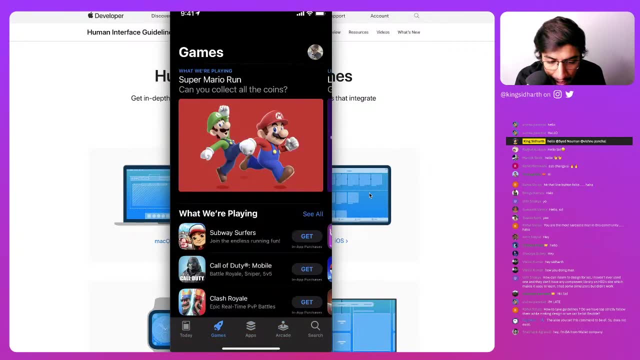 stuff which is app store right now. this is: you can see below our tab bars, right, you can see I can switch between tabs and above is and I can scroll. this is a view. there's a scroll view in. you can see I can switch between tabs and above is and I can scroll. this is a 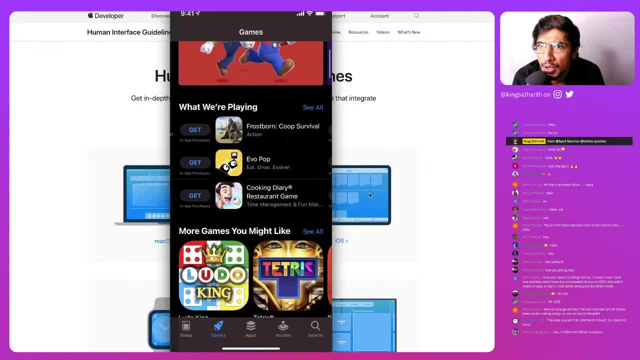 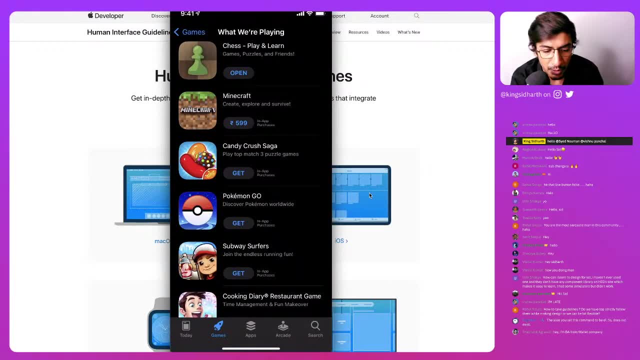 inside which I have another vertical scroll which and which is not covered in the guidelines. funny thing. then I click on see all and I get this inside view where I can go back and you can see the tab bar on top right and suddenly you see a slight inspiration, modification of what we understood, a table view, but you 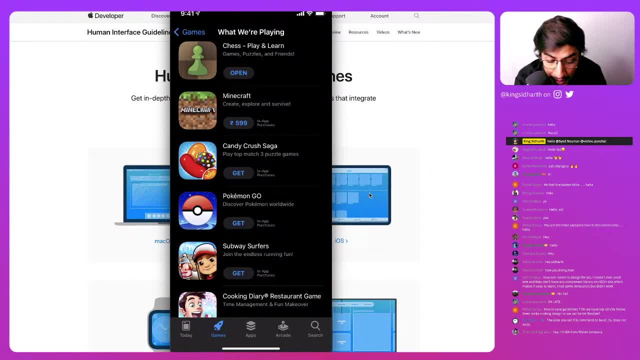 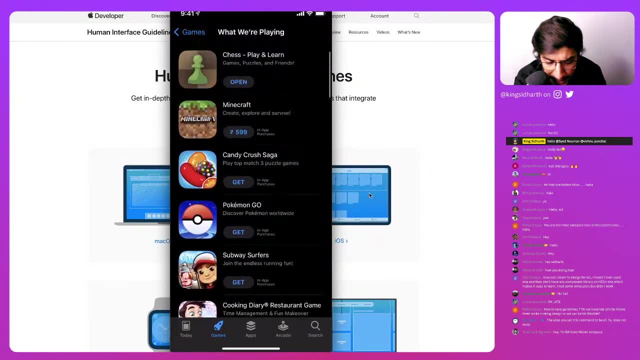 also see buttons. the button we did not see documented in the guidelines, which is like open 500, sorry, five, five, ninety, nine, get, get and et cetera, et cetera, et cetera. I can go back and I can see another, different view of that. 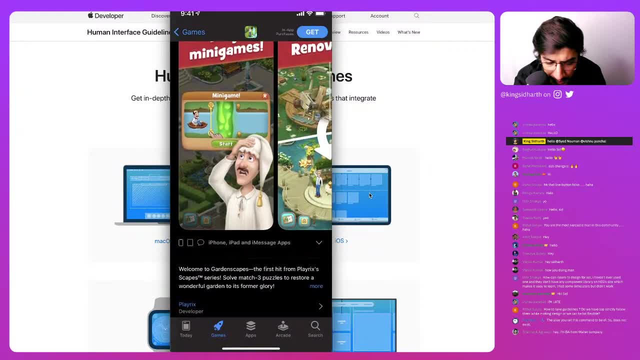 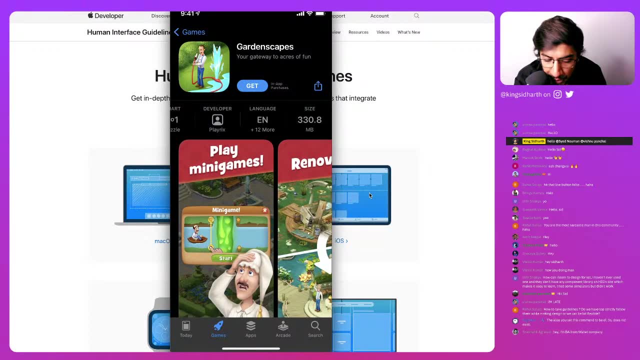 And in fact I can click on individual item and I get to another, something else, another view, And the tab changes. You see special, another button treatment And you see this special thing which I can call- I think often we call stats. 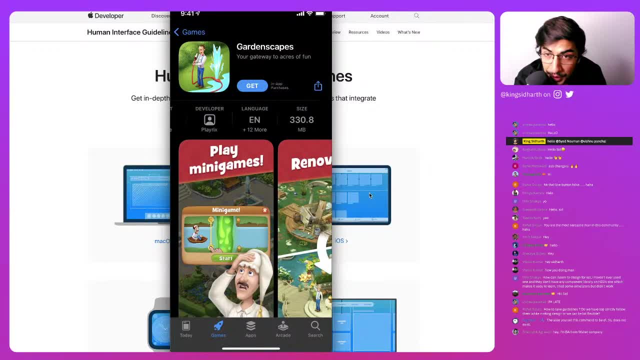 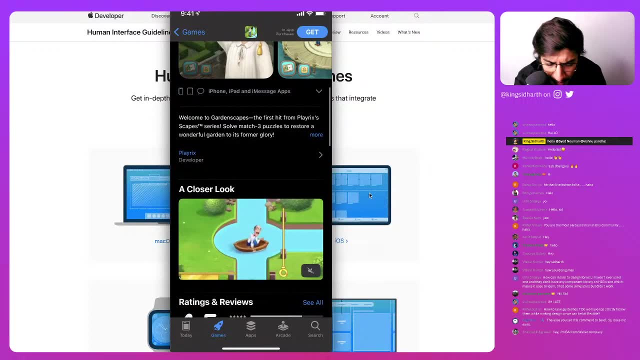 which is again not documented in Apple's guidelines. But again, you can take inspiration. Something like somebody like Twitter on Instagram would follow very similar language, in which case they often do, And then we see even more examples, especially rating something that they have not at all covered. 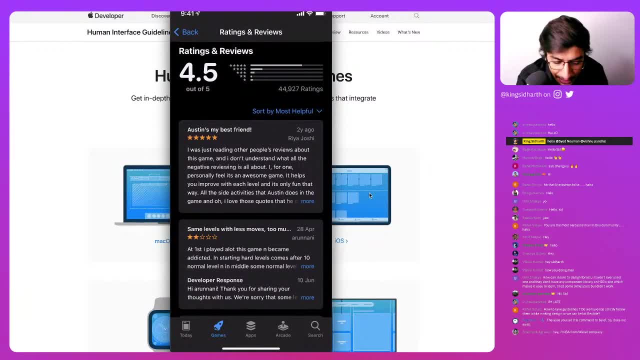 When we look at rating, you see another view: view inside view inside view. the thing continues, And we can, in fact, go one level deeper as well. Oh, they're not allowing it right now. In some cases they allow. in some cases, they allow. 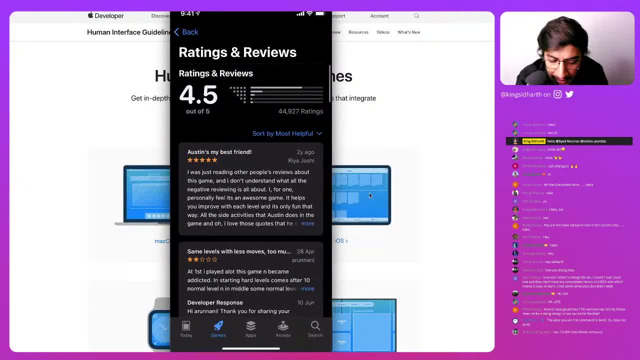 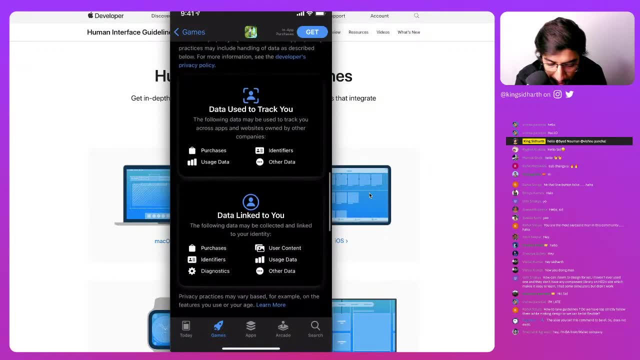 And you can see this is another scroll view. I can go up This rating funky thing is also not documented, but another inspiration you can go for And If you go here, this is again a very different, non-documented, non-standard thing that we see. 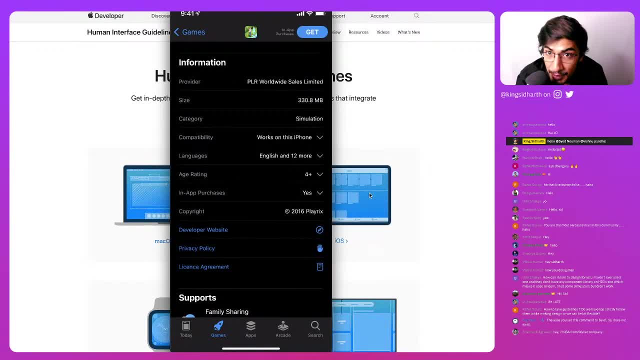 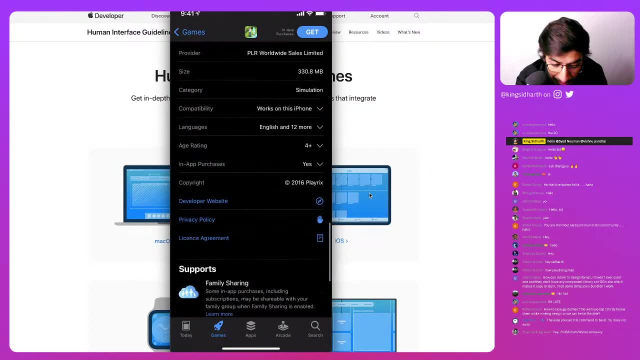 Again we see a table view right. This is again exactly what they talk about in the table view, but very different implementation. Instead of these actions going inside, there's just normal table rendering information, but essentially it is a table interpretation. 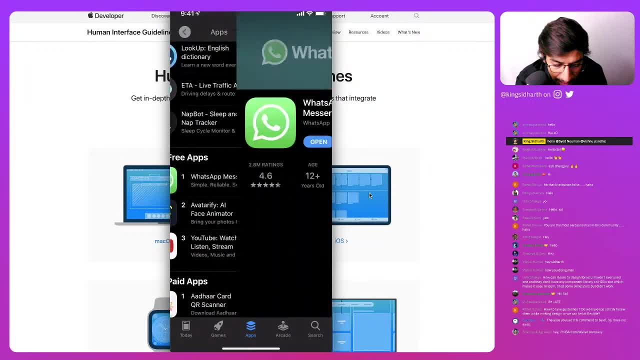 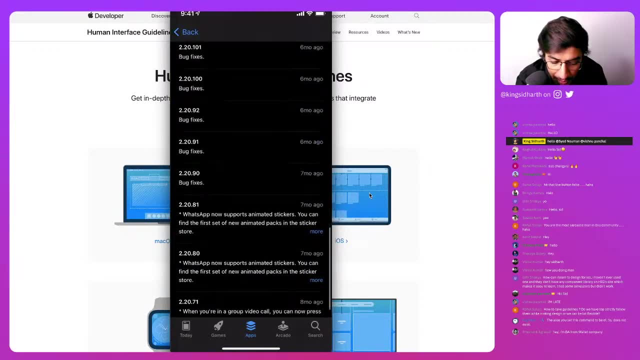 Then we go to apps. right, I can go to an individual app, I can update it, I can open it and I can see version history. Oh, that's another list view, right? List views are also not very well documented. 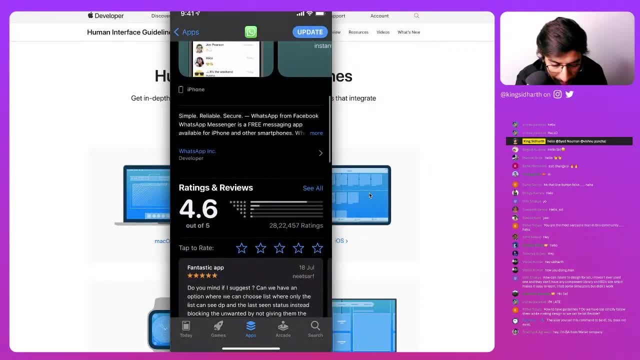 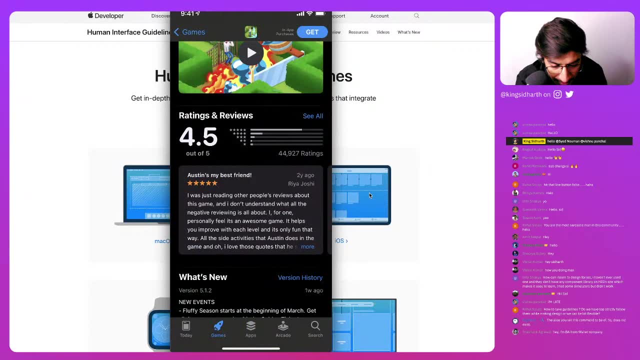 They could be considered a special case of table views, because there's no such thing. I have not seen a such thing as list view in iOS guidelines. So, uh, one of my favorite things is like if you go to homepage and you scroll down. 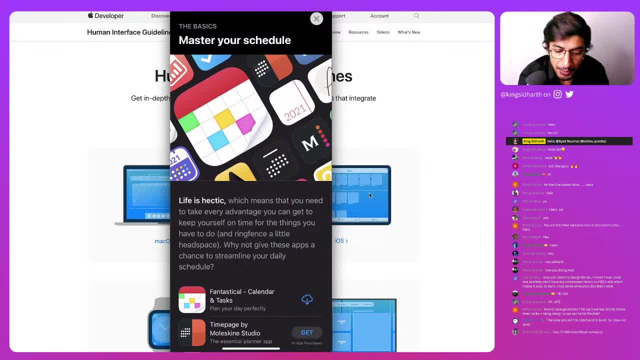 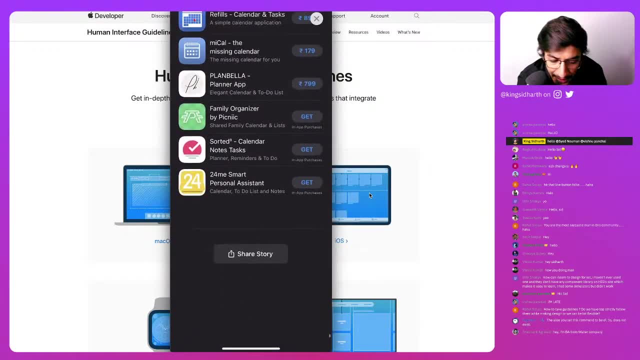 you often have these entire pop-up, like you can see the. uh, it's a pop-up because there's on the top left corner. top right corner there's a close button, but you can still scroll inside it And this is. 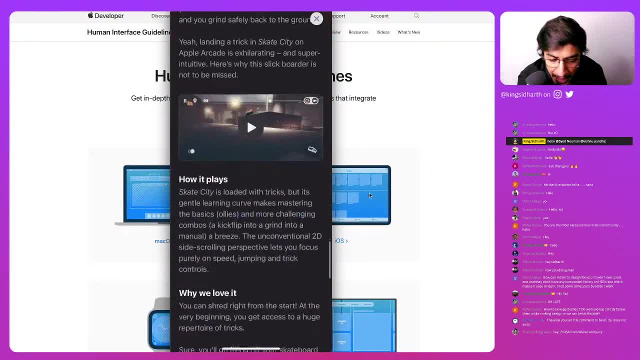 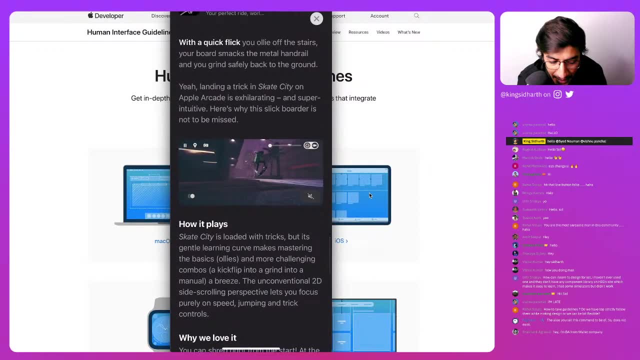 I think the new interesting interface pattern that was introduced by Apple And you can see there's usually you can have a video up there, You can have video in between and a content view Like this is all embedded right. There's video suddenly in there and, like you can see, 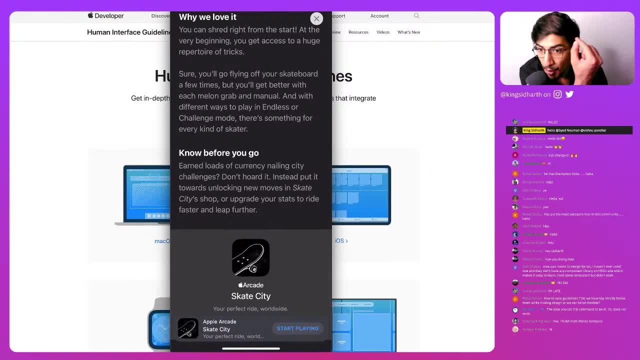 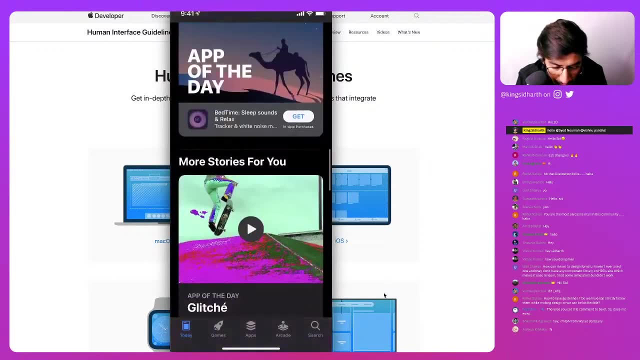 just start to see different things. There's- do you see that thing popping popping up below this small thing? below? There's also not very well documented, but also a pattern used by iOS. So, in my opinion, if you really want to observe, 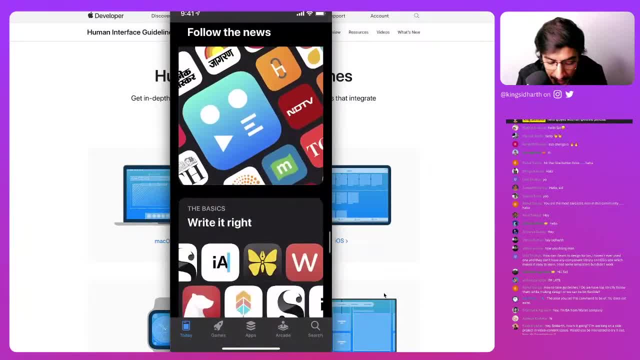 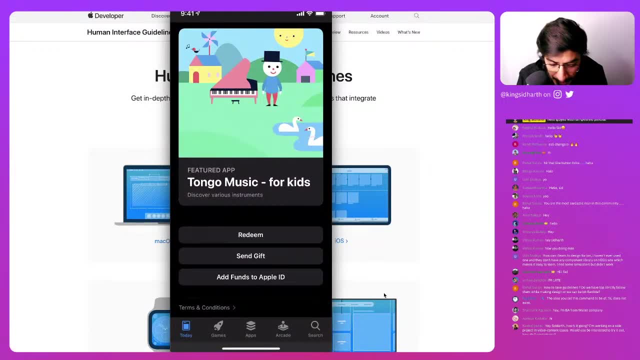 look at notes and look at um Apple's um store, app store, and you will find find amazing examples on how to design for Apple's. um guidelines and search is a standard implementation here, Like you will see, a chess. 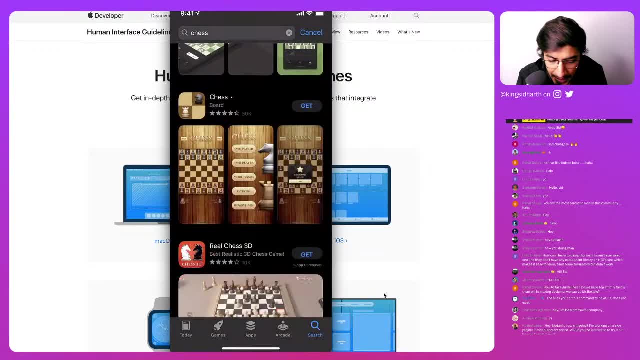 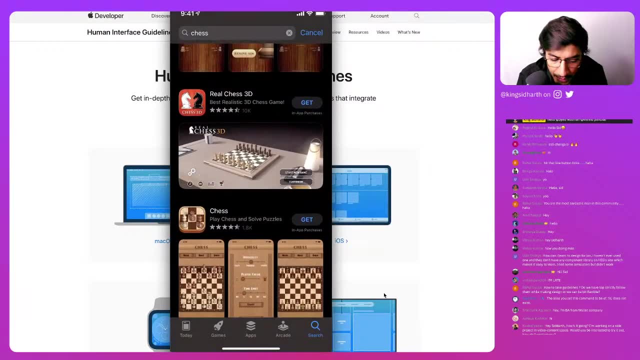 If I look for chess, if I search for it, you can see. it's a standard, you know thing, And this is a new thing. I mean, they've designed this entire thing custom, where they show either three things or a video, or one highlighted thing. 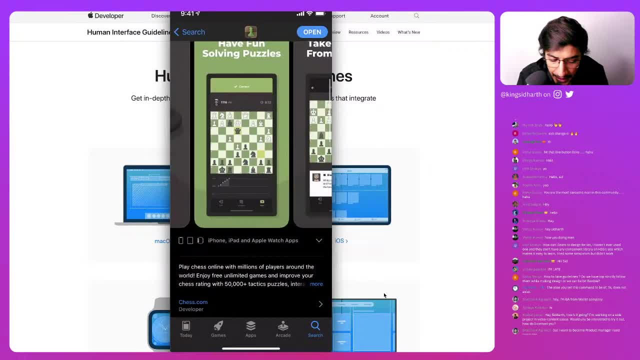 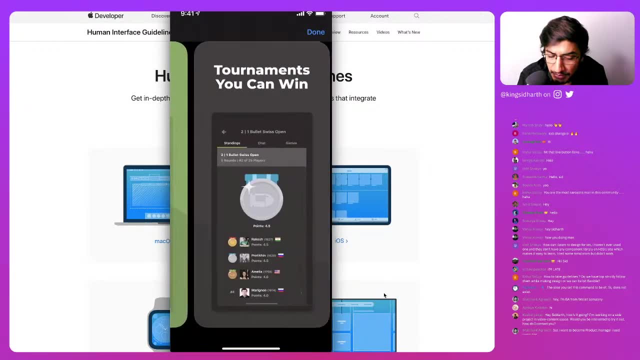 But yeah, uh, you can go to an individual page from here. Here we have, uh, you know, all the screen views, app reviews which you can zoom into individually, And this is this is not covered in their photo views. 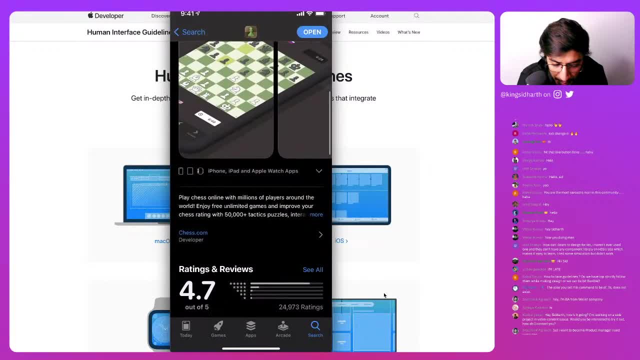 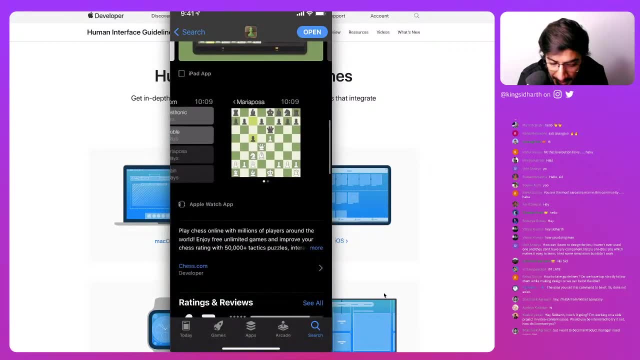 but a gallery view does exist. for many of you out there who will be implementing gallery views, You can also see different screenshots for different you know uh devices as well, And apparently it's also available on um Apple watch. I've not been able to play it. 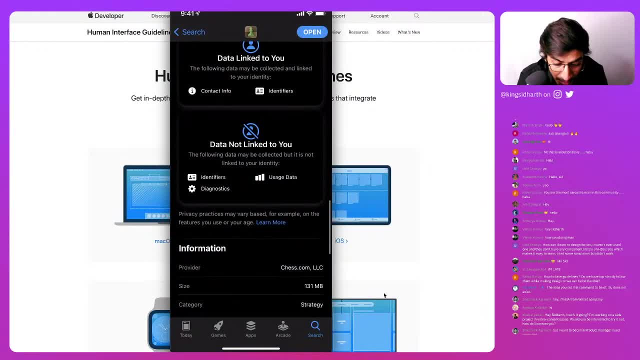 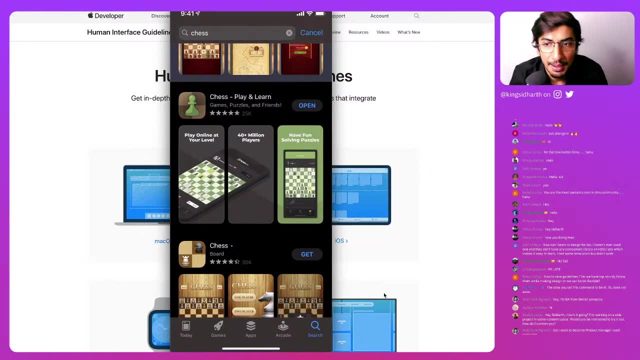 Probably my Apple watch is very old, but chesscom is available on Apple watch as well. What data they use, what data they are allowed to track, et cetera. But yeah, that's implementation Of Apple's iOS guidelines. before we go ahead, ahead and look at other examples, 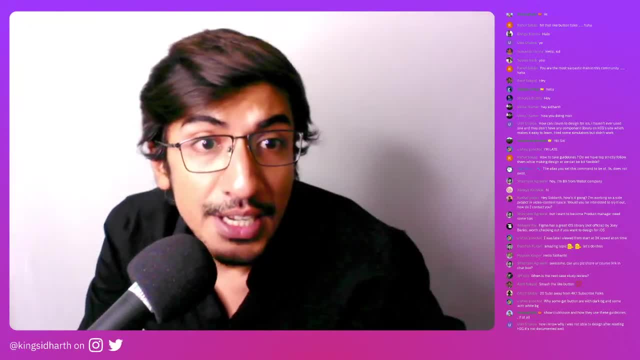 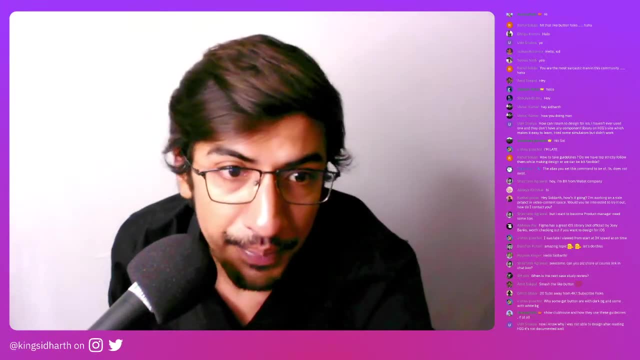 maybe macOS and watchOS. Let me know which one you want to see. Let's take a look at chat. So, before I get through the end of chat, let me know should we cover next? um, macOS or watchOS? which one do you want me to cover next? 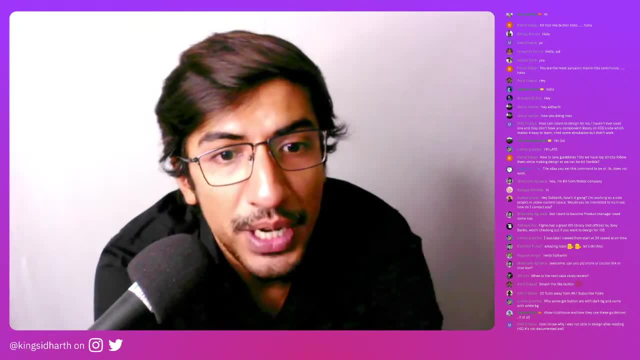 All right, Hit that like button If you haven't already. Hey, so that how's it going. I'm working on a site project on a bit. All right, We covered that. We covered that amazing topic. Let's do this. 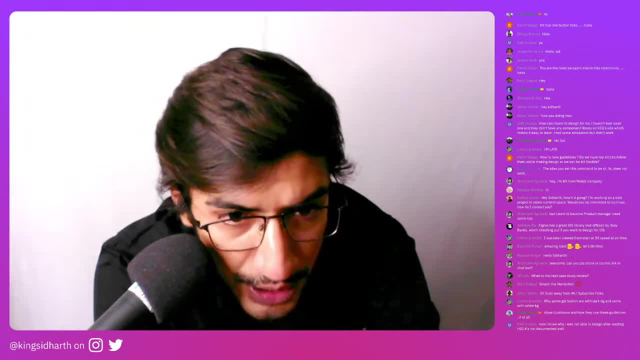 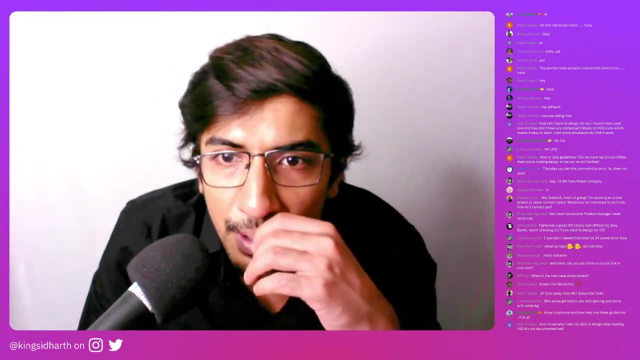 All right, Covered that. Mayank is here. All right, Uh, can you share your post link in the chat Chat box? I can try and find it. I can try and find it, If any of you. okay, The YouTube thing. 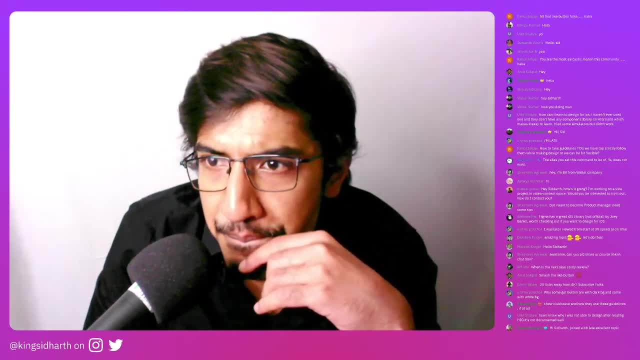 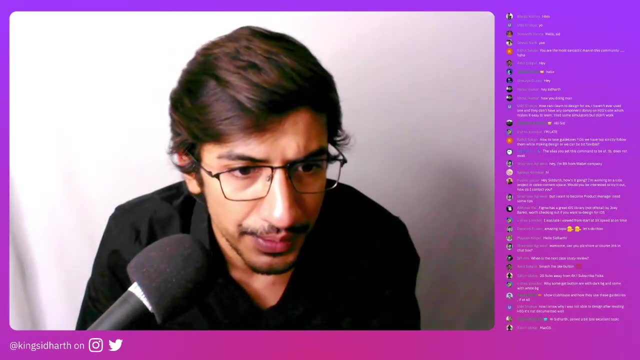 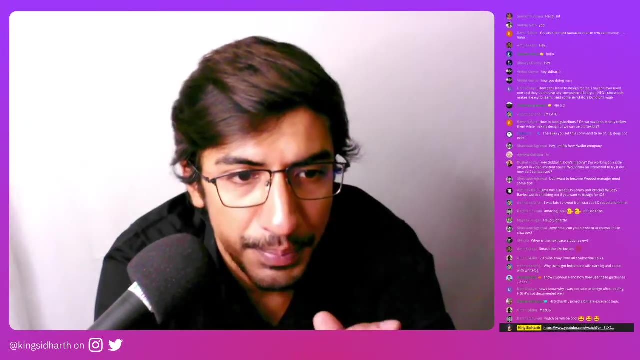 he will not allow you to post um, where is it? Project project: product management course- Hindi, And that is the course link. All right, When is the case Next case study review of SM: It will be next month. 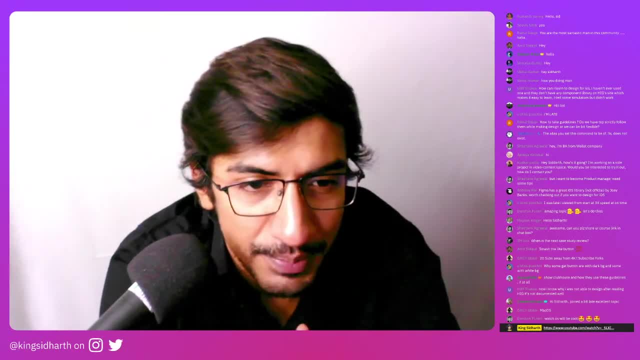 Um, it is saying: smash that like button, smash that like button If you learn something new. glitch says: 20 subs away from 4k. Let's hit that 4k. Let's hit that 4k people. 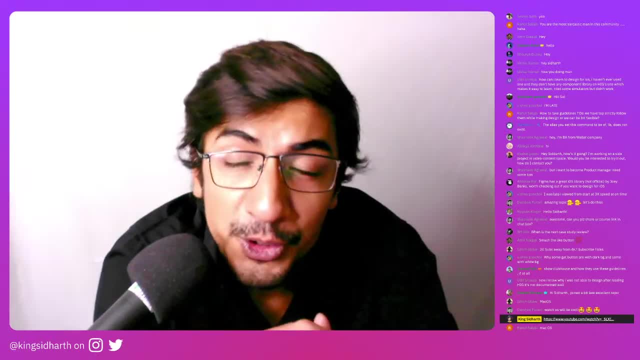 Come on, let's hit that 4k. That's a goal. That's a goal. 5k is the goal for June actually. Well, let's hit that 4k. now I know I was not able to design after reading HIV. 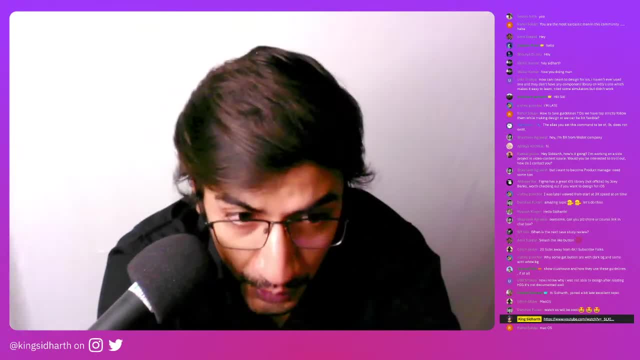 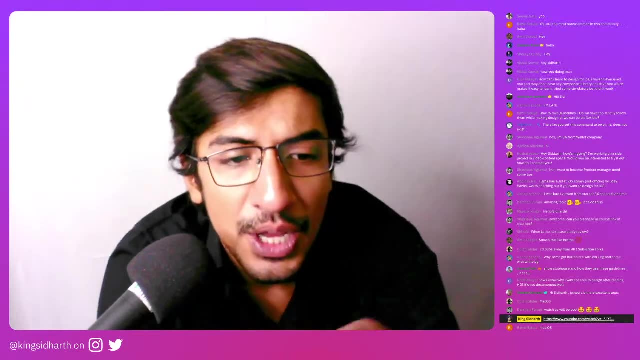 It's not documented. Well, yes, correct, Documentation is not. the song is suit. Apple has the niche. Say is highest bar joined a little bit late. Excellent topic. Thank you so much. No worries, The stream will stay online. 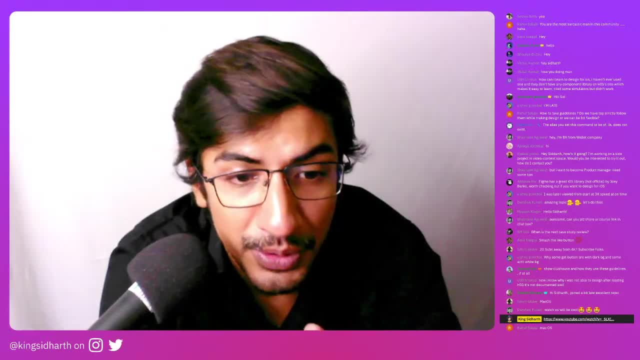 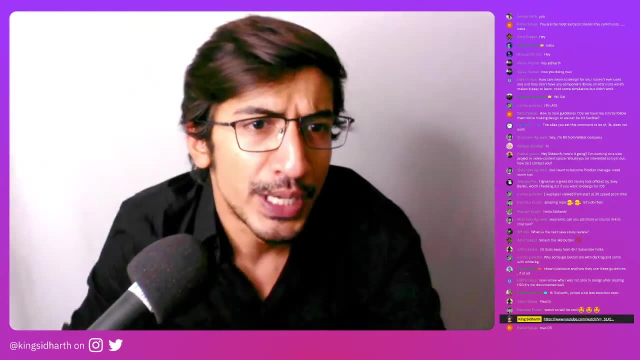 You can check it out later on as well. Mac West, watch West will be cool, Mac West. We have two votes for Mac West. We have one vote for watch West. I'm going to wait on all of you to complete your voting so we can decide which one we are continuing with. 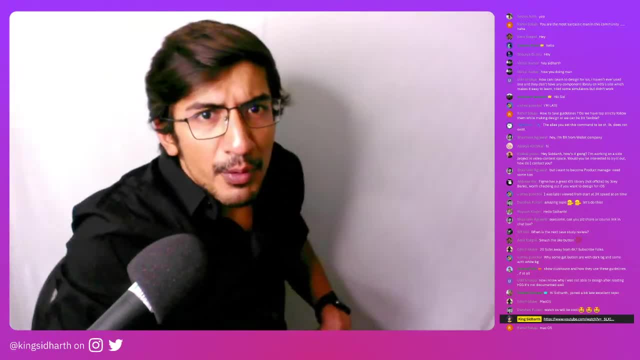 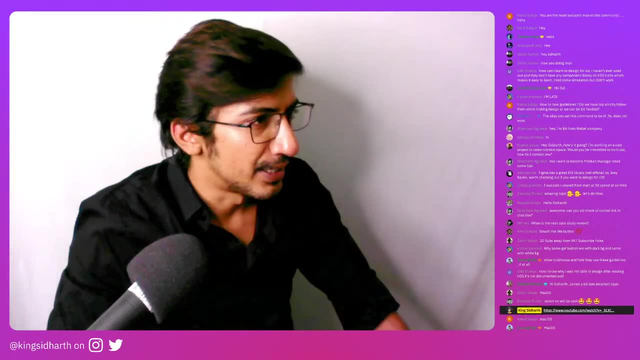 Which one are we continuing with? Hey wait, did you folks? you folks were seeing all of it right When I was talking about all of it. Yeah, yeah, yeah Okay. I recently switched the screen, Yeah, cool. 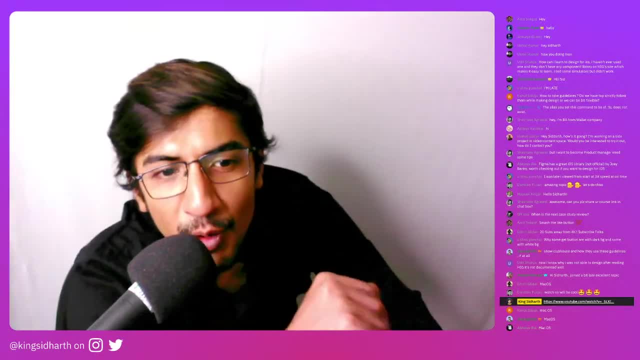 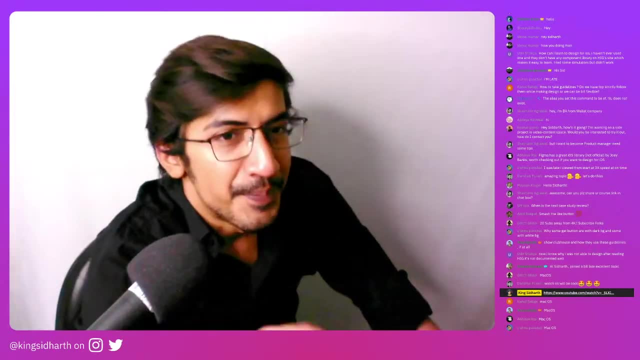 Okay, Mac West, Mac West- Okay, Three votes for Mac West. Four votes for Mac West. Okay, Mac West is winning. Mac West is winning. Fine, Mac West, It is. I'm going to click on Mac West now. 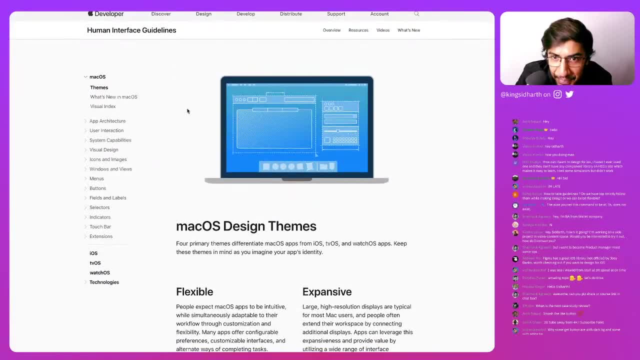 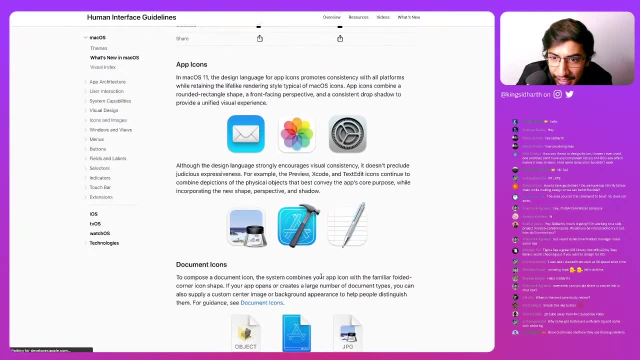 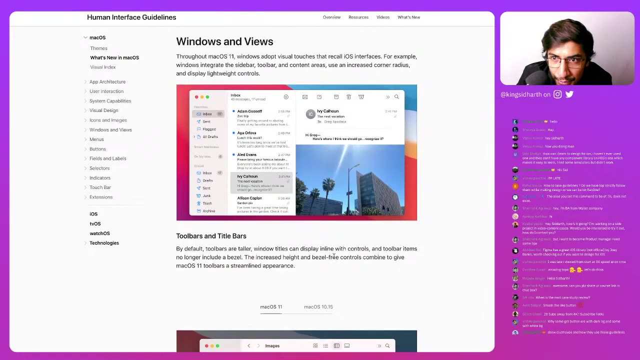 Mac West is an even ancient beast. Um, they start, I don't know why. Uh, of course, there's what's new in uh Mac West of the talk about that. They have upgraded the app icons, The accent colors have been introduced and you can have something called windows and inside which you have views. 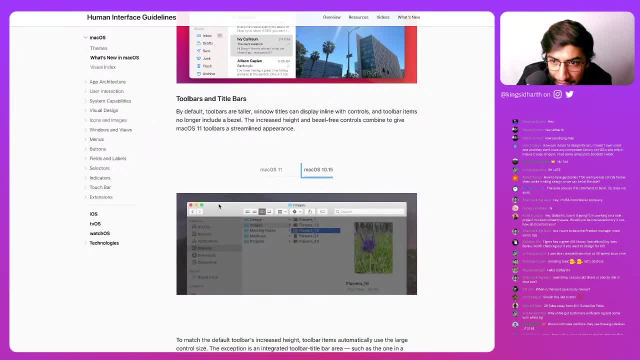 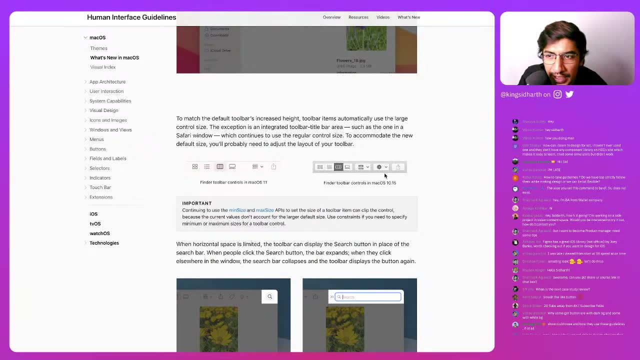 They're defined, called something, called titles. earlier Mac, earlier They used to look like this: the primitive thing, And with Mac West 11, they have changed it to much more touch. friendly issue can say, and it's much more simplified. 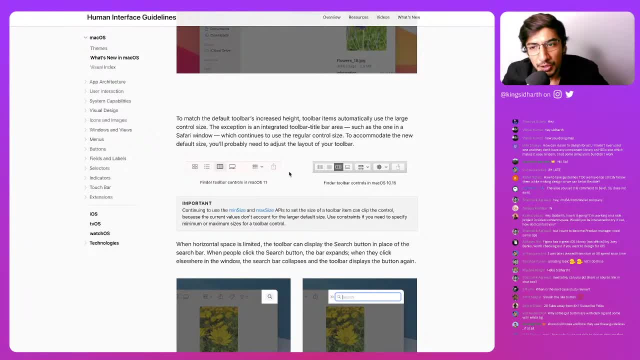 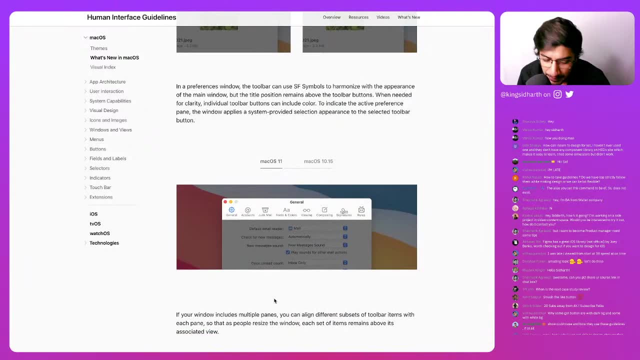 This was a complete desktop paradigm and this has upgraded to this much more. what people are calling- I think the best way to describe is touch friendly, because that touch tap target thingy is. so this thing, even if, um, the Apple should, even if they're not bringing touch to. 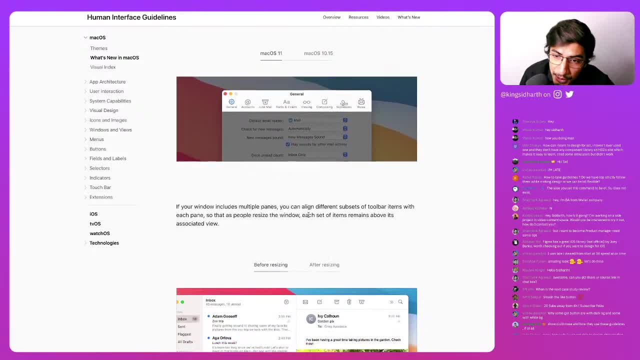 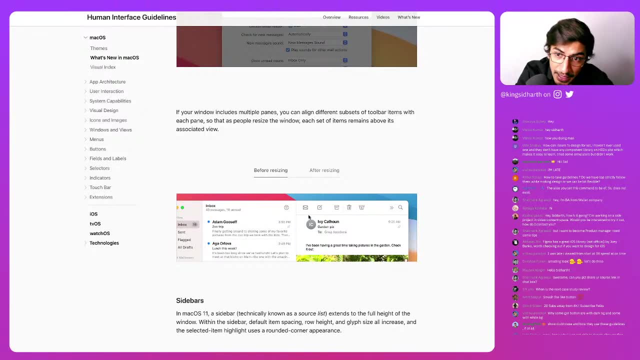 uh, you know Mac devices. I think this unification was much called for. but with them approaching that unified architecture with um Apple, uh, SOC, I wouldn't be surprised. Like, if you want people to use um. 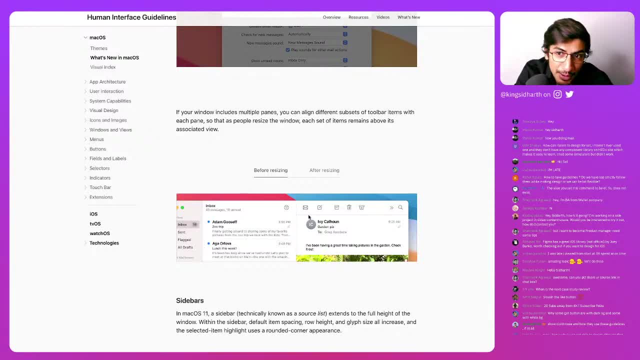 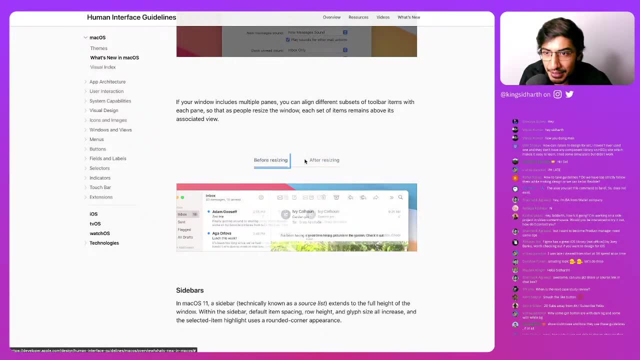 if you can, if you're saying that, Hey, you can now use iPad apps on Mac West, That's has to be coming. I mean, that's has to be coming, the right Um, so they, they are resizing available. 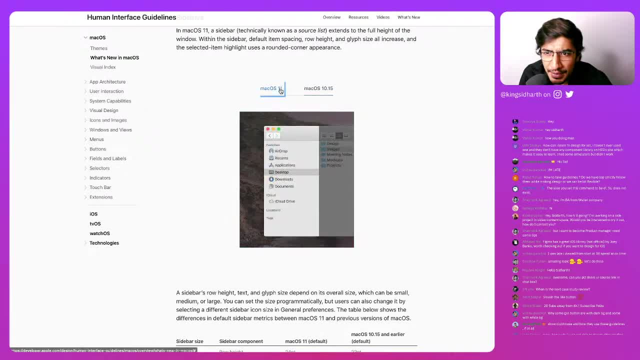 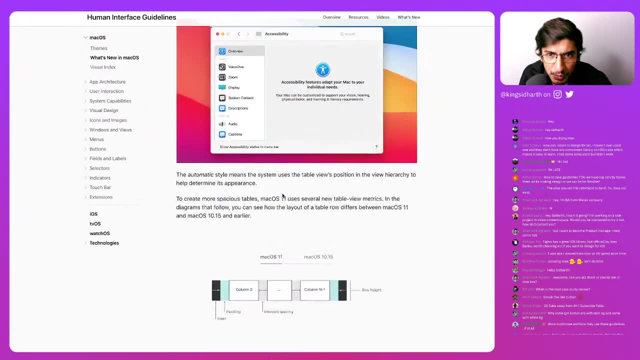 which was earlier not a really thing for everyone. Sidebars have evolved a lot Again, gotten simplified visually. They have evolved a lot in order Otherwise, uh, they also have something called table views, which will get, which will later on. 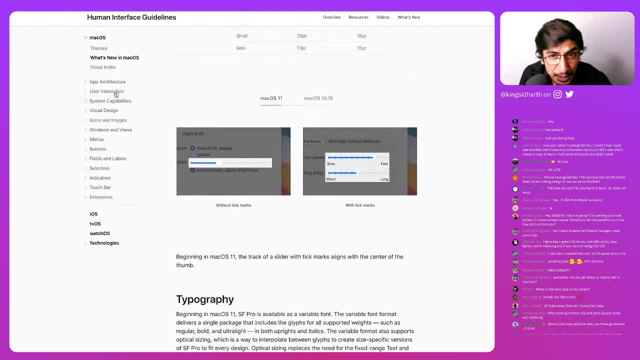 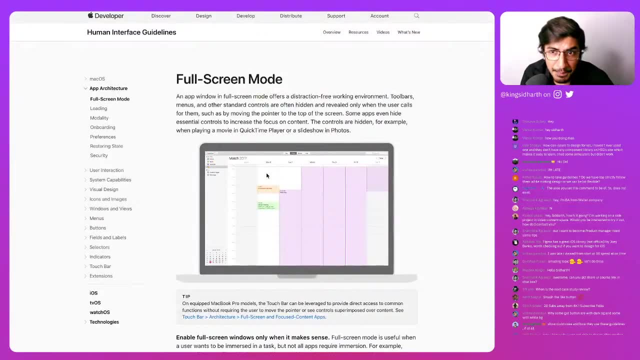 Um, but yeah, uh, it's a massive. this is much more well documented than anything else. One of the things that we know is full screen modes, uh, which are a big thing in um Mac West now, but which is nothing but a full screen. 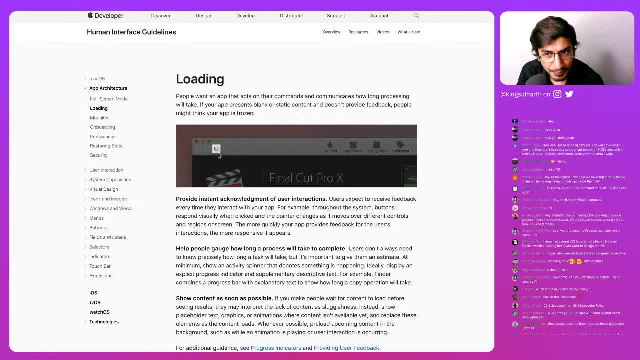 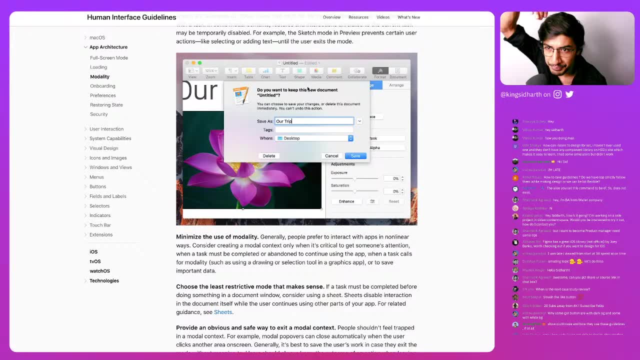 right. I mean, what can you do? Loading as a special area in all the apps, And when they say modality, they all always talk about these. um, I don't know. it's a model, because, yeah, it is a model which opens. 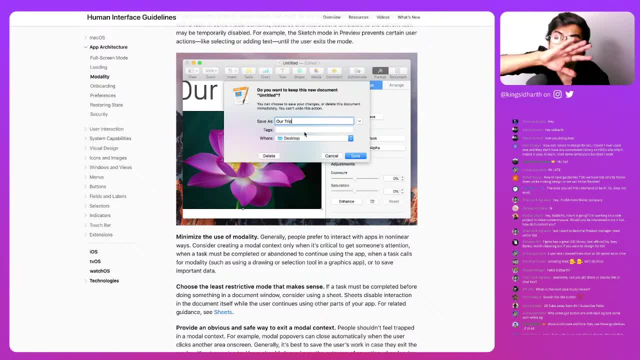 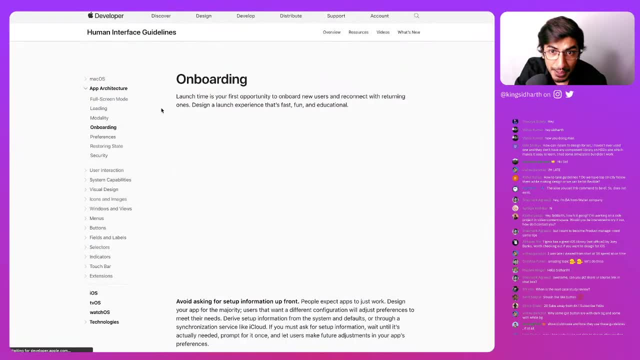 it's like this: It's a nonblock, It's a blocking model, but instead of uh, the visual styling is very different here. Of course, it's used by native apps a lot. Um, again, I don't know how many of you will be designing a native app. 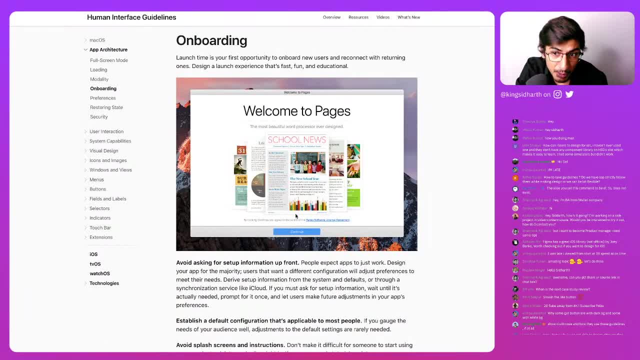 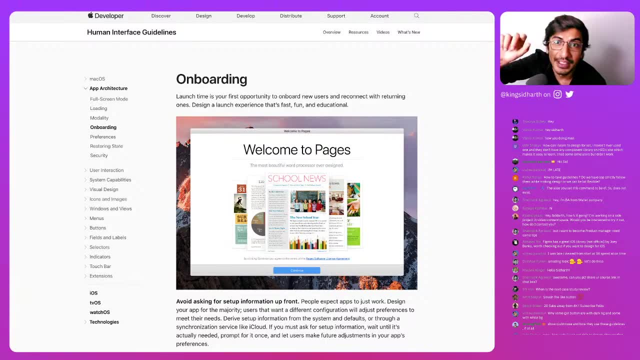 but, um, I don't know why onboarding a special case here, but they do have special onboarding things which Apple's own things, uh app apps used to use a lot. Uh, notes will have a loading thing, Agree. 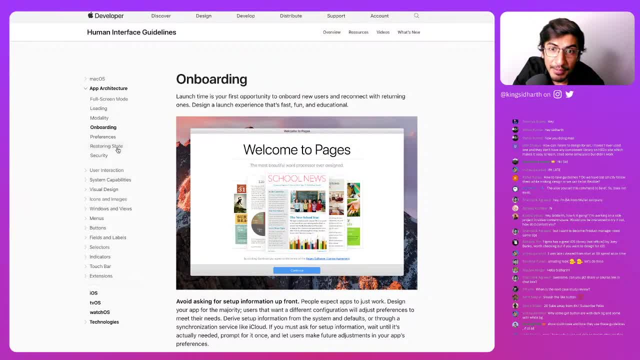 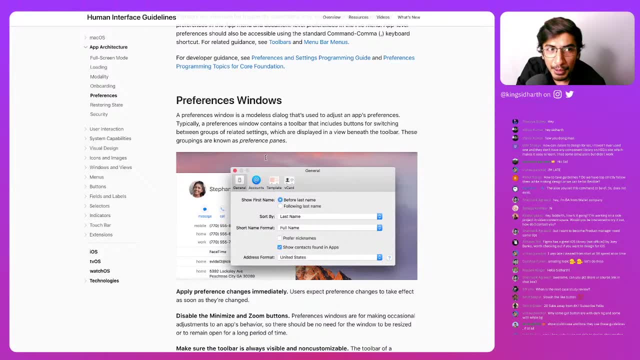 Disagree. Music has a loading thing. Almost all their apps have an onboarding screen. I've not seen that to be the same case from uh other people's uh in other people's apps. For example, notion does did not have a loading screen for me. 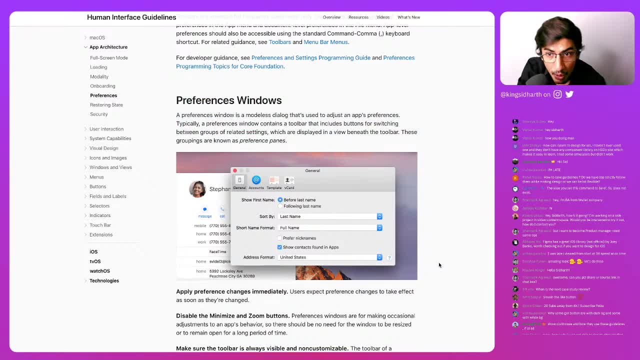 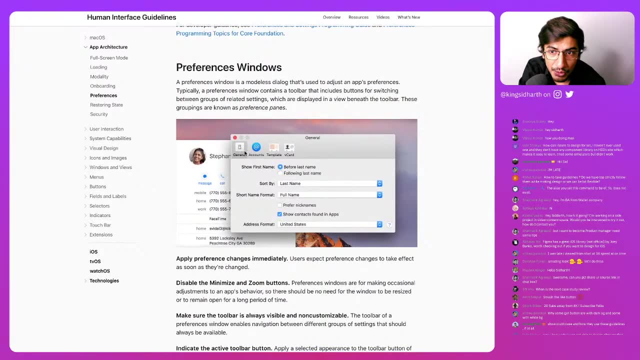 It just was like. login preferences are a standard thing in all apps. All application have something called preferences, which is settings of that application, And usually the standard pattern is to give this kind of tabs on top and give individual settings underneath it. right? 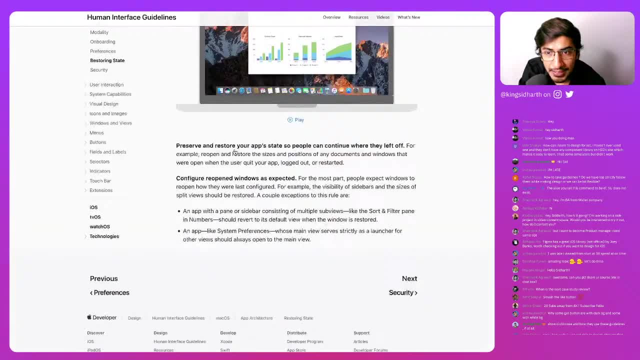 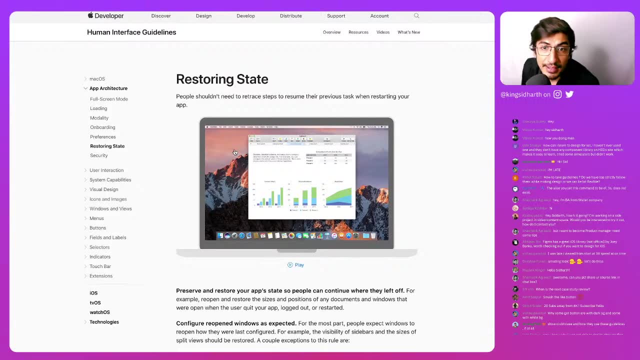 This is a standard pattern. We will see everywhere. Uh restoring state is about like when on a Mac West, where wherever you close the app last, the app is supposed to restore itself from there. This is where uh apps like notion. 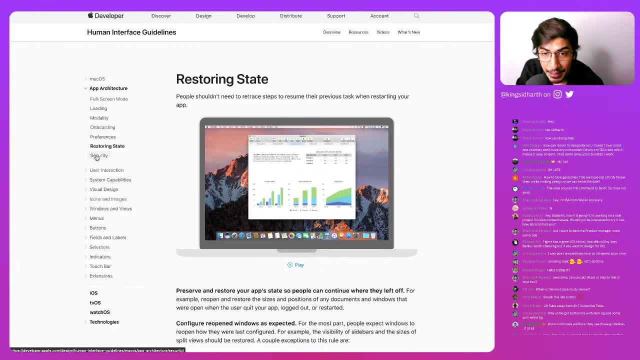 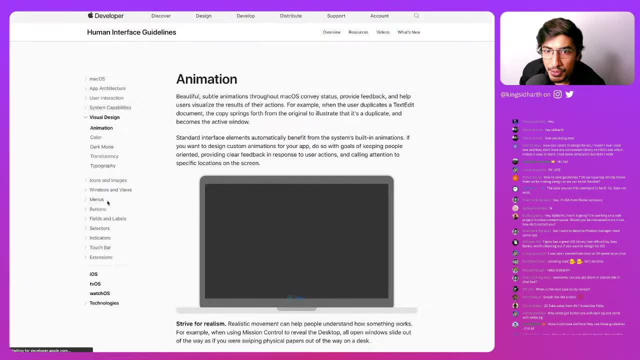 et cetera, break this because they are chromium apps and not native applications of Mac West. Um, in terms of: uh, we're going to go to visual design directly and let's go to some ideas on animation. So they always encourage subtle animation. 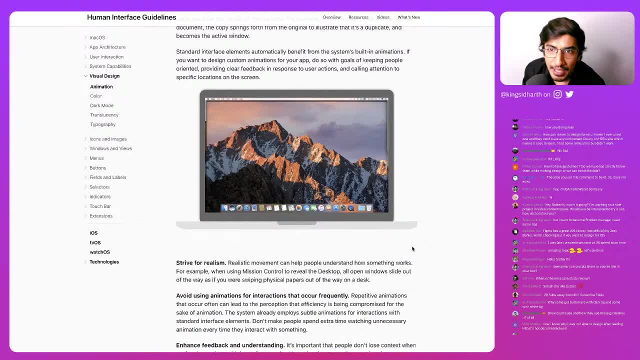 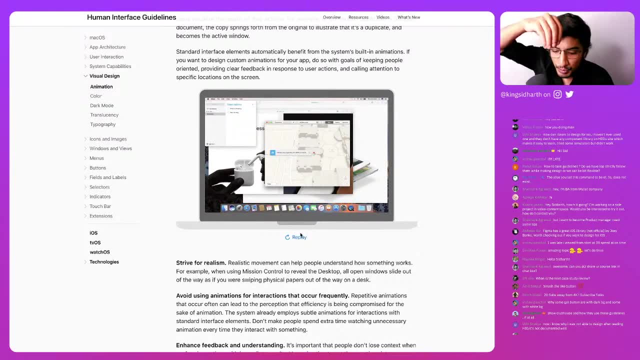 And what do we mean by subtle? Let's take a look at that. If this place- and this is how this, you know all the swipe gestures animate, Now one of the things is, uh, what this does is when you take a track pad or you take this mouse. 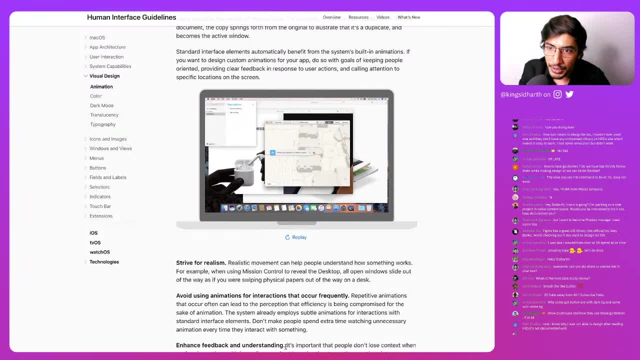 right, And I do this right, Everything will go away. It will do that. Now, the thing here is they're using: if you see, if you closely see the windows, do move away Now. this is one of the first. 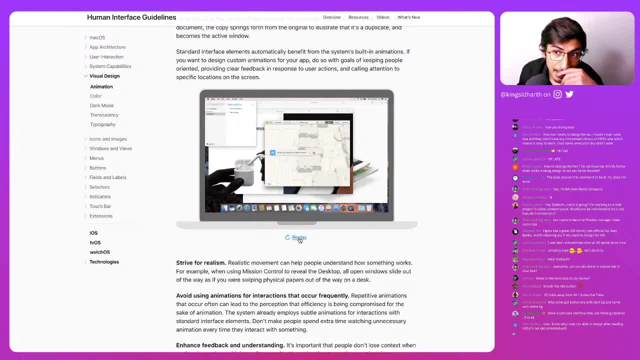 this is- and now this is really old, Okay, And Apple's guidelines. The thing here to note is Apple has been using motion design to talk about space which does not, is not visible as existing since time immemorial, and using motion design to aid. 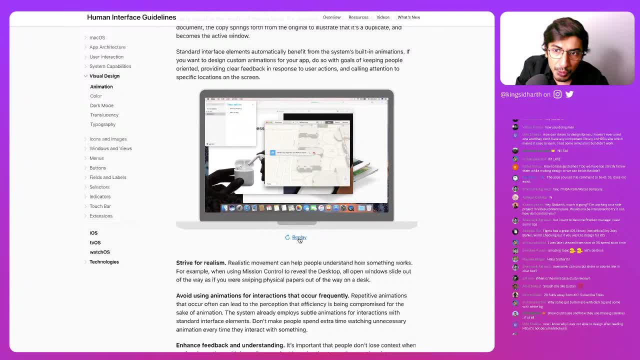 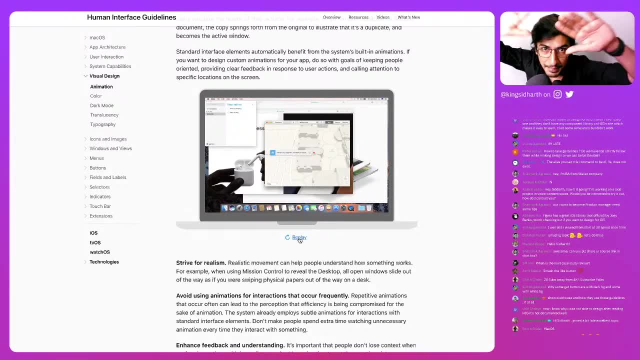 the cognitive, you know, to ease the cognitive burden on the user, because if they just disappeared you'll be like where did they go? But right now my mind is not even questioning because suddenly they disappeared and went into corners and they can come back again. 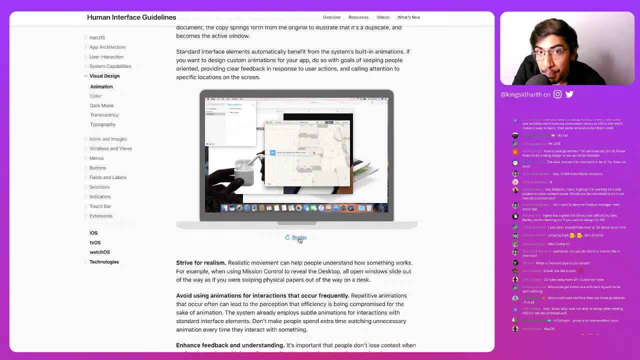 And we see Apple using this over and over again- And these kinds of simple thing that they think about for human beings is why they insist on calling these human interface guidelines. This is where, in their mind, they pick it up from. Let's look at. 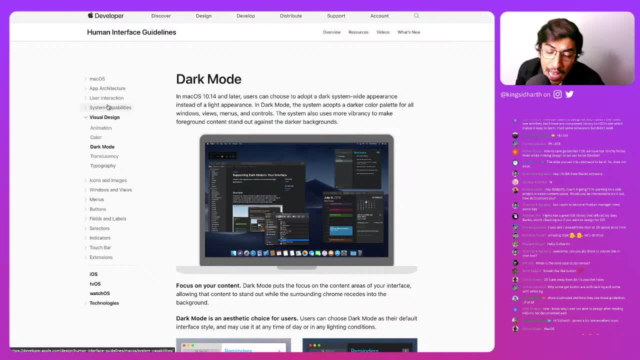 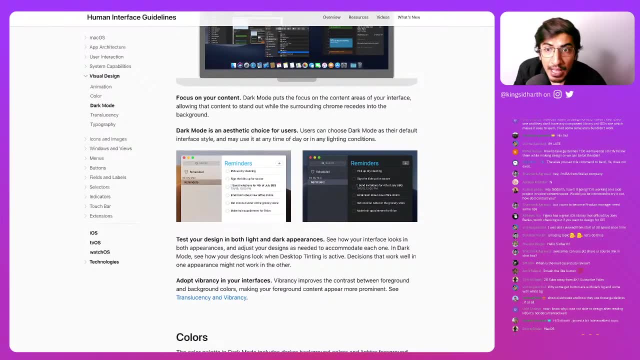 uh, you know MacOS a 10.14 and later introduce dark mode. And why? uh why, Apple promotes dark mode and what did they think about it? In Apple's opinion, it helps you focus on the content and it's an aesthetic choice for users that user can take. 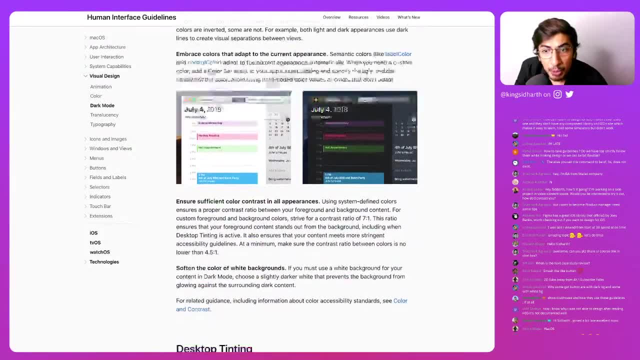 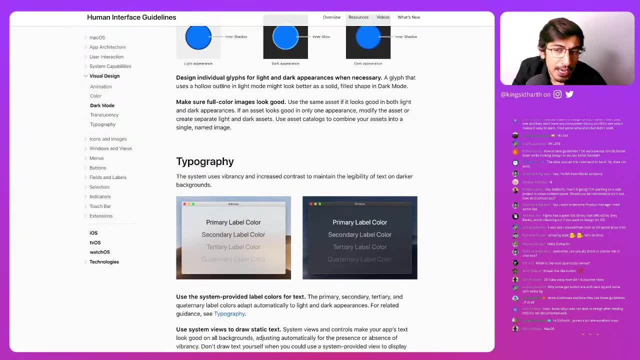 And that's pretty much it. You know they do talk. uh, I did hear somebody mentioning that Hey uh, dark mode can save you a lot of battery life, but that's not true for all the cases. I am still waiting for somebody to produce a YouTube video with detailed analysis. 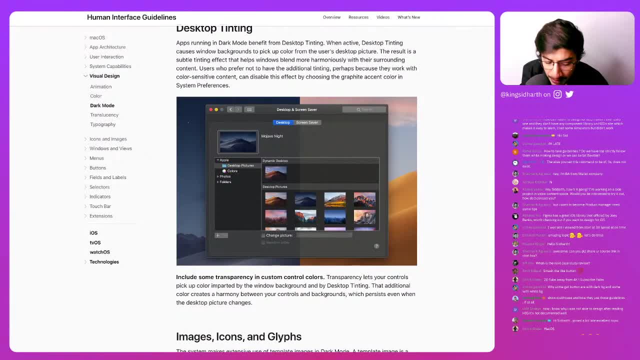 However, uh, another thing, uh, no, here is that when, when we talk about dark and light mode in desktop, there might be true dark and true light mode, but it's not true for MacOS anymore And it's definitely not been true for mobile devices for the longest time. 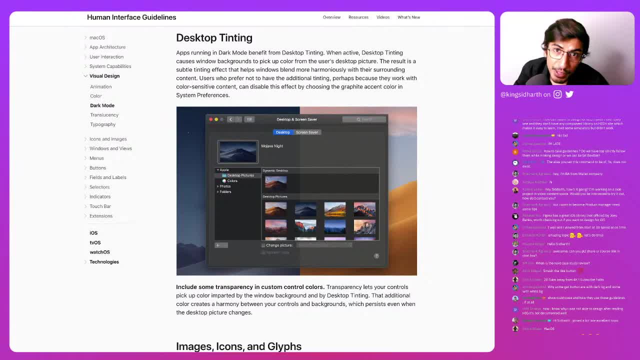 There's something called that tinting. that happens especially on iOS devices, where the brightness and the color tonality shifts. So the gray you think is gray or dark you think is dark is not the same drug throughout the day or in all lighting conditions. 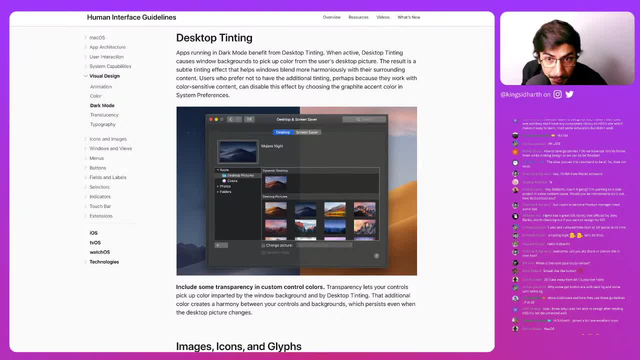 dark has to change and evolve. That is that makes the you know what you're designing for even more dynamic, So that's something to keep in mind, especially for iOS people as well. Translucency was introduced long back in iOS. 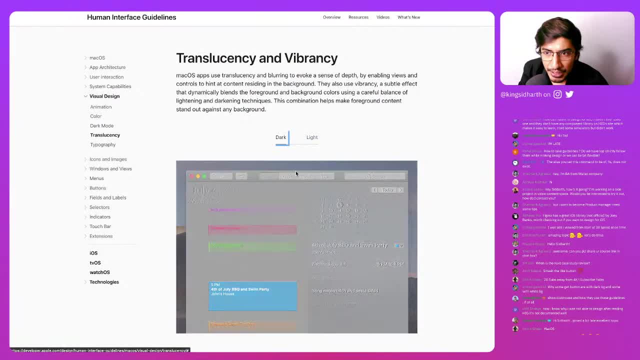 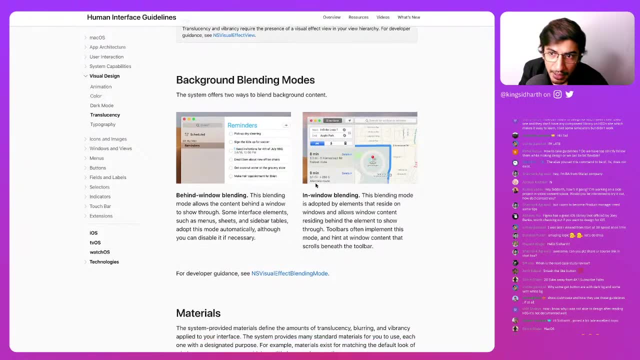 I think I was seven- introduced translucency And then this was introduced- uh reintroduced in fact- later to MacOS. earlier it used to be there and you can see it's reintroduced again. You can see a slight hint of what is in the background here in the highlighted section. 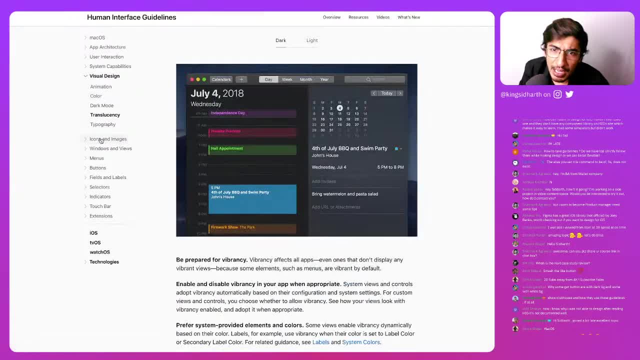 And this is where a lot of people get inspired and want to do a glass morphism on top of it. But translucency, transparency, is an age old thing. Sure, You can make glass morphism out of it You really wanna, but 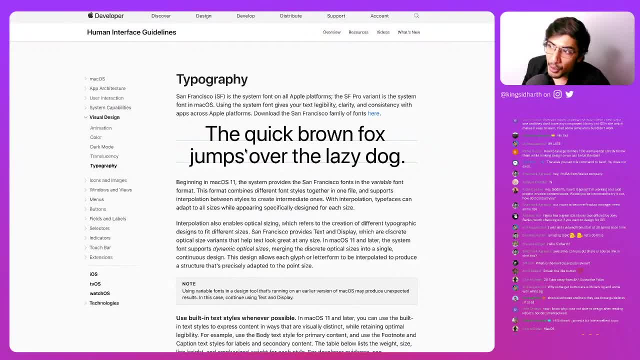 um, unlike newer models- which in itself is an hour- skeuomorphism, which talk about an open statement and open idea of translating elements from one dimension to the other, glass morphism is just very limited, So that's where I find it confining. 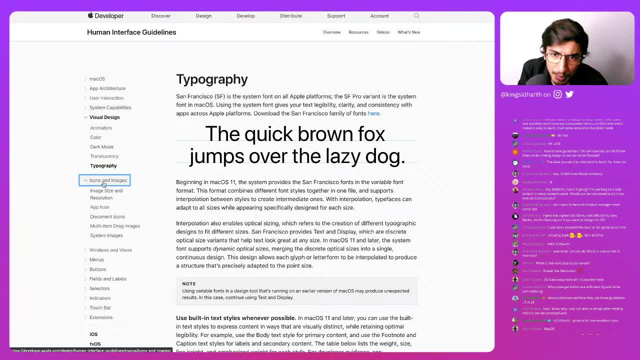 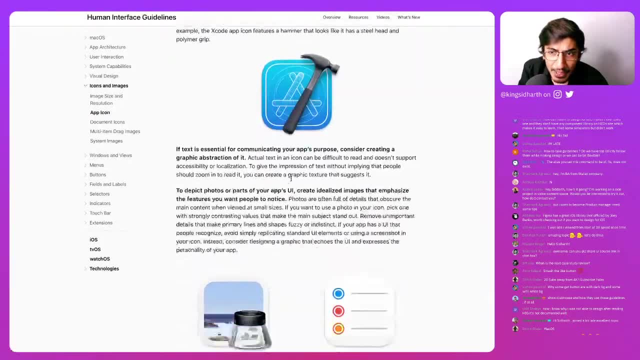 So maybe not at the same par level with neo morphism or skeuomorphism. They obviously talk, have guidelines around how to design app icons. Um, you know what are the dimensions you should have, What are the inspirations you should have. 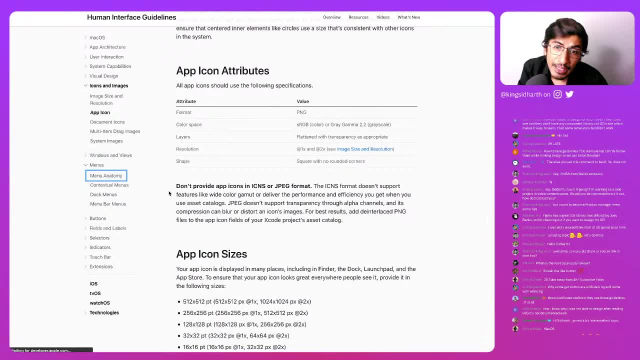 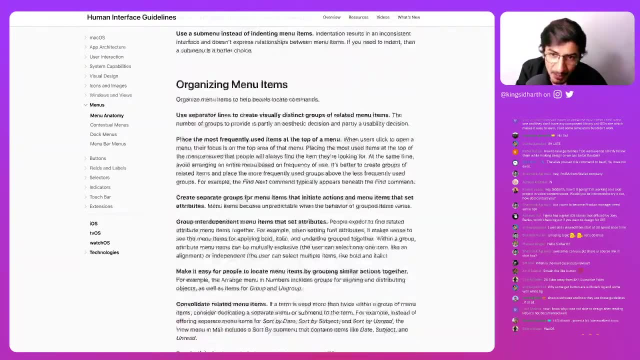 But like, honestly speaking, like everything else, um, let's look at menu as well. Why not? This is the famous complex menus that exist on desktop, which cannot exist in mobile phones or exists very differently on mobile phones, that, like we spoke about contextual menus, are something that change. 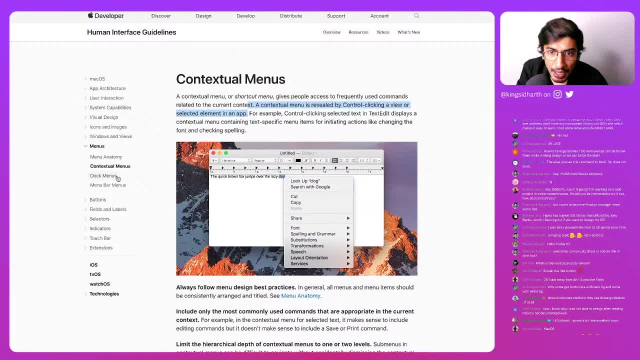 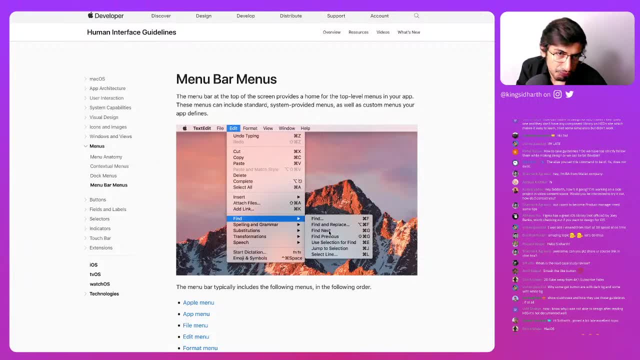 uh, you know, like uh, based on selection. for example, this is the contextual menu, uh, which is I click menu, as we call about them. Doc, menu only happened at the bottom screen, menu bar menus. I'll leave it that touch bar is a special B. 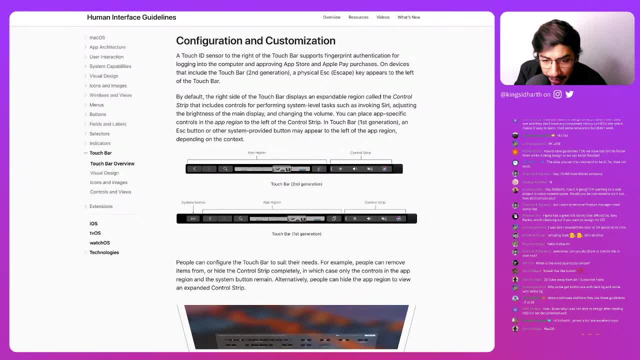 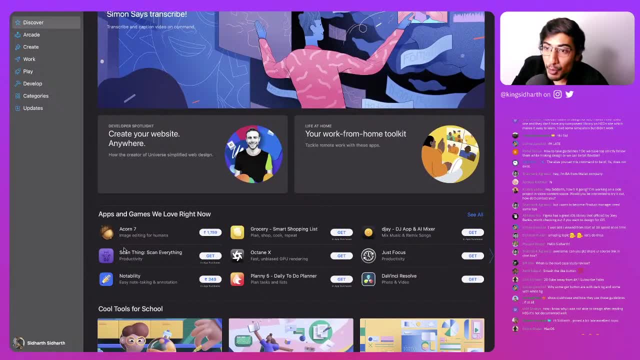 So, just to get this, leave the guidelines behind and go to implementation. and look at apples again: Apple's own implementation of their own guidelines in terms of macOS app store- Again, a great example of how to translate, not only how to design for desktop and macOS. 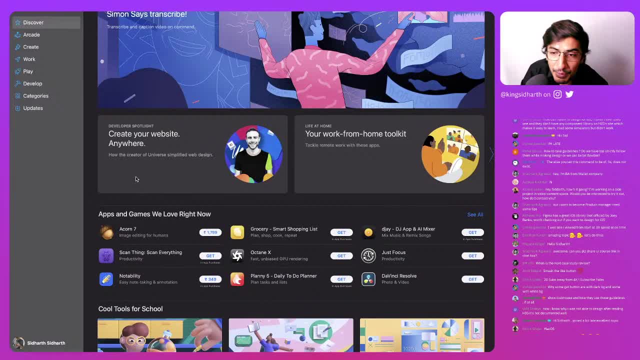 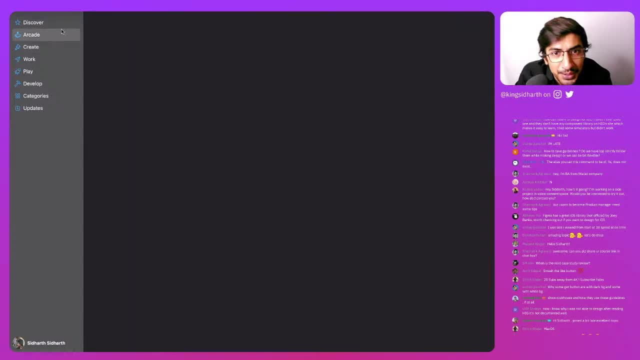 you know when it comes to Apple, but also how to translate these ideas. If you remember, some of these were tabs right earlier that you can use, So this will be just for those who are interested. right earlier, when we were on iOS. now they are sidebar items and search is ever. 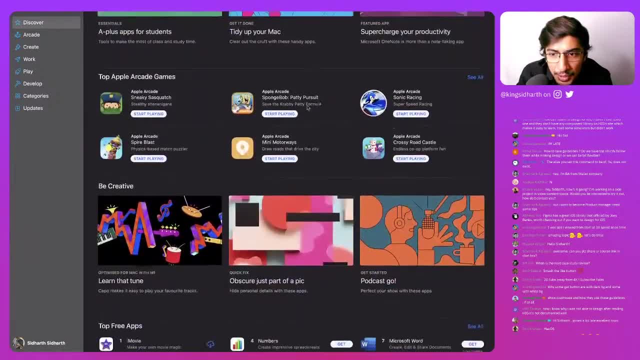 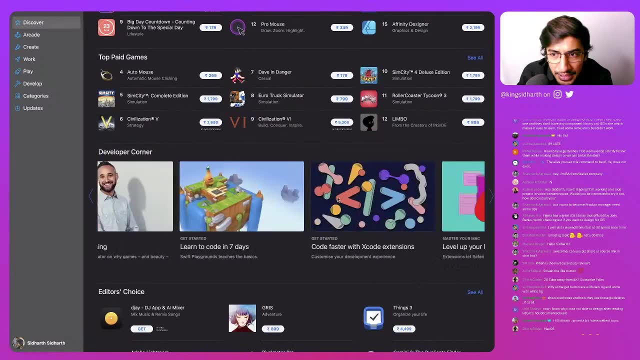 present there and, as you can see, they are card. they were cards earlier. which cards are still here? but they are in. the scroll view is still also here with us and we see this here as well, but much more content is able to surface as it should, and what they are able to do is highlight one item where I can go and 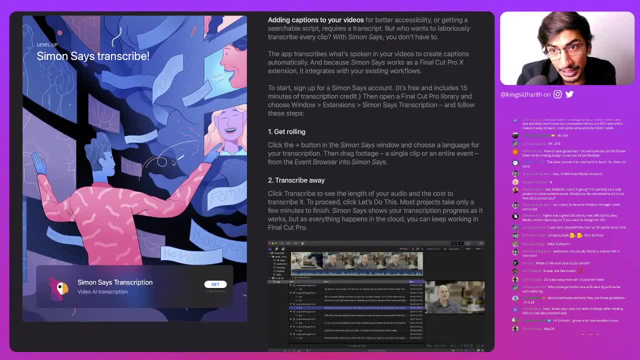 this screen view with the pop-up view earlier we had is translated like this: what irks me is- and on iOS this would have a close button on here- it has a back thing so I can go back, but it's the same item. here I have a static thing. 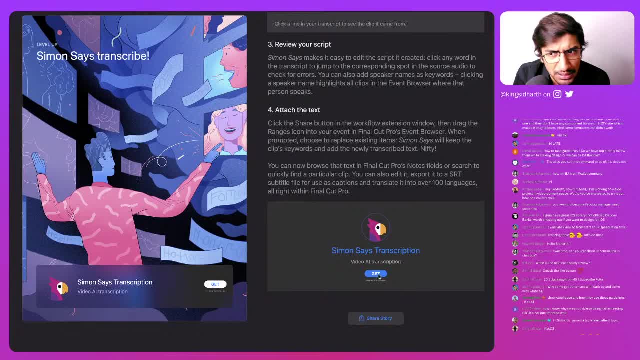 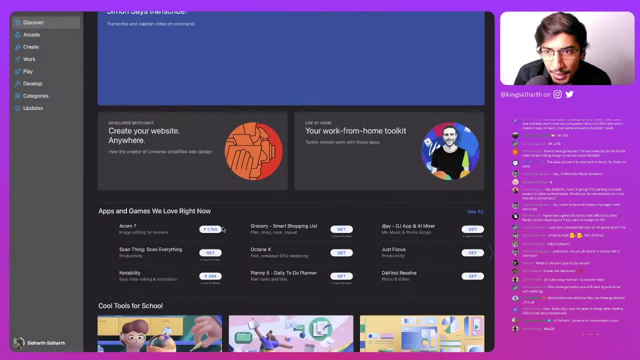 which I can. you know. I have buttons. I have this massive button, the smaller button here. I find Apple's guidelines way funny. I have normal text. I have images embedded in between, and then we can go to these individual items again. these are all these posts here, and then we can go to these individual items again. these are all. 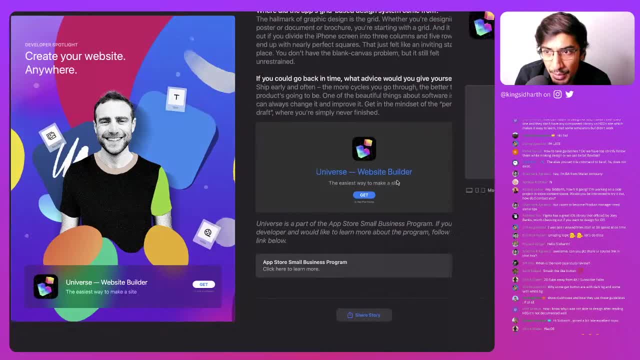 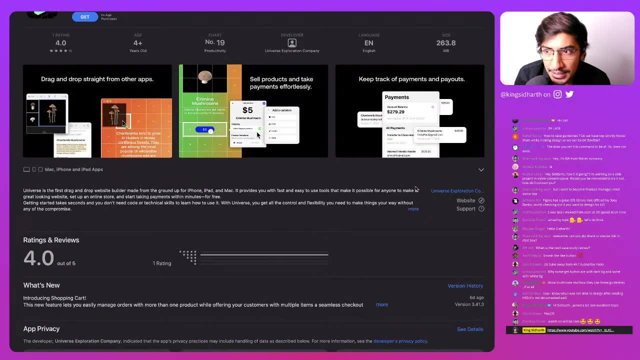 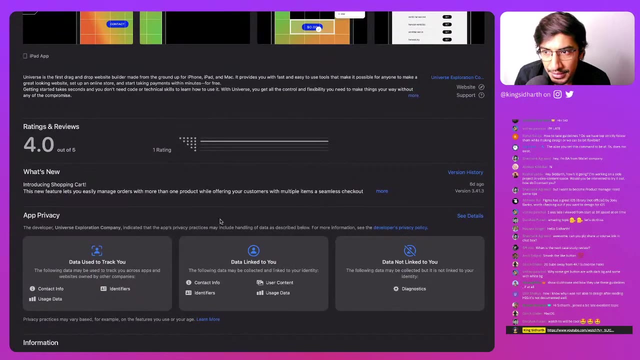 that we see right. and there's an app card where I can go an individual app. if I go to app, I see this again, this stats kind of thing- I see the app screenshots. I see again I can see the app screenshots from different applications: how it'll look on iOS, I will look on Apple, iPhone, iPad, etc. then I see the. 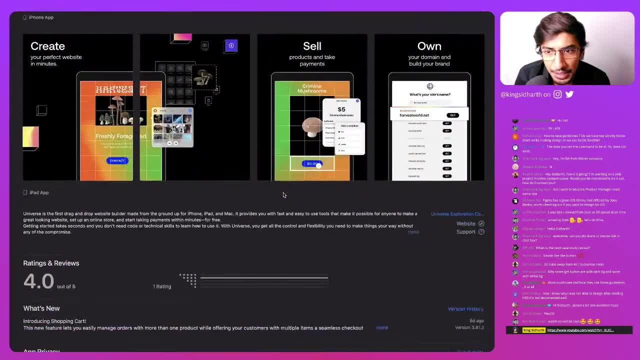 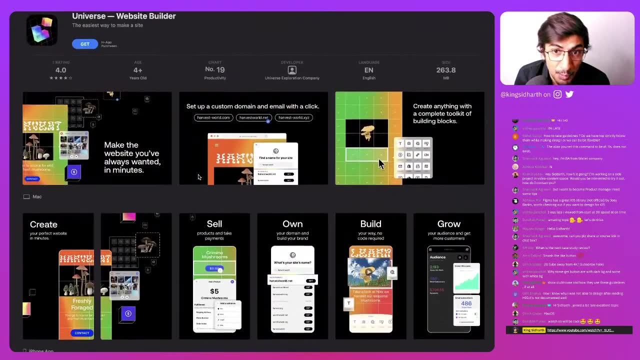 rating section again, and generally a very well translated thing. the only thing that I do really dislike here is the amount of width of text is makes this illegible, right? so this is not where it does not get translated very well, but otherwise I think it's pretty well done. so this is. let's take another. 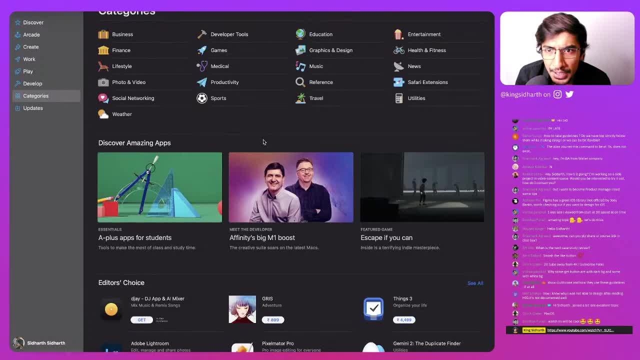 look at, let's say, categories- right, categories again gives you a sort of like split grid view, which was not there, a split table list view, if you will, which was not there on iOS, and this also we see repeating on iOS, for sorry, it was not there on iPhone, it is there on iPads. so this is Apple's own implementation of 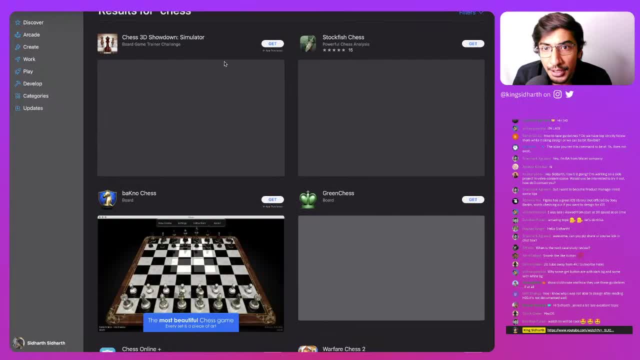 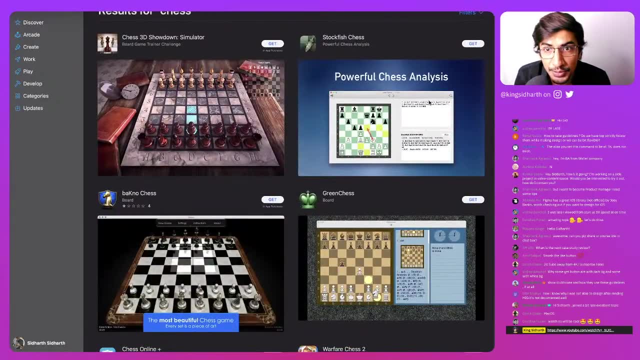 their own guidelines. if I search for something like: so this is Apple's own implementation of their own guidelines. if I search for something like: Again, we saw this with Chess. You see very similar thing happening here. Either they have here. they are mostly promoting single screenshots, not the series of screens, sequence of screenshots. 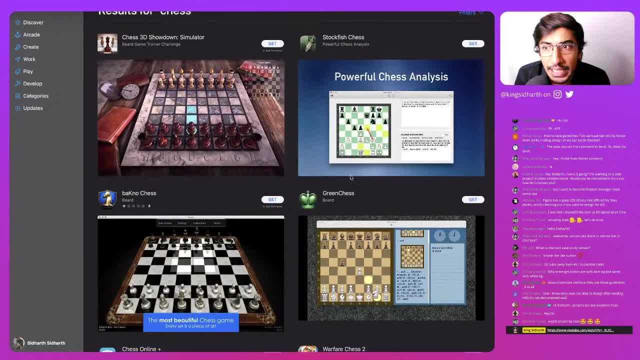 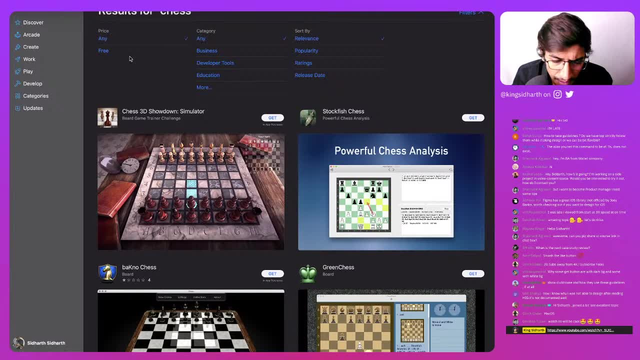 we saw, And, as we can see, chesscom does not have a native Mac applications. Here you can have additional filters. I think these do exist on iOS search as well, but they are not as noticeable, In fact, let's try to look for them. Oh, they are not. Filters are not present. I will show you. 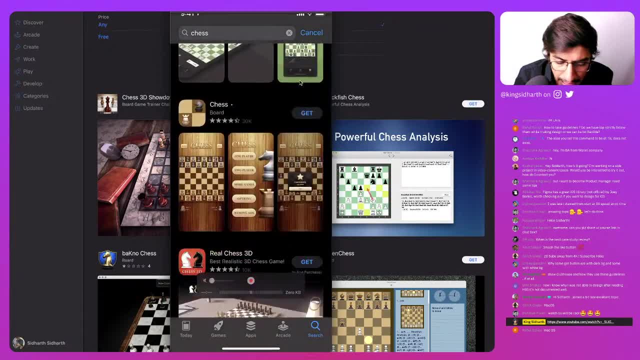 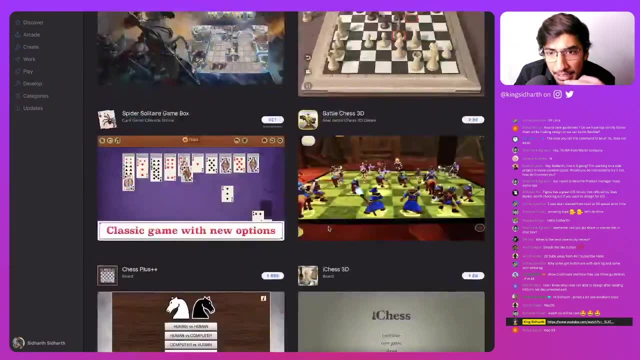 filters are not present here. I can't filter anything here, I can just cancel it, And with that we have covered Apple's Mac interface guidelines as well. Another great application to study here is notes application. Another very well done. Calendar is also an okay application. 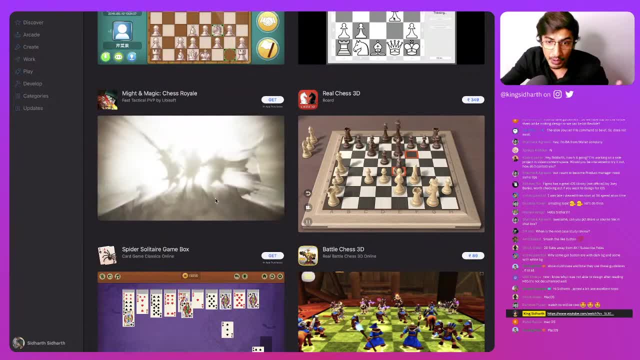 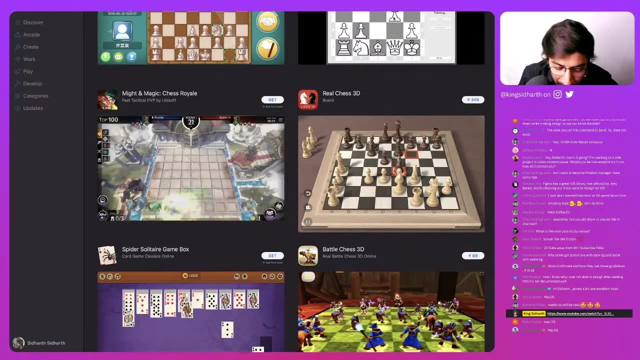 I'm not a big fan of calendar. Photos is another. So photos: I can't open photos right now, for obvious reasons, and notes, for obvious reasons as well. I don't want to open it. The worst examples are: Notion, perhaps because it's a Chromium app not built for, specifically for this use case. 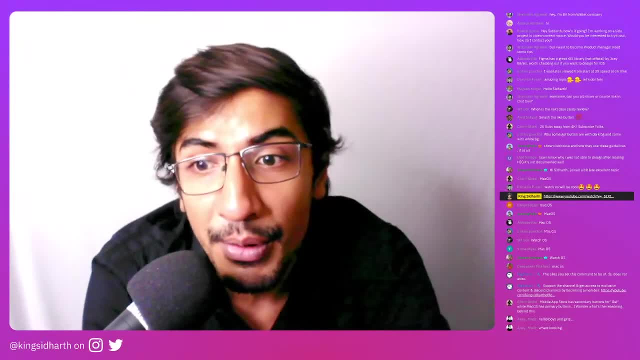 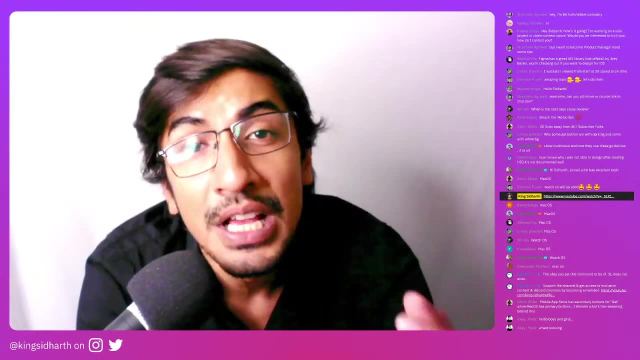 With that we have covered app how to read how to go about, how to survive in Apple's world of design systems, and how they think about design, how they encourage design. They lead by examples. look at who they are giving award to each year. 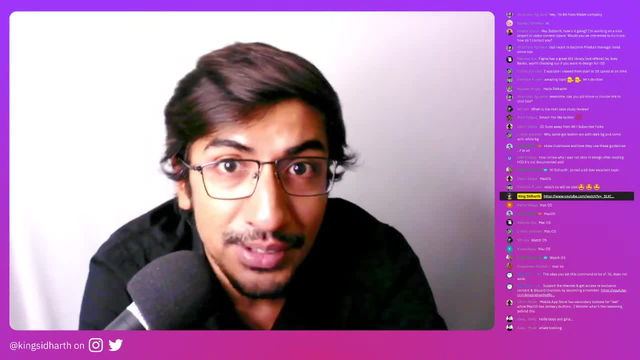 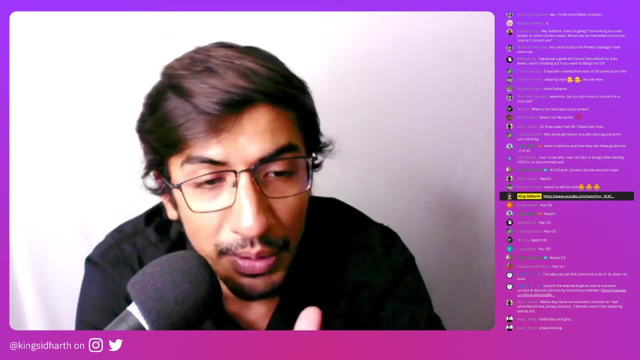 That's why who Apple hands out design awards to is critically important, because that's how they recognize: Hey, this is the kind of design which we encourage from Apple's side and we think is the best, And that's another way to learn. So that is why Apple events are so important. It's all. 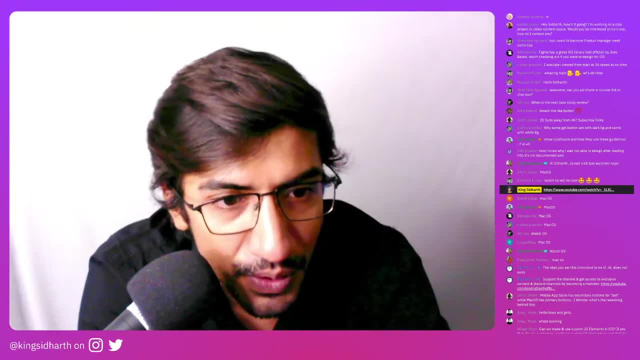 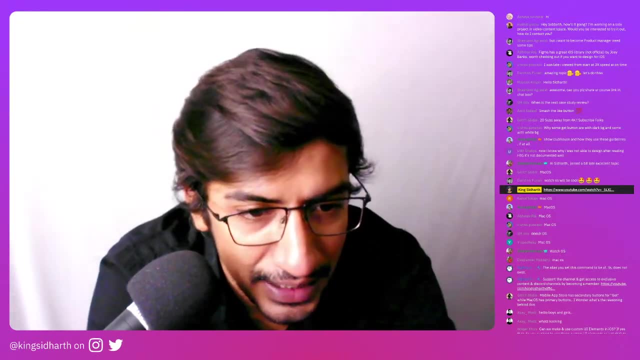 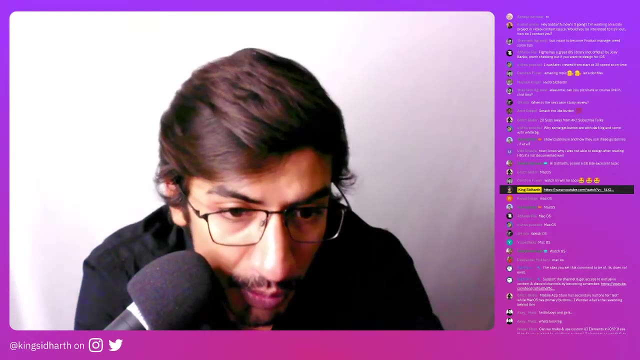 community driven, example driven. All right, All right, All right, We have covered that, All right. Akshay is here. Hello Akshay, hit that like button. if you haven't, Can we make and use custom UI elements in iOS? Yes, Yes, That is the intent. You are supposed to make custom or iOS elements. 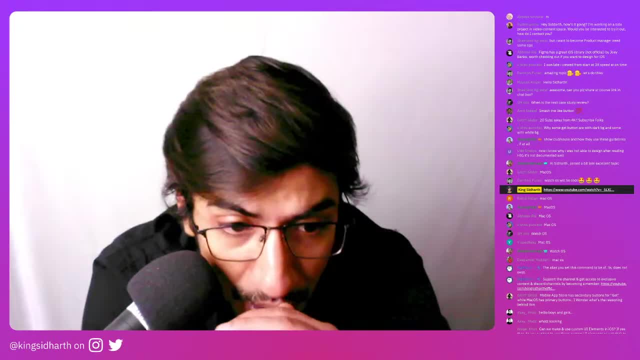 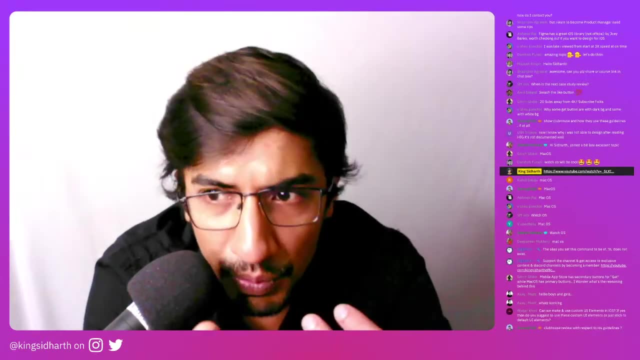 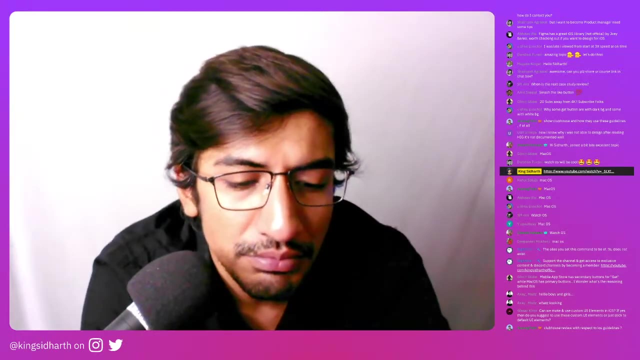 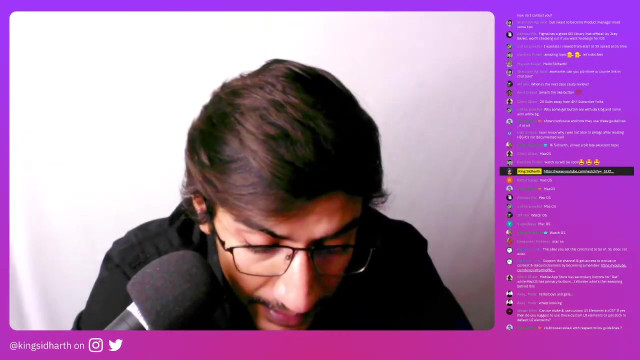 unless it already exists. If, then, do you suggest to use these custom UI elements or just stick to- I mean, you can and whenever there's a good reason, you should- Clubhouse review with respect to iOS guidelines, Think about it. I mean some parts confined to it very well, Some parts I don't understand, like the: 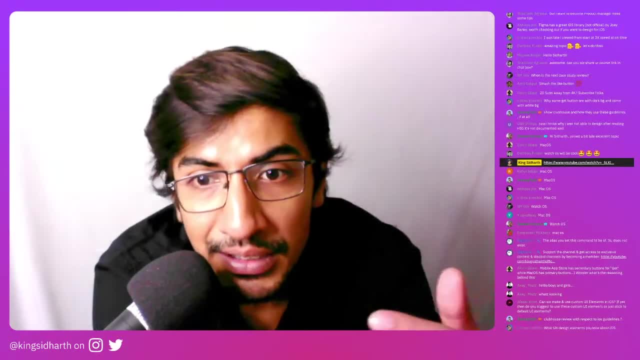 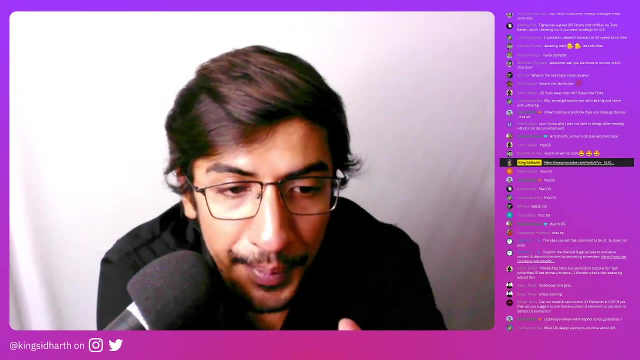 I think the biggest thing is for me the their use of tab bar is. you can say the tab bar is non-compliant, but I think that's a great reason to go away from clubhouse UI. So yeah, maybe I can open clubhouse and show some of you, as long as it doesn't join me into some random room. 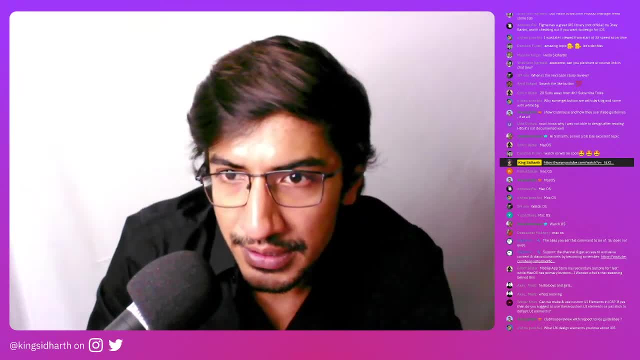 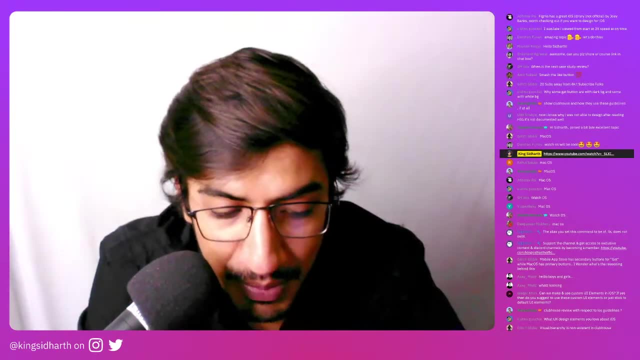 Yeah, So let me show you What I mean. So this is clubhouse, right? I have 10 invites, by the way, Those those of you wanted, and these are the rooms. So this is a you can say a modification of list view. 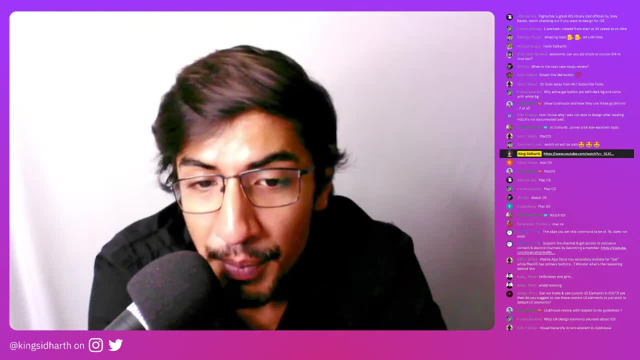 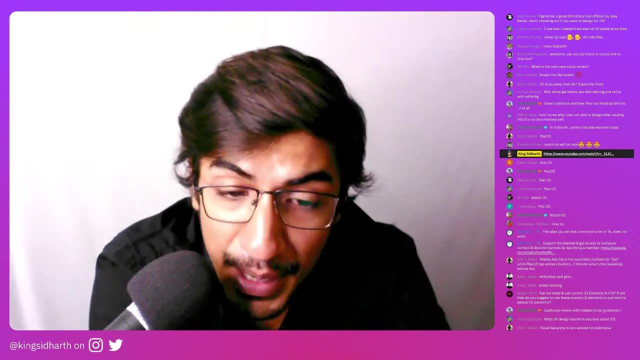 and the tab bar is very non-standard. This is not how we see iOS tabs bar, but I think it's a good modification and their actual tab bar, If you think about it, has moved on top because search, this thing- which for typically tab items, have moved on top. But I 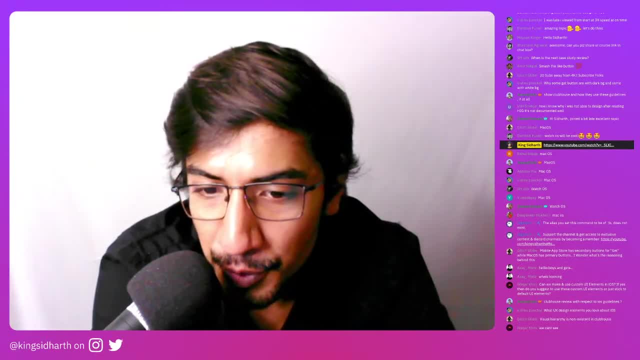 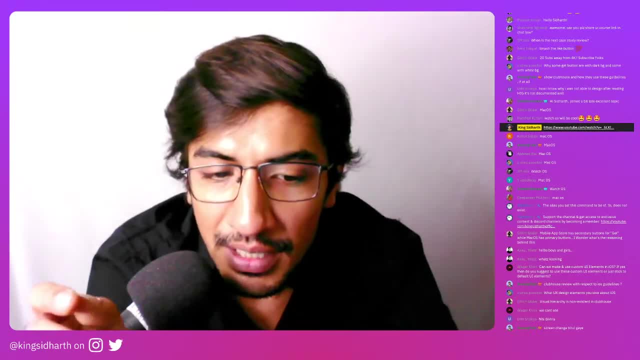 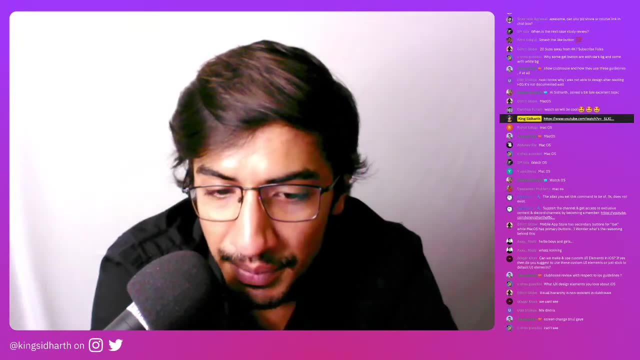 So it really does work for me, Like I don't think they are. they've not broken rules where they were not required. They have only broken rules where they've made it better. Of course, you could argue about many, many things, about how they've done multiple things. 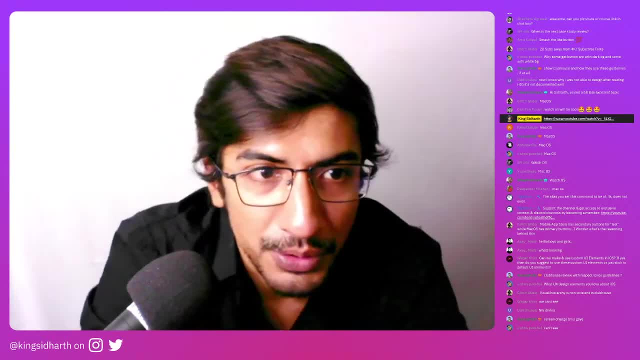 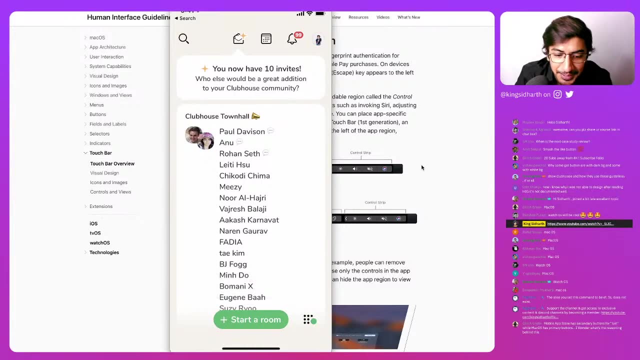 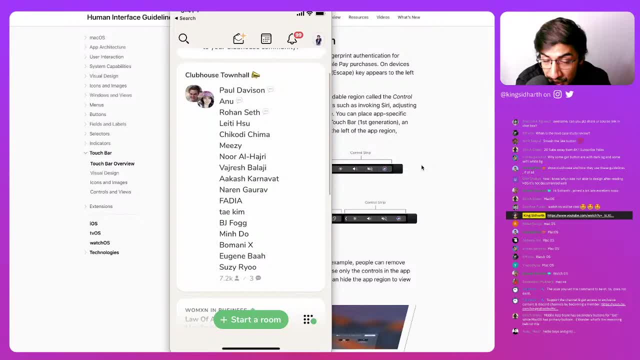 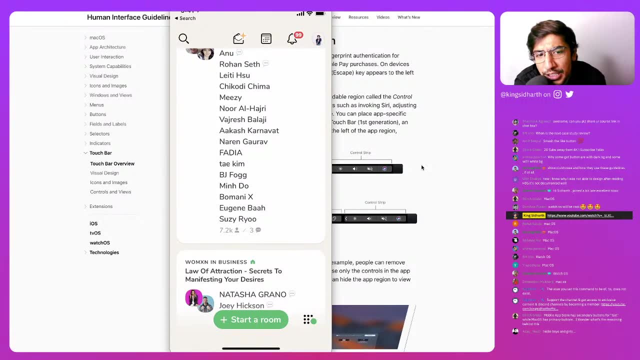 there's a list view which is modified. it's not typical table view. this is not how we see tables and the tab bar is also not standard. right there's a gradient happening and like every item which was on top, like notification, calendar, uh, invites and search, which are typical tab, and your account. 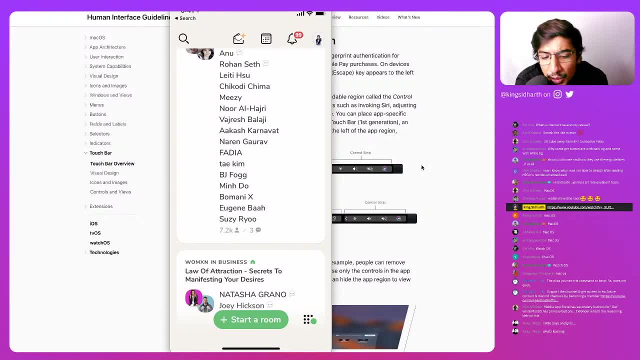 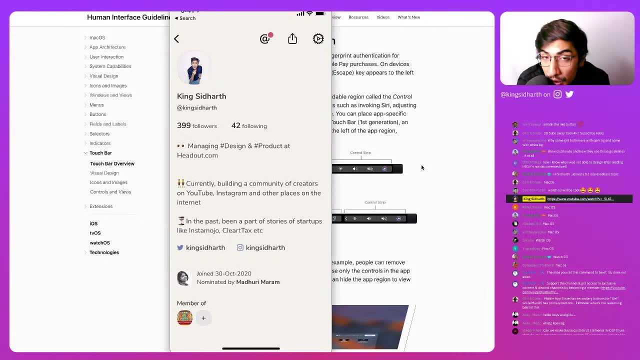 which are tab bar items are on top, but they know starter room and this thing will be more often used and they have. all the decisions they have taken are i i feel are good. all the rules. they are broken are from a reason and they're completely justifiable. by the way, i have 10 invites send me. 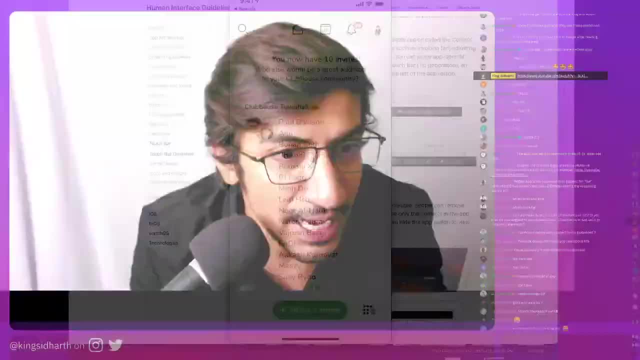 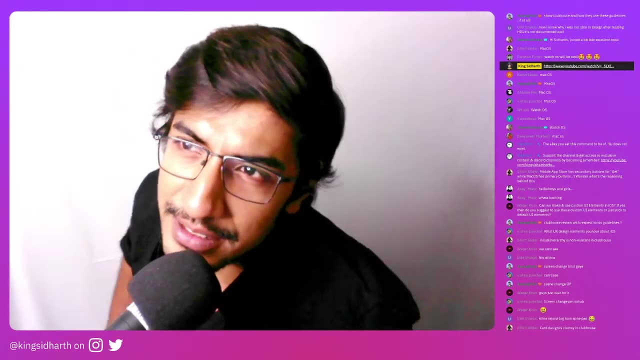 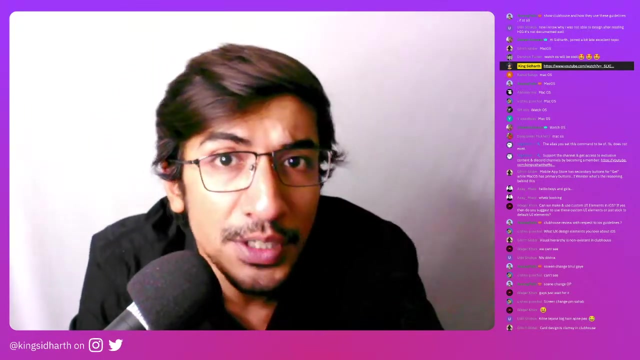 a dm if you want any of those invites. and with that we come to the end of today's live stream. if you learn something new, hit that like button and uh tell us. give me a suggestion on what should we uh be streaming about next. i'm planning just sharing with you. i'm gonna try and convince my 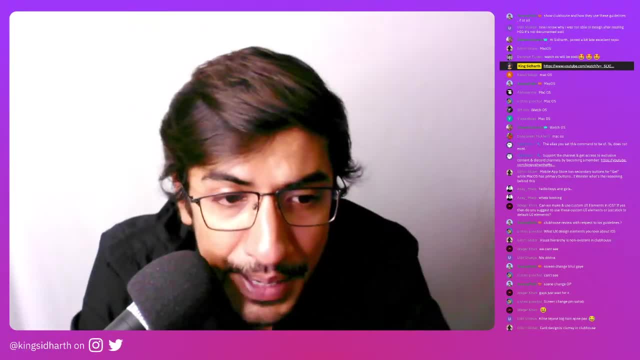 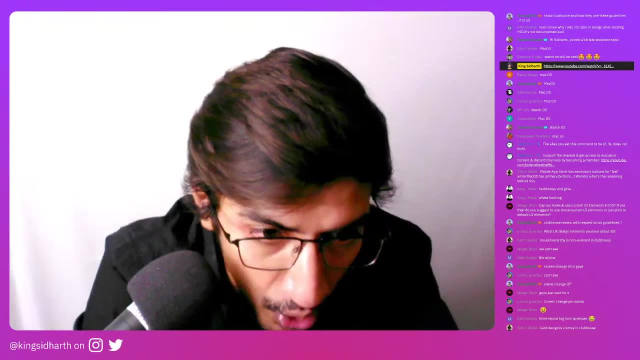 team who has been doing a lot of user research and user testing lately, to come and talk about user testing and specifically, specifically supervised task-based testing, something we employ a lot. that is why, um, let me know if you're interested in that. i can set that up next week. i can also do it in english. 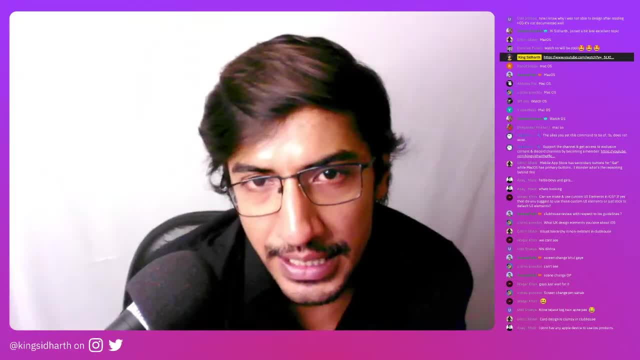 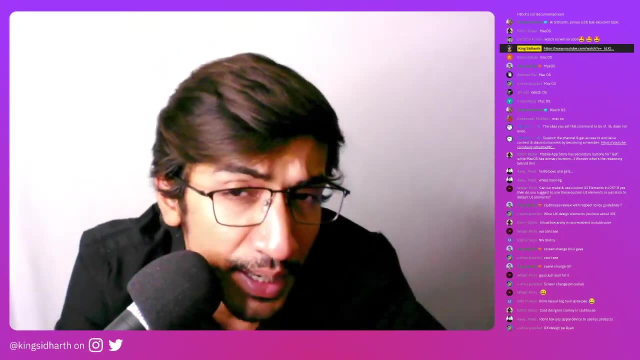 as well as hindi, or both, like once we do english and then we do hindi with a different team member, so we can do that as well. let me know what you're interested in. car design is clumsy in clubhouse. a lot of design is clumsy in clubhouse because they're fast growing, that you will see a lot. 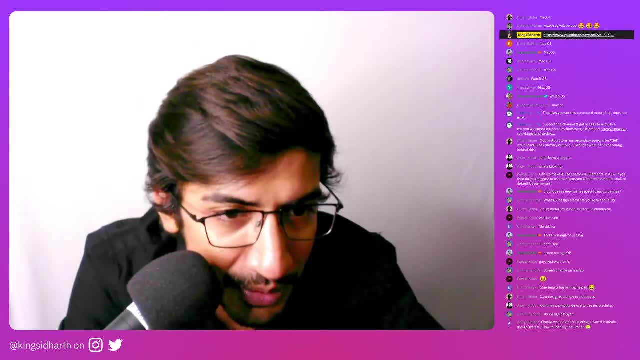 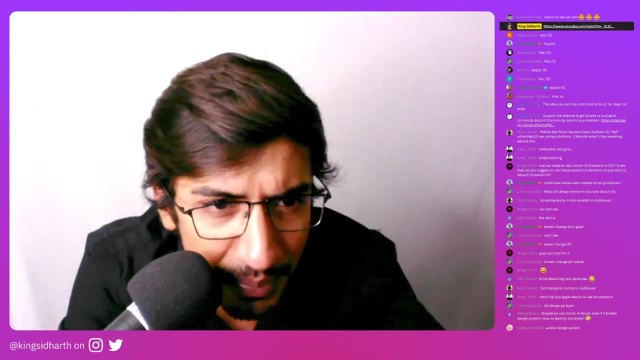 of things like that. they use five different styles of icons, so a lot of things are clumsy, i think visual hierarchy is there a little bit, not very great, but yeah, uh, all right, i don't have any apple device to use ios products one day, akshay. 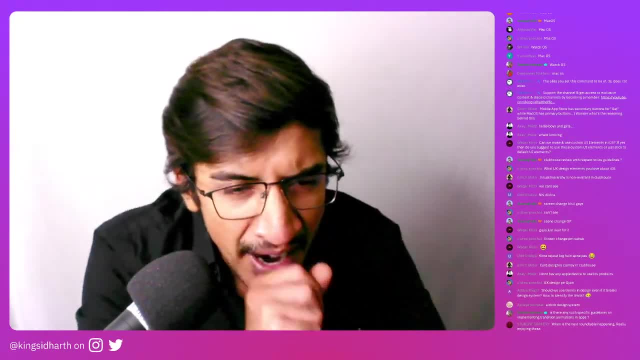 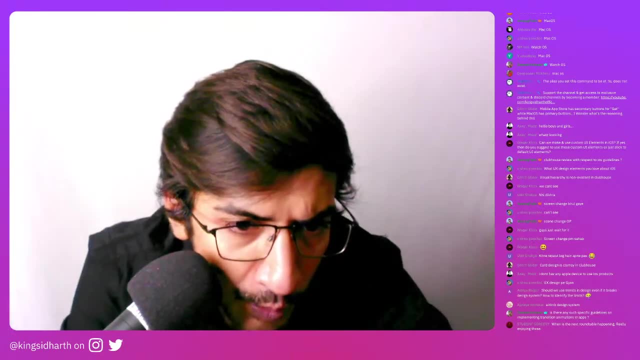 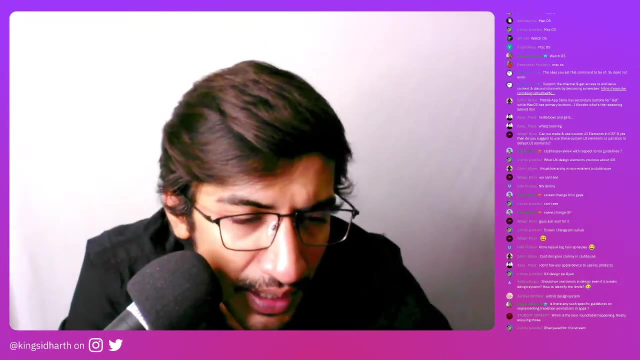 ux design. begun, gyan vishnu. it needs to be some specific um topic right, should we use trends in design even if it breaks design system? how to identify the limits? uh, unless there's a great reason to use a trend, um, i don't think i mean, keep them the social media post. no, that's where you can break systems. if 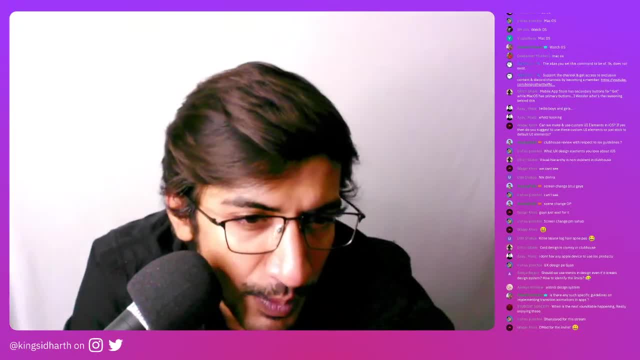 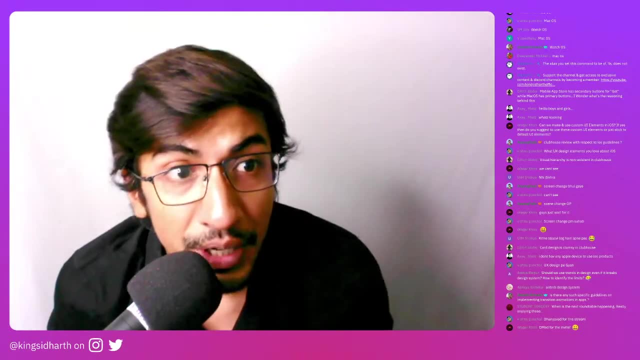 you want, don't break it in ui. airbnb design system. oh, you, you, we can. that's an interesting opinion. let me know what the folks think about it. we can continue this design system series and go through other companies design systems if you want. that is how we can continue the series. 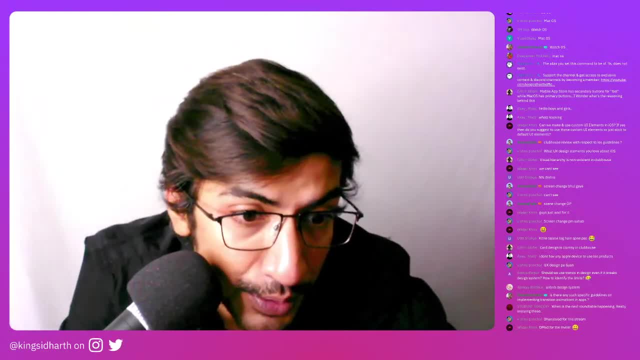 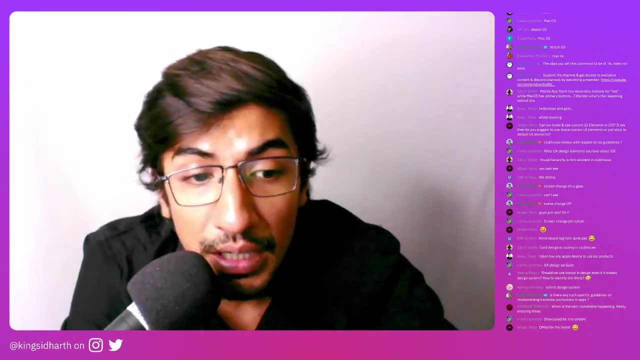 like. airbnb is one, zomato is another. we can go through these people's design systems if you want. let me know if that is something people will be interested in and if yes, which companies, uh, invite a design system. what am i saying in white? which company's design system? 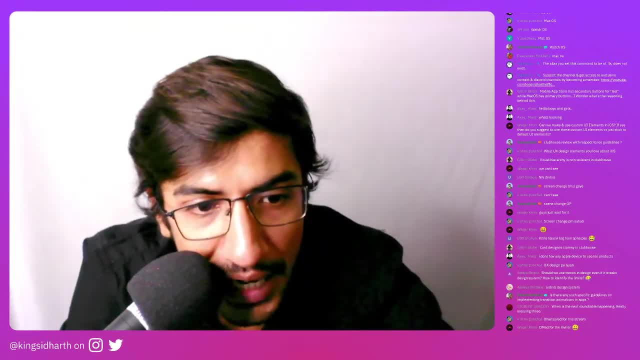 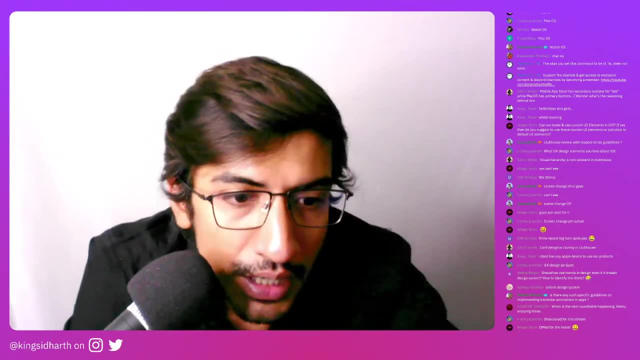 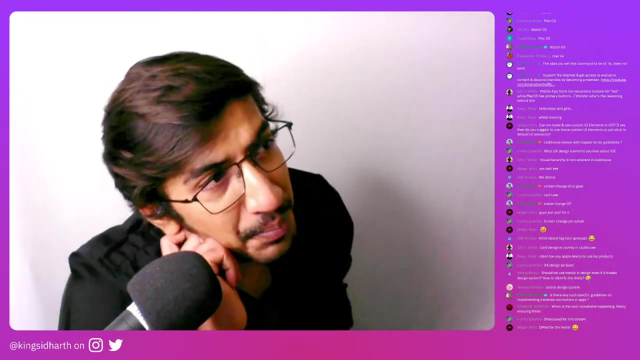 will you be interested in? let me know in the comments as well in live chat. is there any such specific guidelines on implementing transition animation in apps? not really the niche, not really students, are there? just example: student sorcery. when is the next round table happening? really enjoying, enjoy those food sorcery? i have not been able to plan. those require a lot of planning and 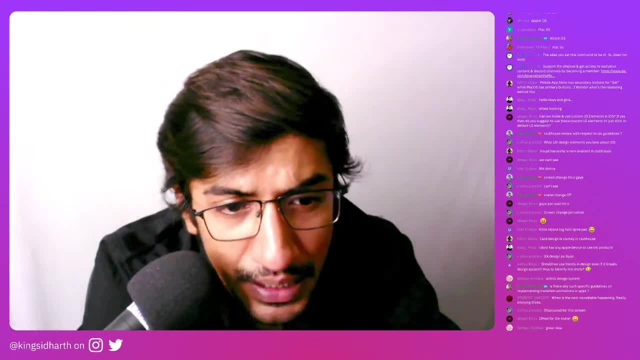 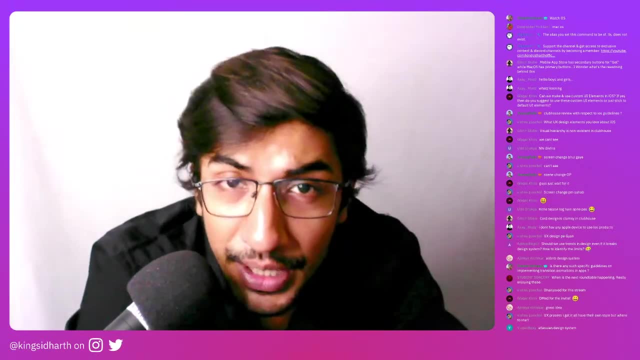 you know, preparing, for which i have not been getting time, but soon i really want to do those. i miss those as well. i really enjoy hosting uh round tables as well. i really want to get those back. so thank you for reminding me of those i this serves as a good reminder and inspiration for me to go back and try and 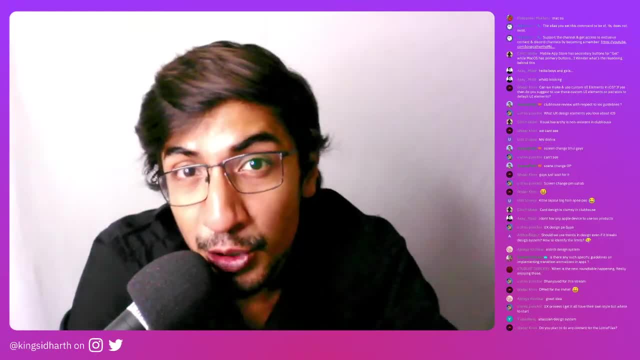 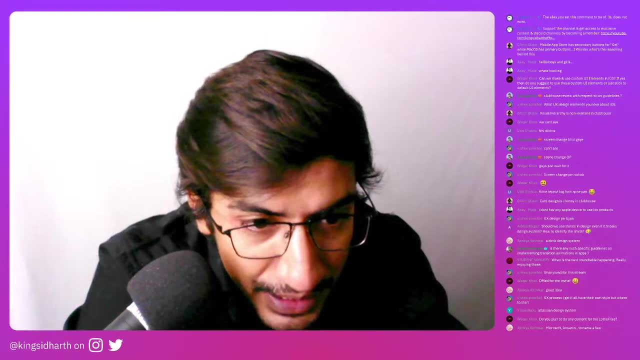 pursue that idea. so if any of you enjoy, do. if any of you enjoyed something that i did and i'm not doing it anymore, let me know in the comments. you never know, that will probably become a kickstarter for me to do it. uh, ajankya says: great idea, this, that's your idea. ux process: i get it all i have. 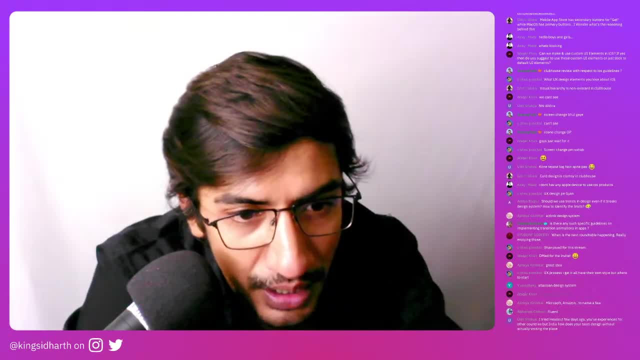 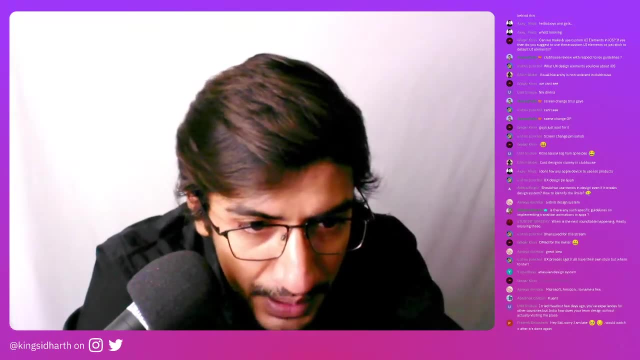 their own style, but where to start? all right, that's a very vague question. vishnu, atlassian design system, that's a good idea. atlassian, microsoft, amazon, to name a few. fluent, we don't see a single company emerging. all right, so i will, i will. um, i tried, tried head out a few days ago. you have experience for other countries, but india. how? 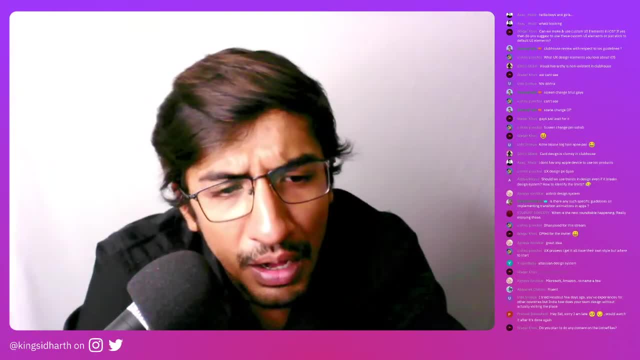 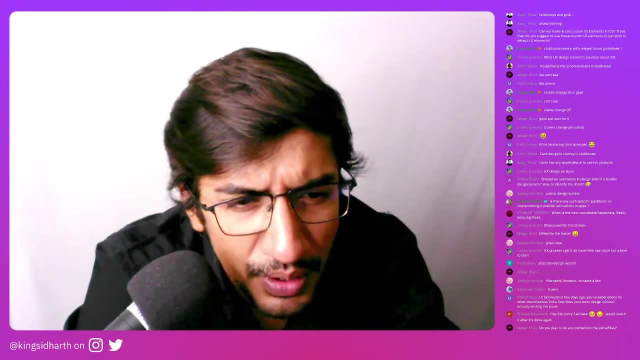 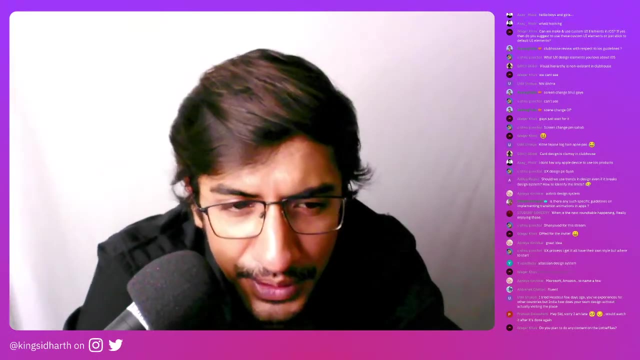 does your team design without actually visiting those places? um, um, that's an interesting question of that. i mean we know what goes on because there's ample of evidence, stories, direct connection, etc. etc. we know what's happening on the ground, so i mean we don't need to visit to. 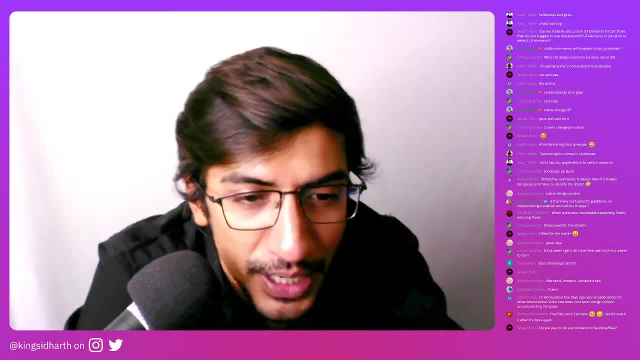 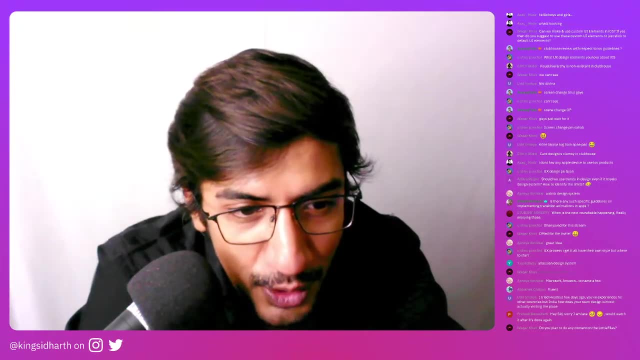 design individually. it's, it's, it's. it's complicated, it's not? i won't be able to answer the entirety of it in one stream, but yeah, we have our information. uh, hey, sorry. he said sorry i'm late, would watch it after it's done again. no problem, prateek, watch it back and hit that like button. do you plan to do? 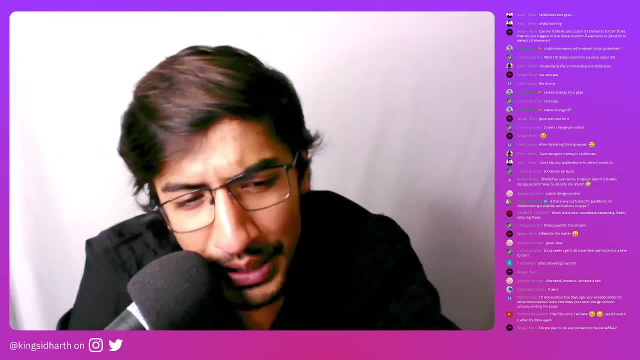 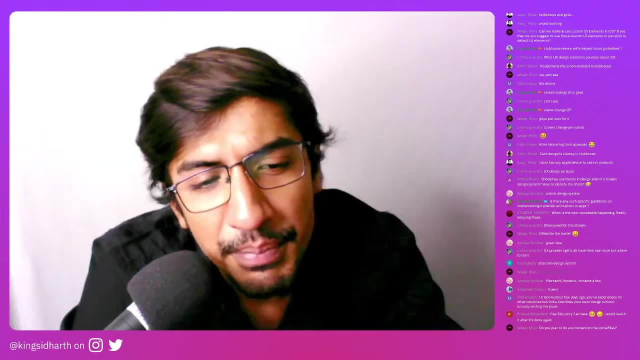 any content on lottie files. no, i may not be the right person to do that work. uh, uh, because um, a walker or walker- i don't know how to say your name, but i don't know if it's that's. but yeah, i'm not the right. 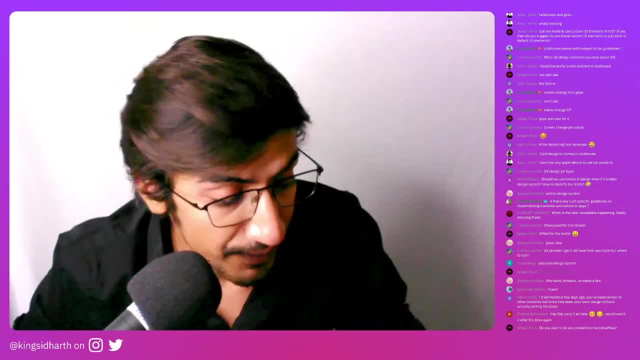 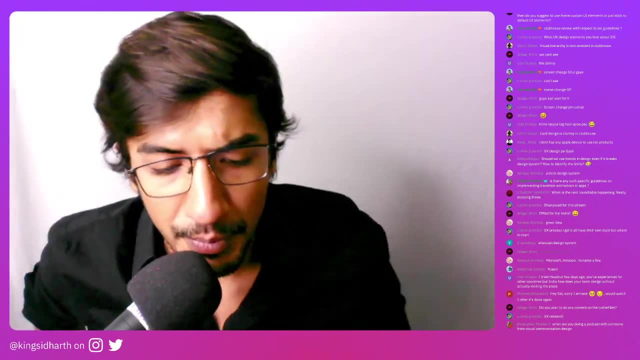 person to do lottie files, because i don't handle a lot of motion design for my company and therefore don't, and i'm not the person who ends up using lottie at all. we don't use lottie at all right now, at head out, but if- and we do end up using it, uh, someday i will invite a designer who takes the 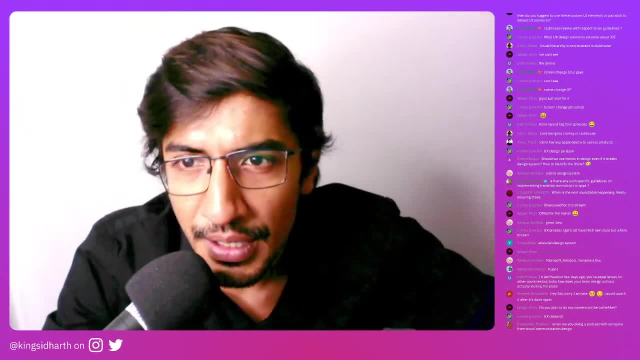 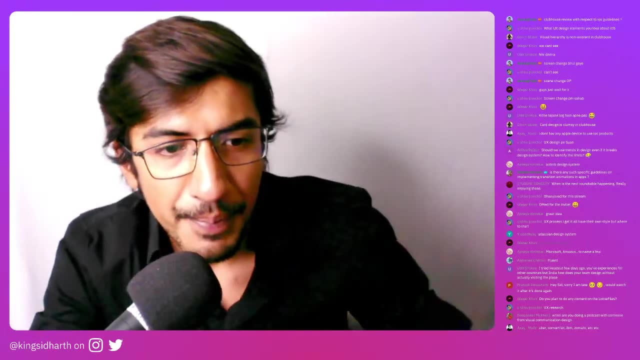 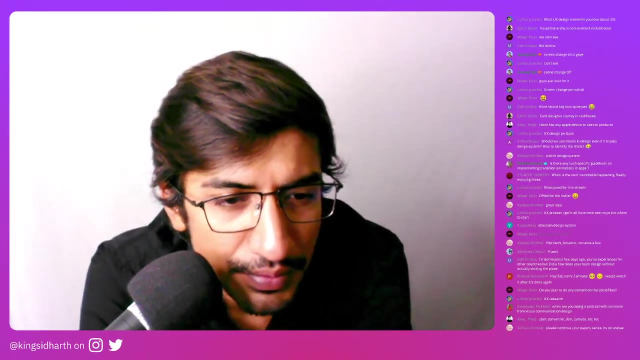 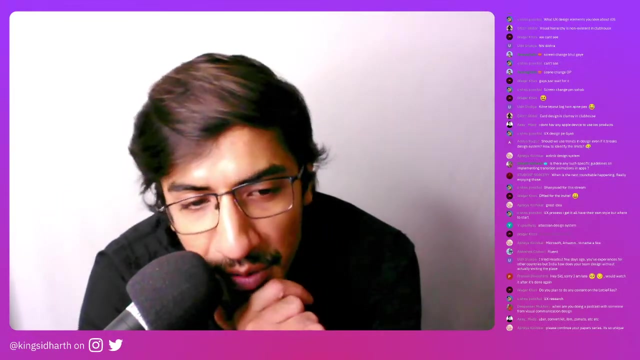 lead most likely will be our ux engineer. so yep. um, when are you doing a podcast with someone from visual communication design? um, we can, i have not planned anything. the punker: we can, we can, but i haven't. i said which plan immediately. but is there some specific thing you want to learn about visual communication design? 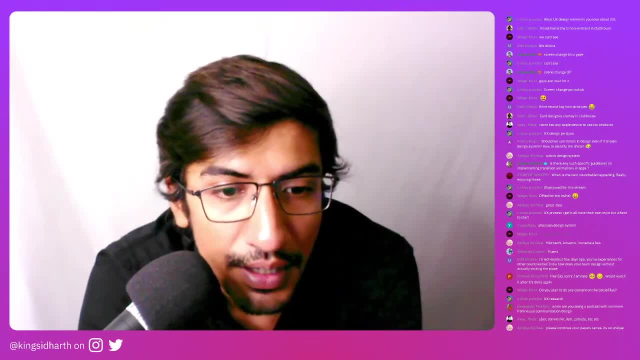 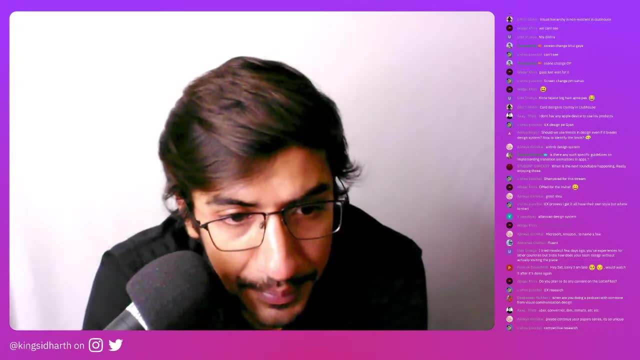 that you want, that. you want to know somebody's specific story, or is there a topic in mind that you're curious about? akshay says uber. uber is great, ibm is great, zomato- okay, uber and ibm and zomato are great ideas. 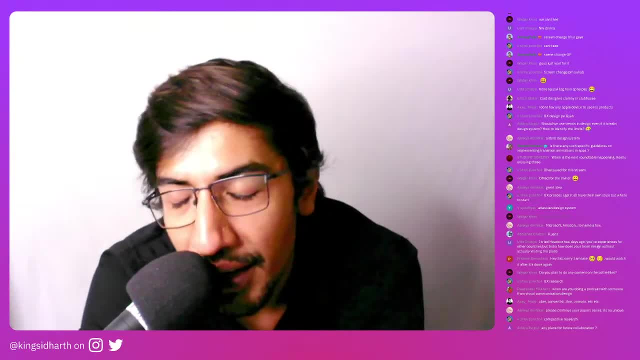 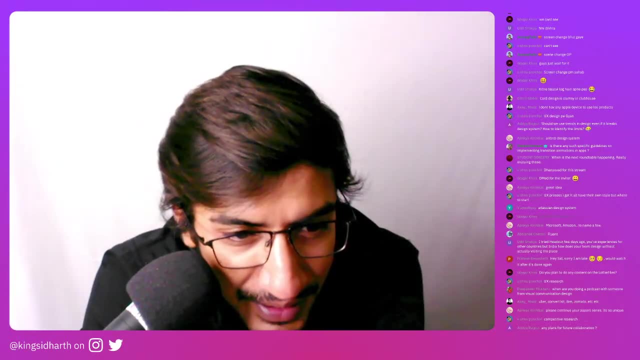 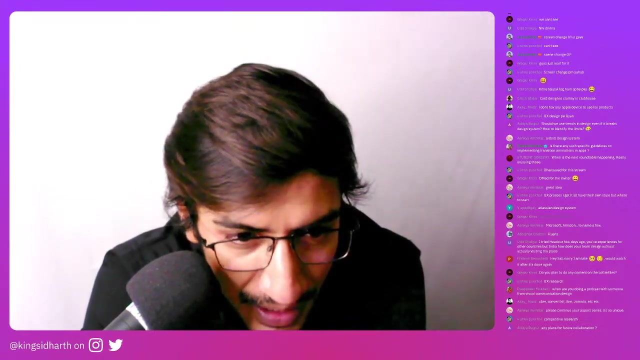 please continue your paper series. yeah, man, i have to continue the paper series. i just don't get time. i really want to continue that series. competitive research: what is competitive research? yeah, never heard of competitive research. competitor research: are you researching your competitors or are you talking about comparative analysis? competitor analysis, because competitive research. 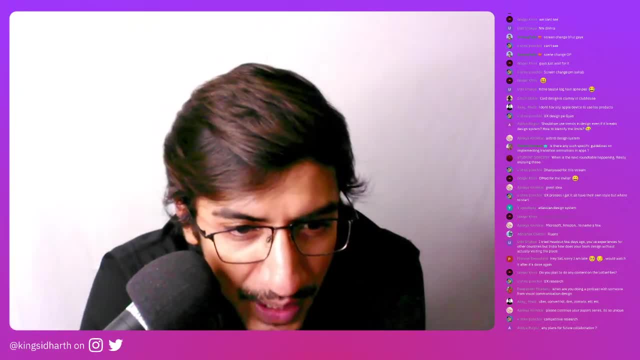 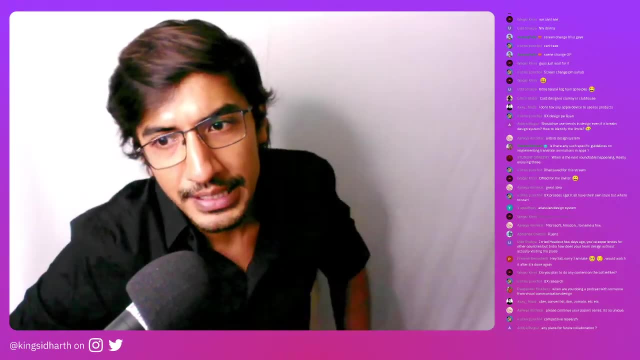 i don't know what that means. any plans of future collaboration? that's a very vague question, aditya. oh, do you mean like having guests? yes, i don't know what that means. but i don't know what that means. yes, yes, soon, soon, i have i've sent some invite to some guests. let's see how, when they respond. 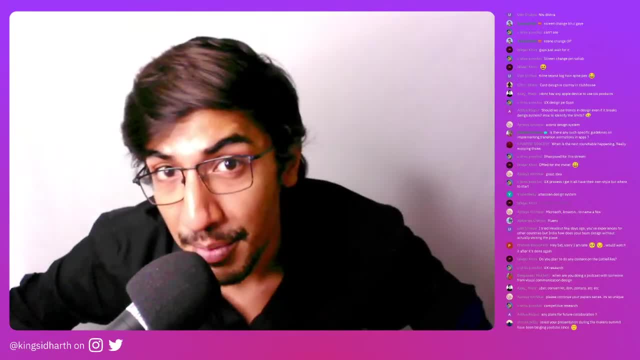 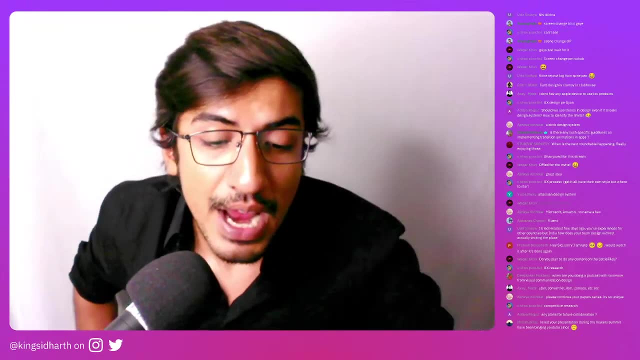 i'm planning to send out to more. thank you so much once again for joining in. hit that like button if you haven't already. if you're new here, make sure you're subscribed. we have a goal for hitting 5 000 subscribers by june, um, by start of june, by the end of may. basically, we want to hit, so we have. 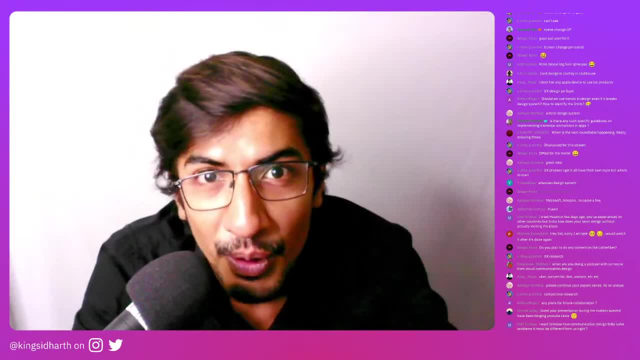 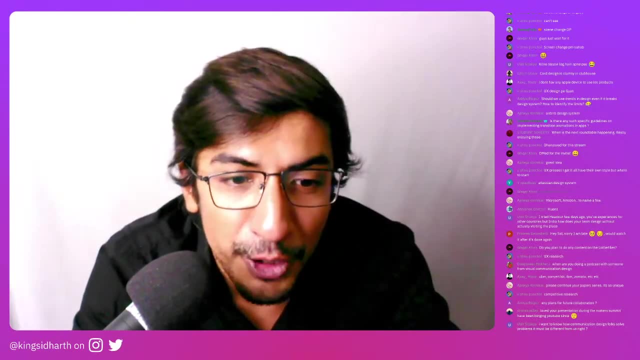 april, may, april and may. just two months left folks, hello thousand folks. we have to get more. share this channel, invite more people. we have to hit that target. all right, love your presentation during the maker summit. have been, uh, been doing youtube since. thank you so much, sharon welcome. 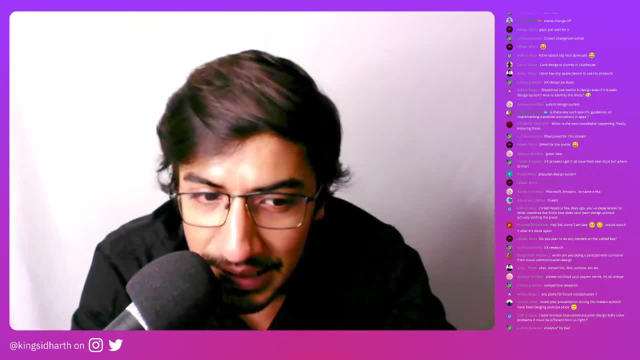 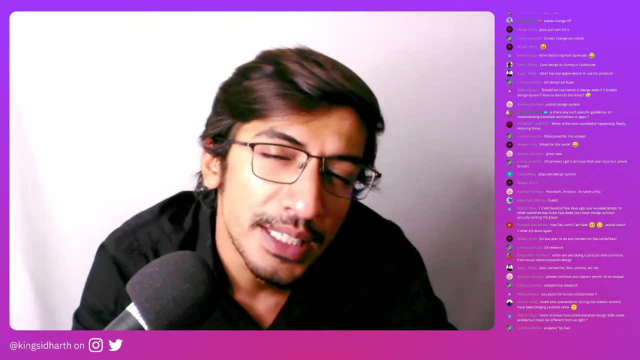 to the youtube channel and glad to see you live here. all this says i want to know how communication design folks solve problems. it must be different from us, right? ah, it is different from us. it is similar to us as well. both are equally lost. but i guess we can invite somebody from visual. 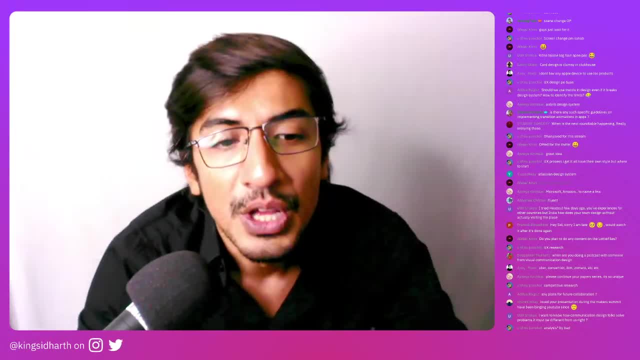 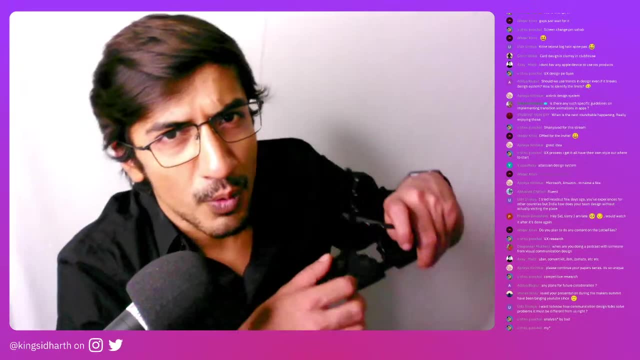 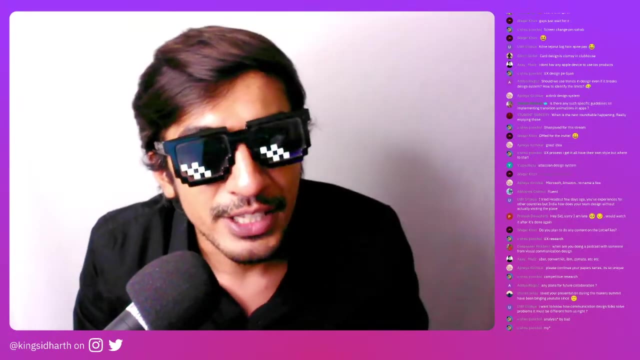 communication design and help us figure out what their process is like. all right, with that, i'll take your leave. once again, thank you for joining in on this weekend. check out the new episode where uh- where uh- new feature chachi is talking and complaining about tech dead chacha and engineer bhai resolve trying to resolve their age old conundrum. check that new. 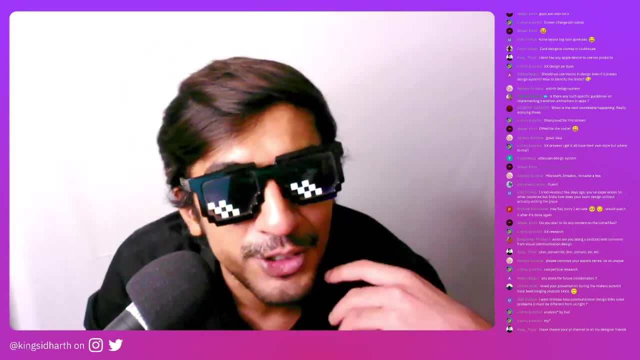 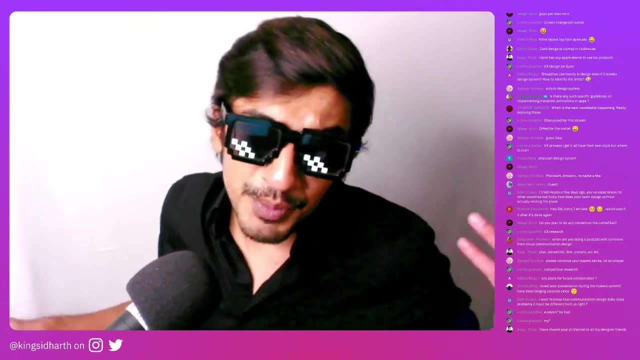 episode out on instagram. give that some love, give it some comment, share it on story. tag me, show some love and i'll make more episodes. intern kumar will make a return very soon. if you love intern kumar and if you've been missing, uh, dm me, etc. etc. and comment here. so 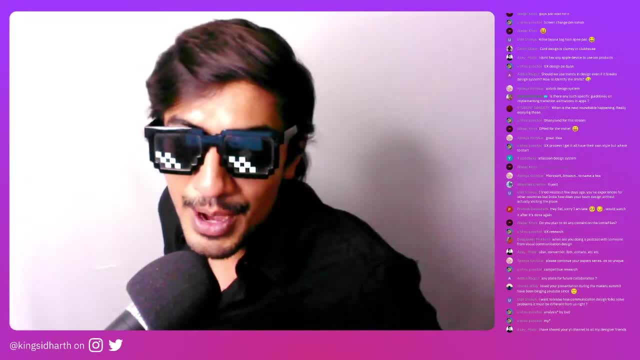 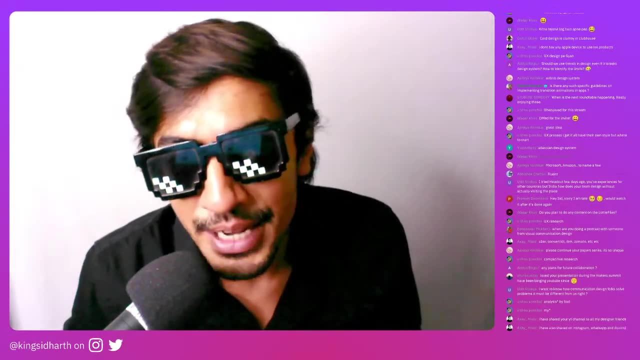 i know you've been missing, intern kumar, and i'll see you. very uh, i'll see you next weekend right here around the same time as we always do. till then, take care. good night. shabba, khair, shubh, ratri, sayonara, love you, marry me, etc. you.